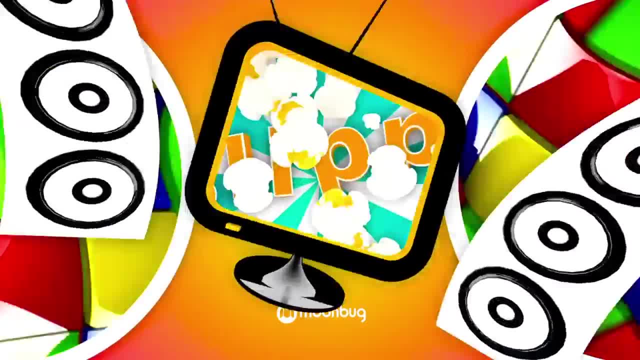 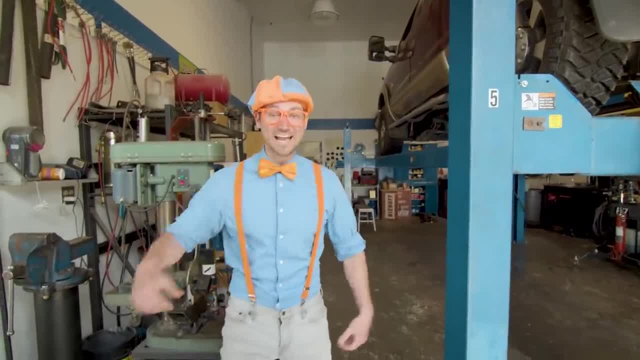 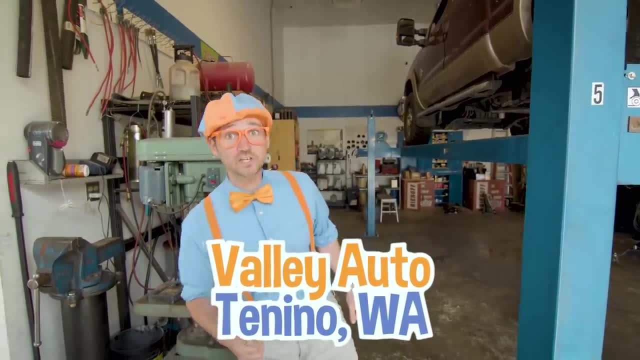 So much to learn about. It'll make you want to shout: Blippi, Whoa. Oh, hey, It's me, Blippi, And look at where I'm at. Yeah, I am at Valley Auto in Tenino, Washington. This is where they work on vehicles. Whoa, do you see that truck up there? 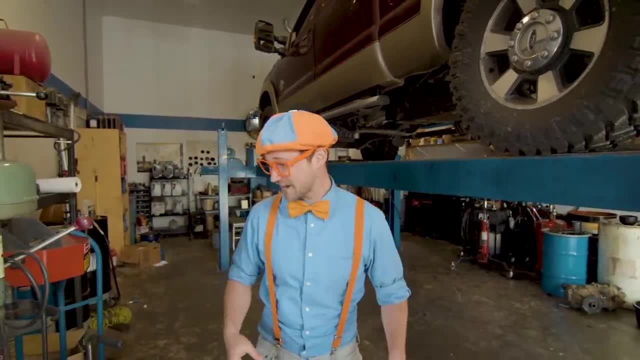 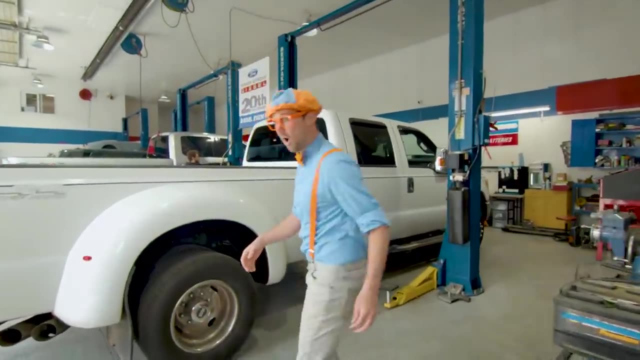 Whoa, It's so high up there. That's crazy. Whoa, so many cool machines in here. Come on, Whoa, Look at this big truck. Do you see how it's on the ground? Yeah, they're on the ground. 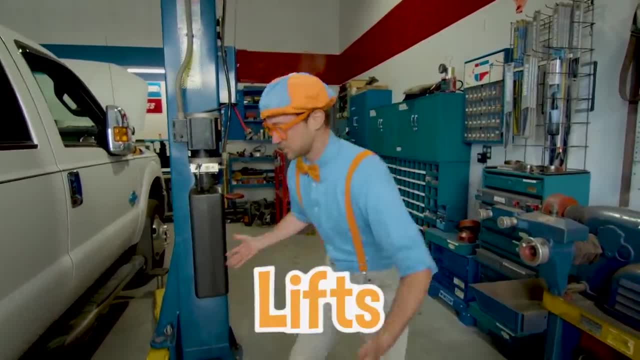 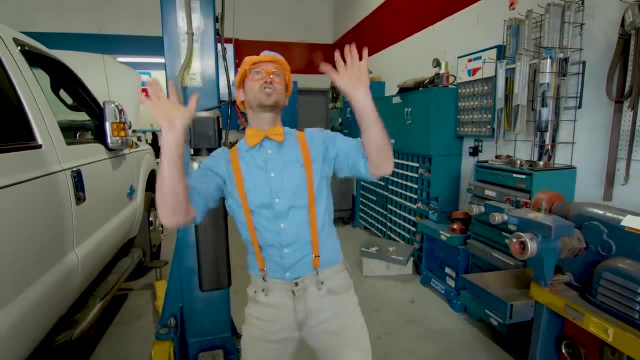 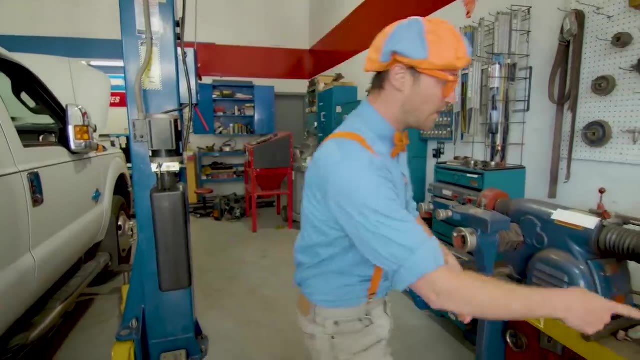 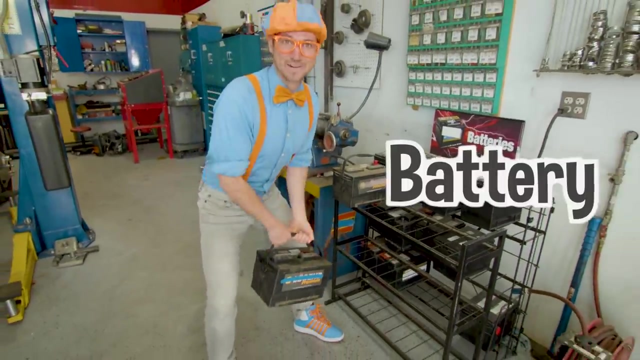 but then they use these big things called lifts to go underneath and lift it up to the sky, So then the mechanics can work underneath the truck and car, So then they don't have to bend down or be uncomfortable. That's pretty cool. Oh, look at this. Whoa, this is so heavy. Wow, this is a battery. Yeah, most vehicles have. 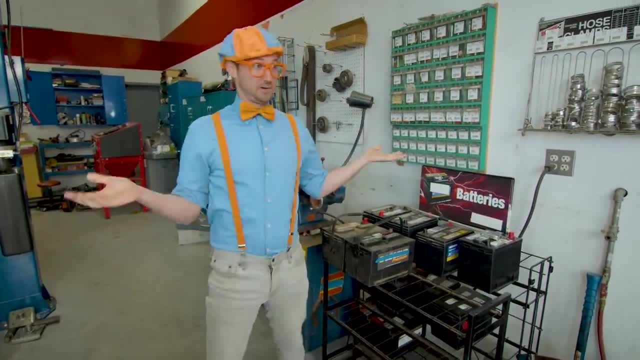 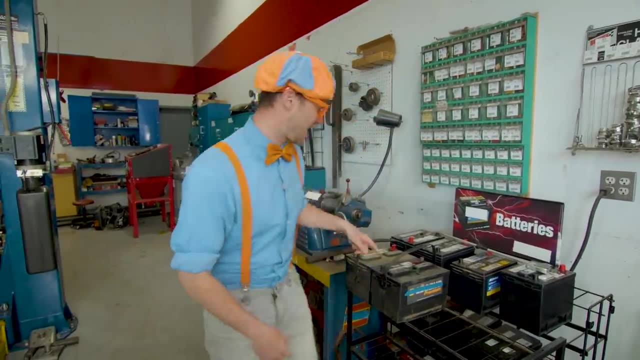 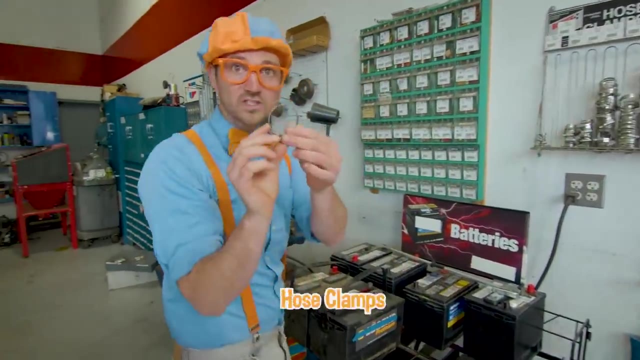 batteries. so then it helps them turn on, Yeah, and also turn on the radio And things like that. Yeah, batteries have electricity stored inside. Oh, look at that, Look at these. These are hose clamps. Whoa, there's a small one and here is a big one. 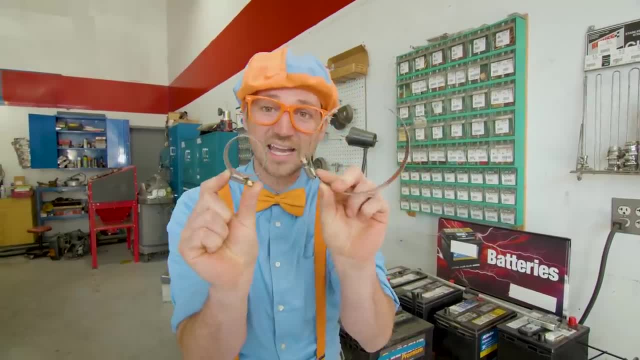 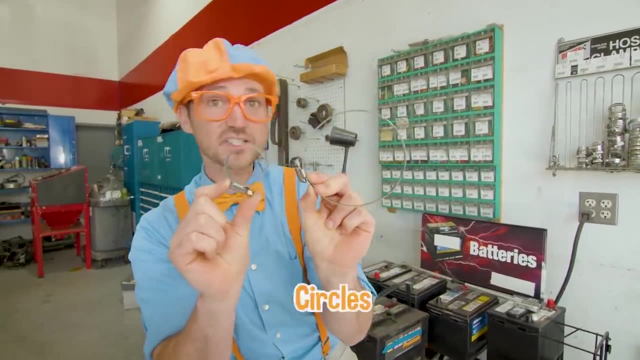 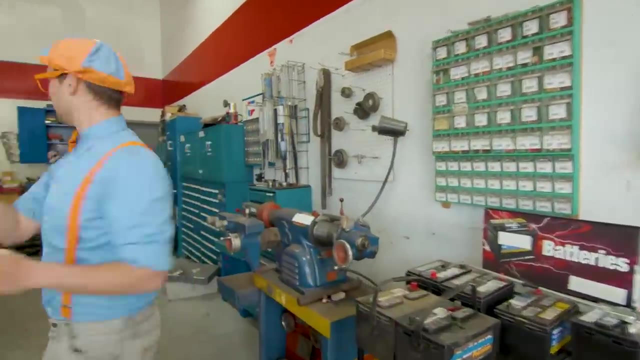 These are what goes around: hoses and clamps them nice and tight. Hey, what shape are these? Yeah, these are circles. Pretty cool, huh? All right, let's put those back. Let's keep exploring. Whoa, Look at all of this. 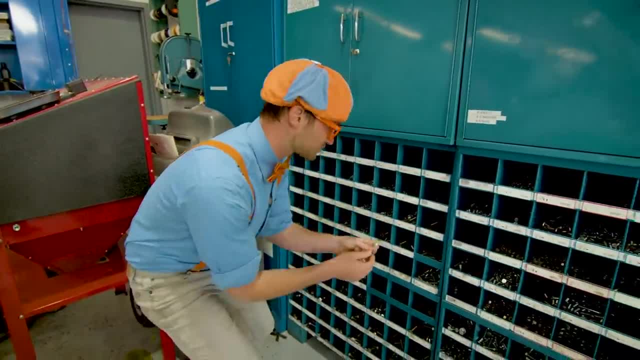 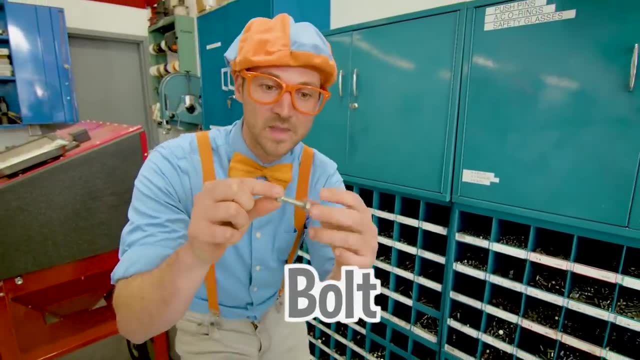 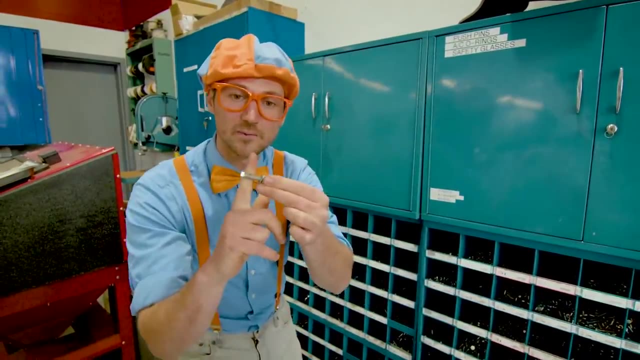 Look at all of these. Do you see these? Wow, This right here, yeah, is a nut washer and a bolt. This is what you use to tighten things. Yeah, nice, and close together Like, say, if there is a piece of metal right here. 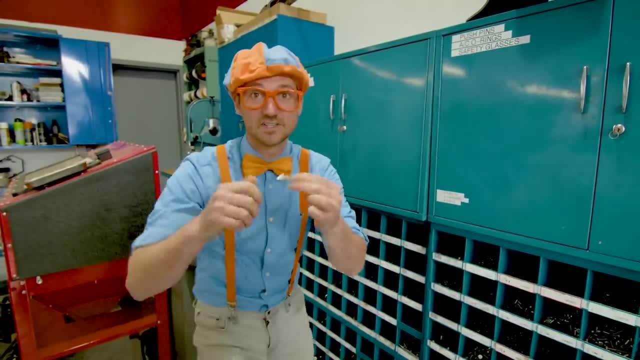 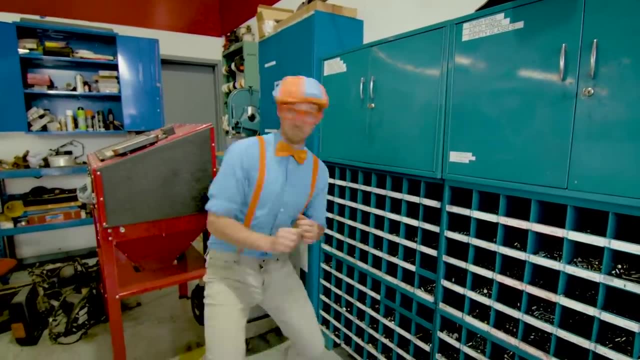 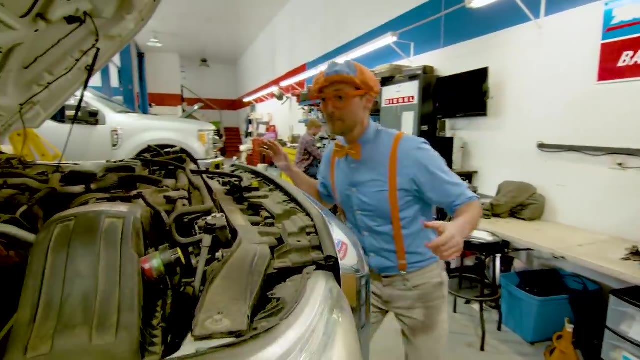 and another piece of metal, you could tighten it nice and tight, so then it doesn't slip and slide. All right, let's put that back. Uh, Okay, whoo, So cool. Whoa, This is a massive engine That looks so powerful. Wow. 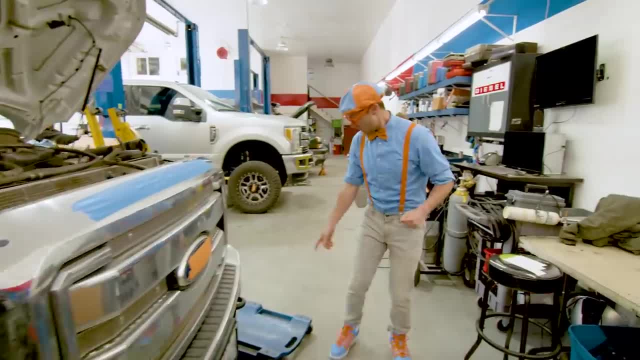 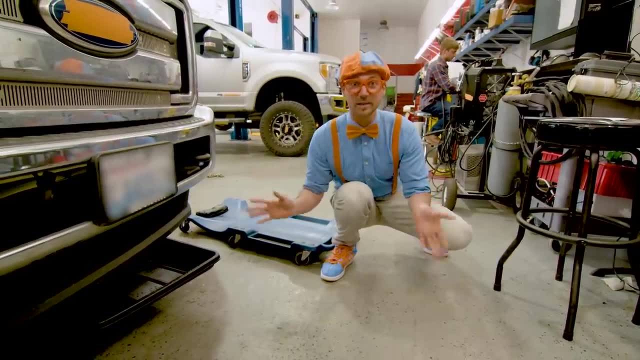 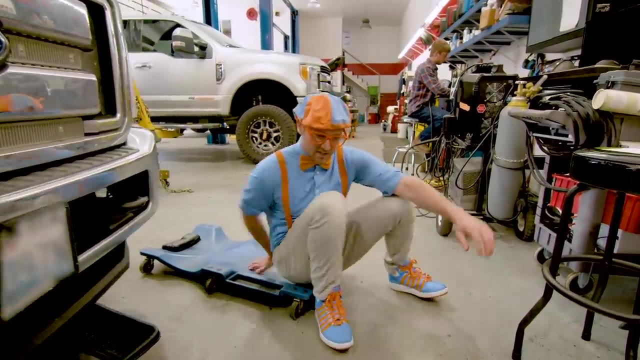 So cool. Well, hey, let's see. Oh, look at this. Remember earlier how I said that the lift lifts up the truck so the mechanic can stand up nice and tall. Well, sometimes you might not have a lift And you need to get really low on the ground and work on the vehicle from the ground. 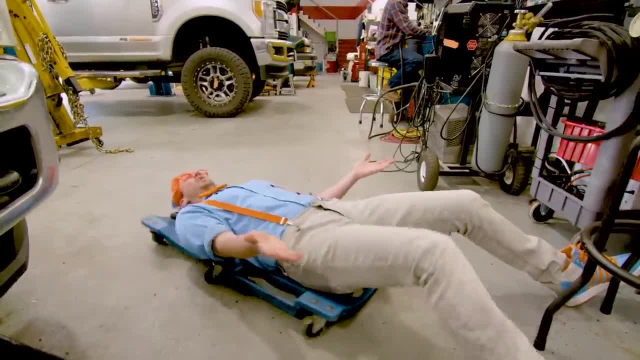 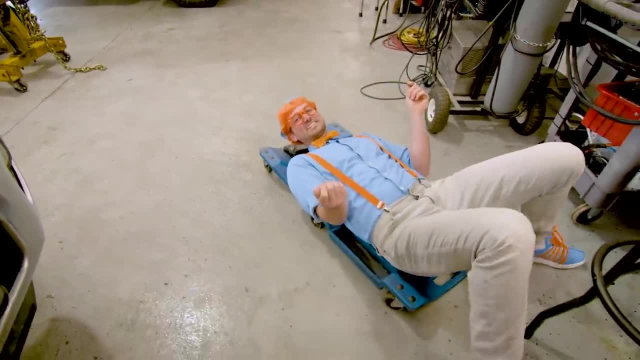 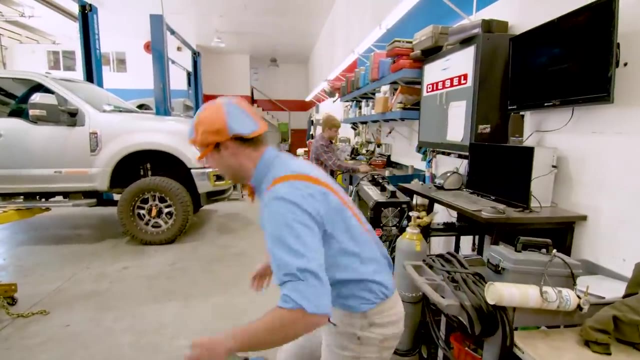 Whoa Hey, Whoa Whee. Look at me, go, I'm a mechanic. Whee, Yeah, you can slide because it has wheels. Okay, all right, enough playing around, Let's get to work. Oh, hey, It's someone else. Who are you? 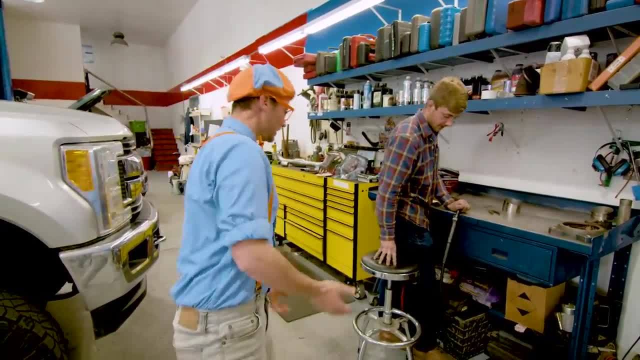 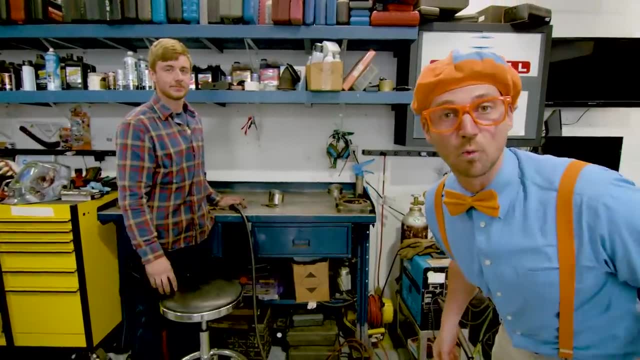 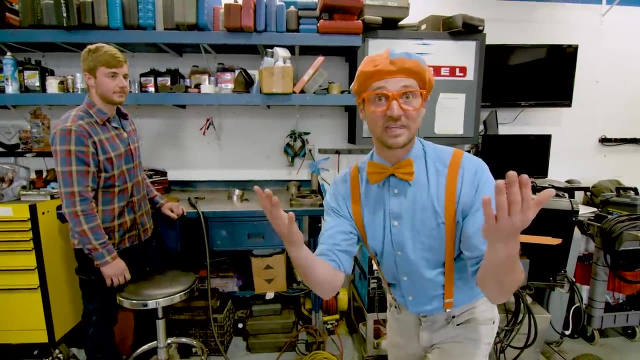 Colton. Oh nice to meet you, Colton. Well, what are you doing over there? Getting ready to weld? Oh, weld, That's really cool. Hey, do you know what welding is? Yeah, welding is where you take two pieces of metal and apply some electricity, heat, some gas, and it becomes so hot, they become connected. 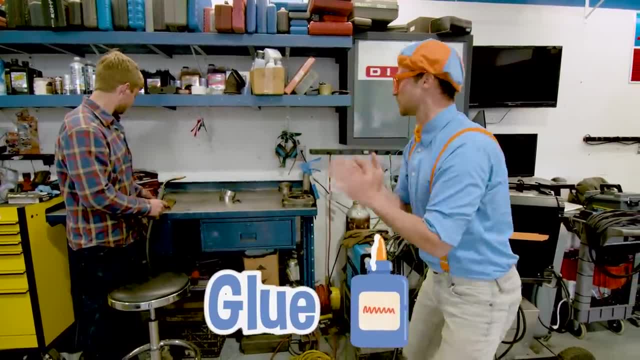 Yeah, it's kind of like that. It's kind of like glue, but for metal. Well, Colton, will you show us how to do it? Yep, I just need to lift up the truck. All right, let's check it out. 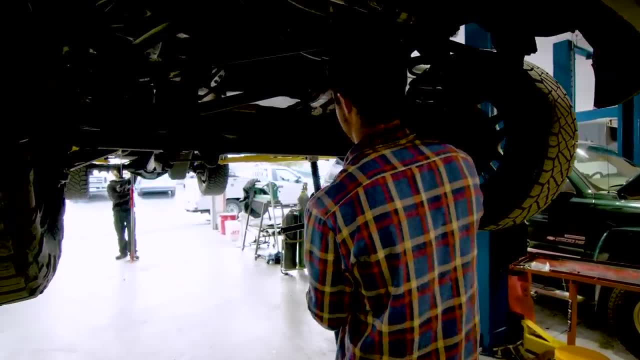 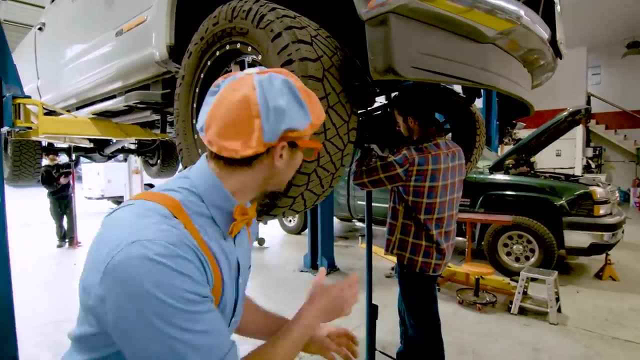 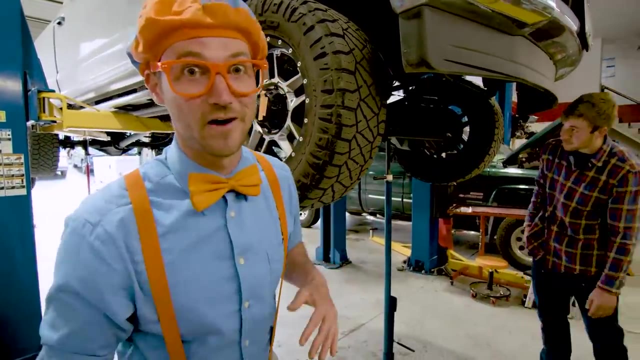 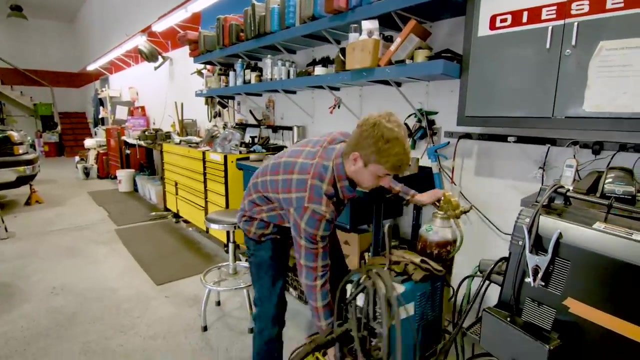 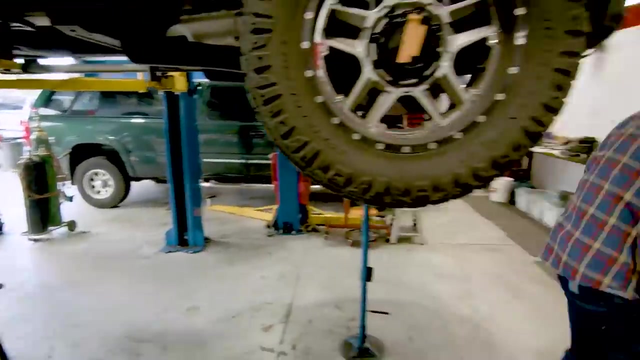 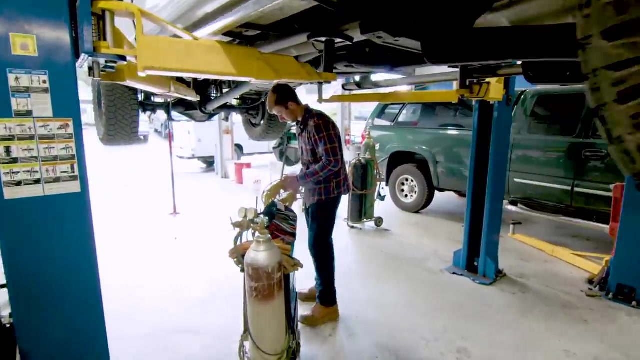 Wow, do you see what they're doing? Yeah, they're using those metal posts to go under the truck so then they can work underneath it safely, so it doesn't fall on them. Okay, let's watch them weld. Oh, looks like he has some safety gear. 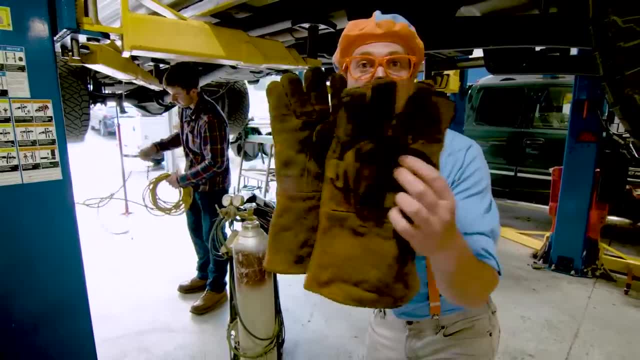 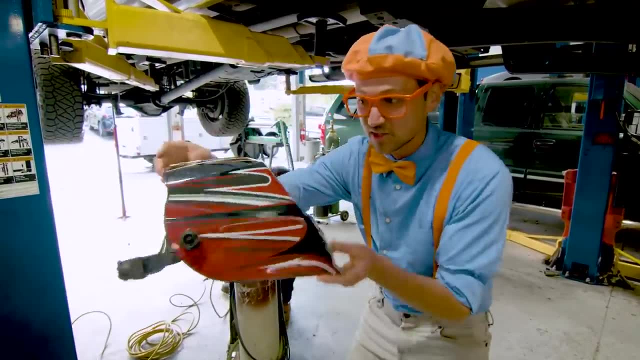 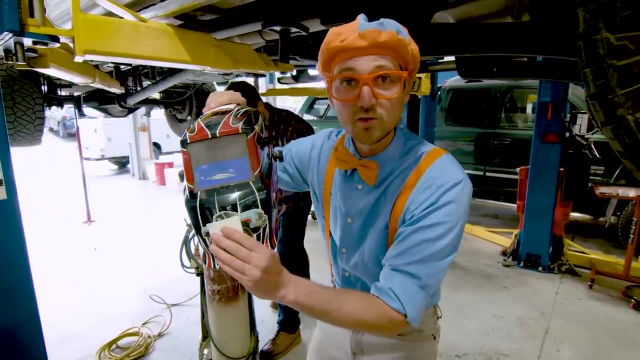 Check it out. See these? Yeah, these are his gloves. It keeps his hands protected while he's welding. And this looks like his helmet, Yeah, and it has this really dark shade right here. So then he can't see, He can't look at what he's doing because it's too bright to look at without this. 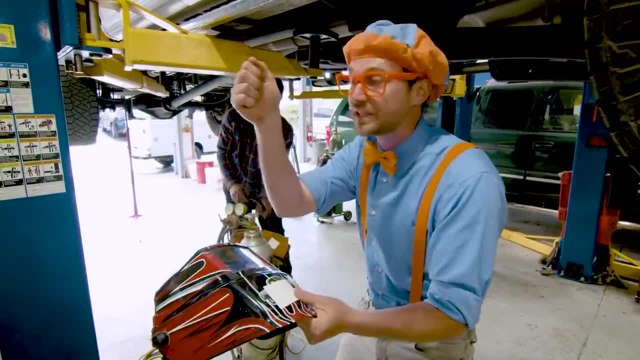 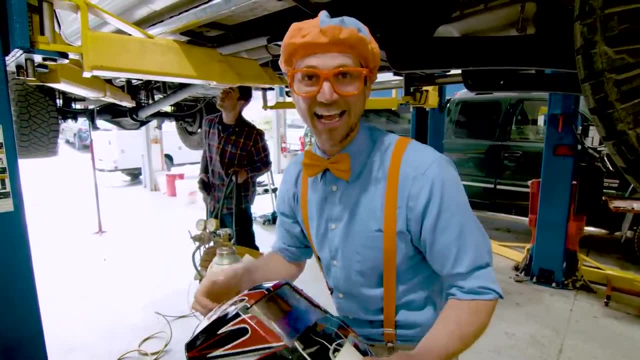 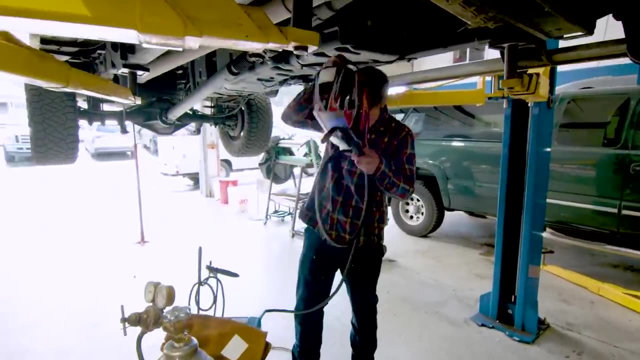 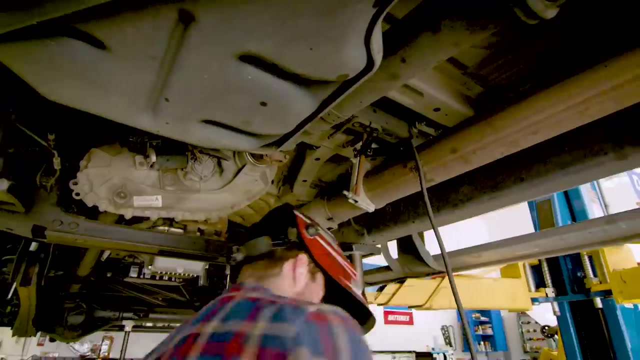 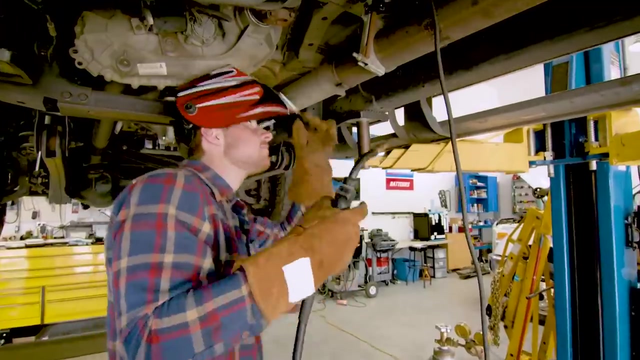 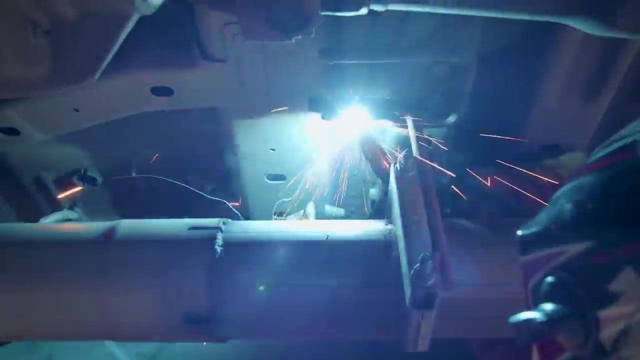 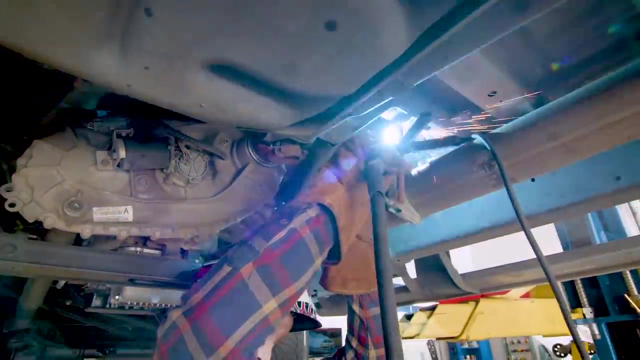 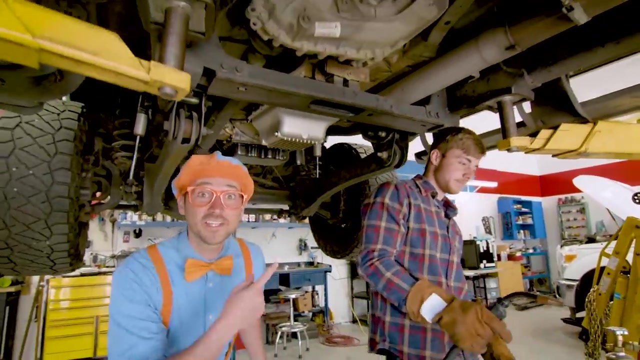 You definitely never want to look at what you're doing welding, unless you have this. So if you ever see someone welding, do not look at that light. okay, Okay, Oh, here you go. Ha ha, Whoa, Did you see that? 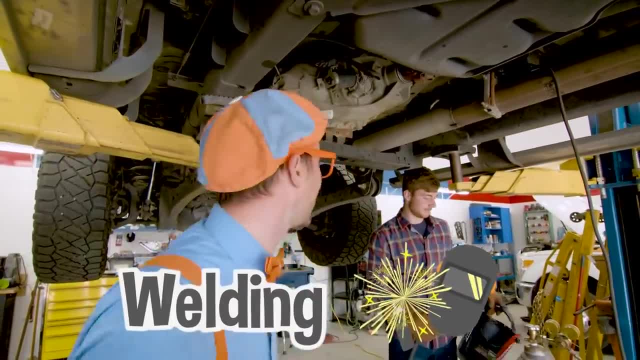 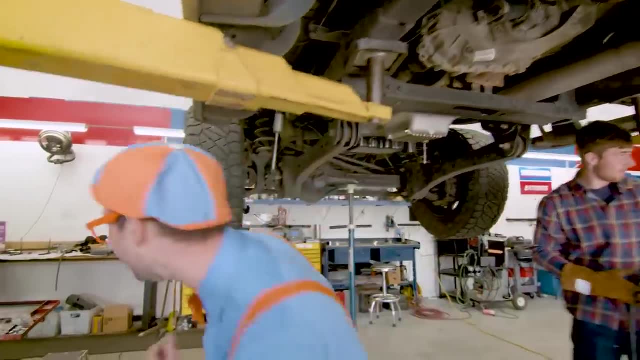 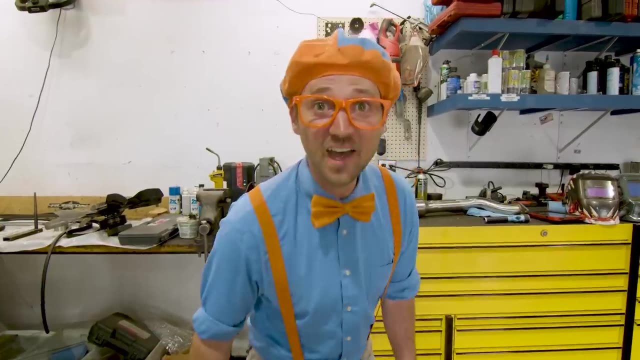 Wow, colton did such a great job welding. hey, colton, thank you so much for showing us how to weld. yep, no problem. yeah, all right, let's keep exploring. let's go. this has been so much fun. did you see? when he was welding it looked like fireworks. 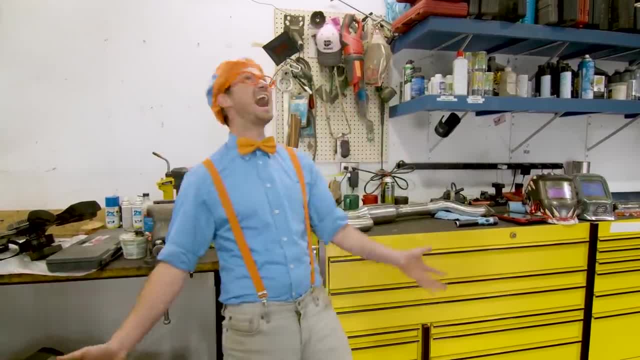 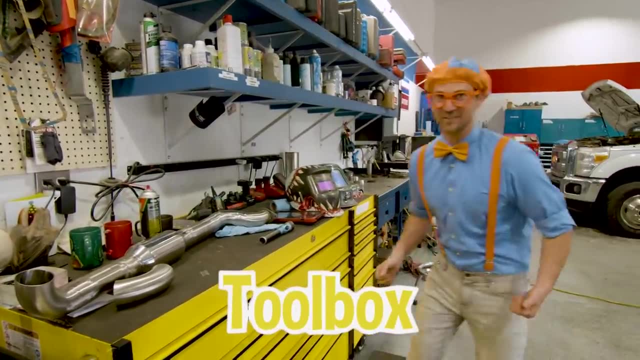 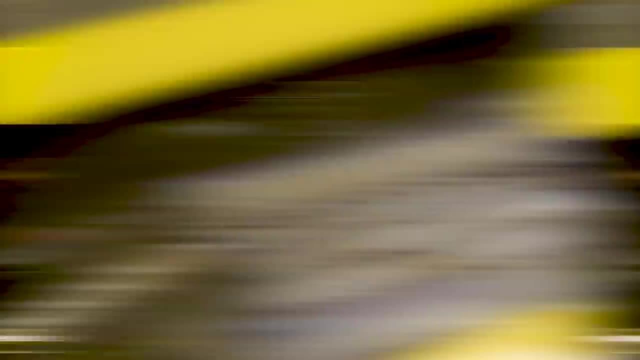 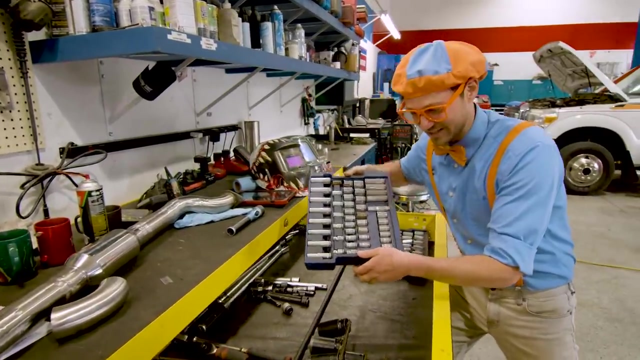 push yellow toolbox, uno. i think we should open it up and see what tools are inside. look at these socket sets. wow, that is so nicely organized. whoa remember earlier? yeah, we were talking about those nuts. yeah, these sockets are so nice. oh, wow, that is so nice to have. dop語, liver stuck in the trên. i see something in there. it's mine. i need to share mine, at least some, so it's safe. but let's see what it actually is. it's from action divine. oh my god, look at that. it's so beautiful. 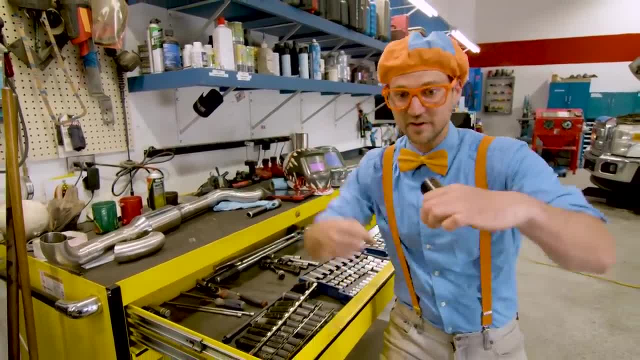 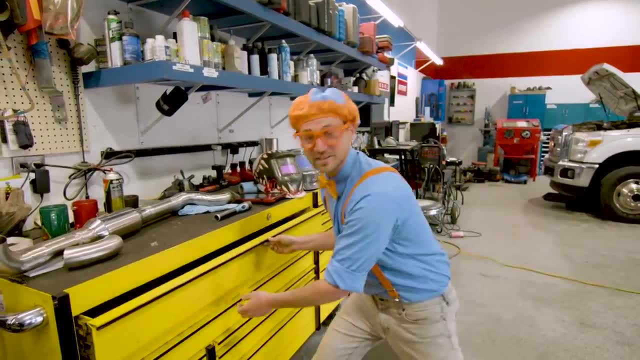 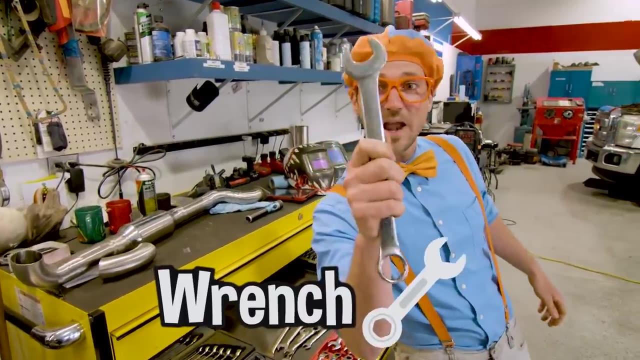 sockets go over the nuts and then you use a lever and then turn it and then you get it nice and tight. yeah, that is really cool. oh, let's see what else is in here. i love tools. they're so much fun. whoa, look, yeah, a wrench. yeah, you can also use these to tighten nuts. 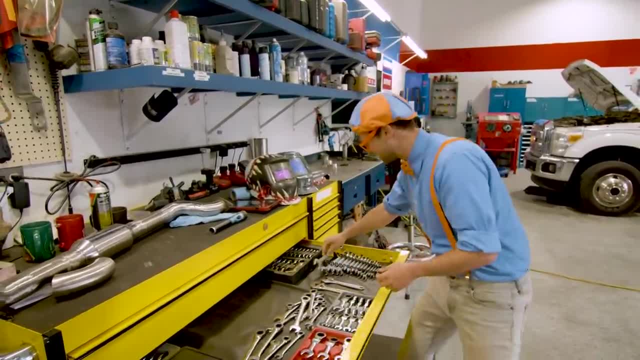 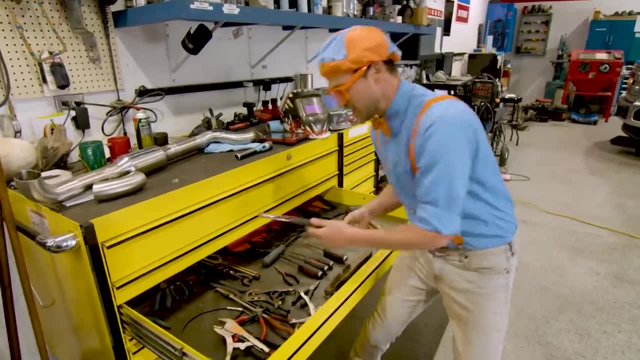 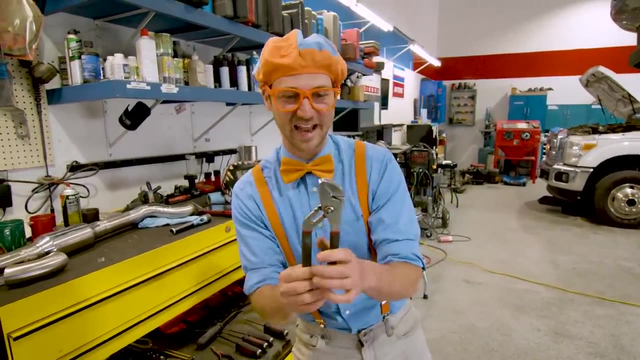 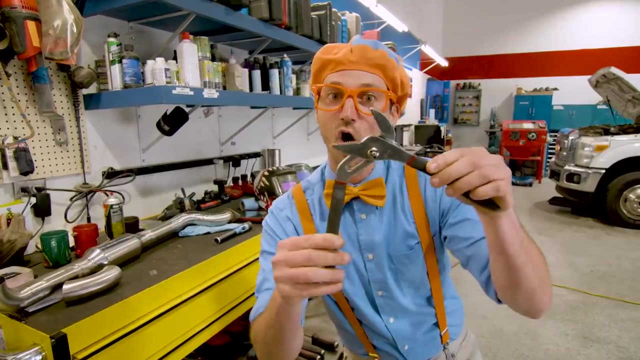 oh, that is so cool. all right, let's put it away. oh, what else is in here? whoa, yeah, a crescent wrench. whoa, we must have a customer. someone else will get that, but hey, check it out. a crescent wrench looks like a mouth. hello, hello. 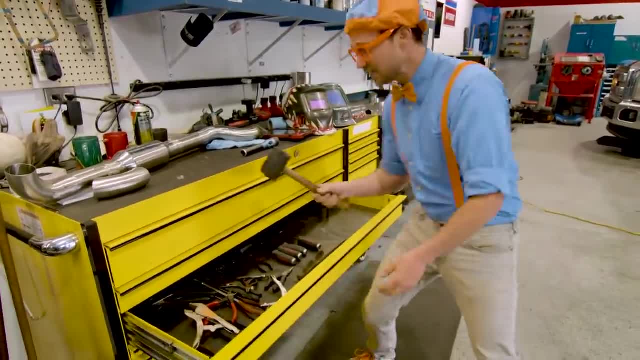 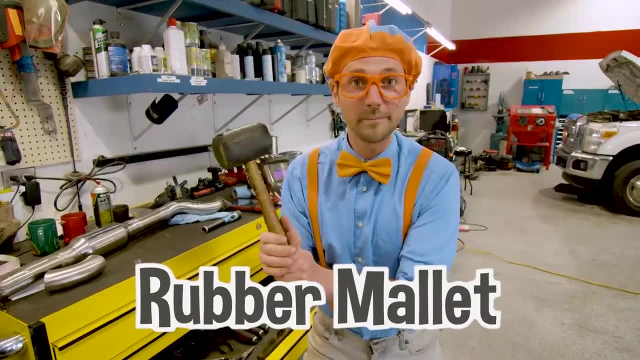 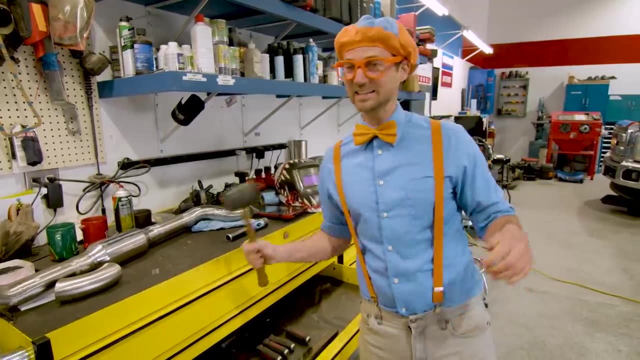 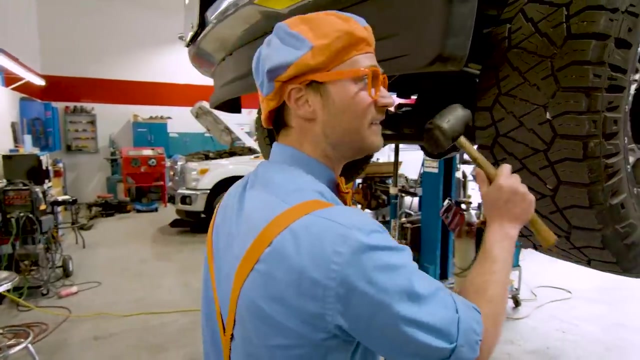 that silly, okay, well, oh, look at this. you know what this is. yeah, it kind of looks like a hammer, doesn't it? yeah, but it's actually a rubber mallet. watch this. yeah, you can hit things with it. yeah, you uh like a tire. watch this. i don't know what you would do that for, but 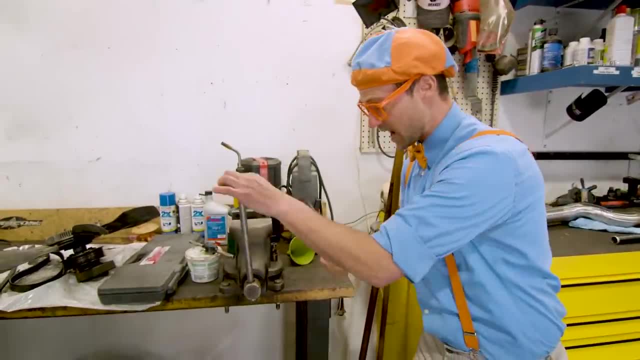 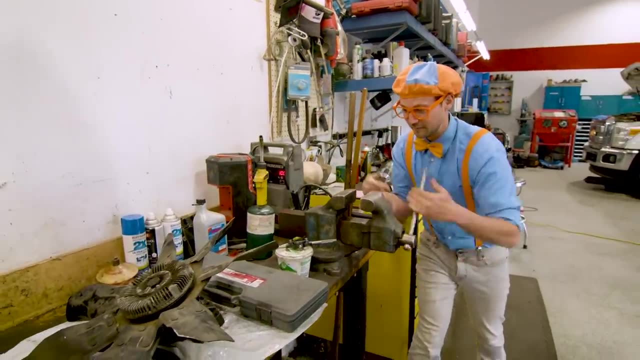 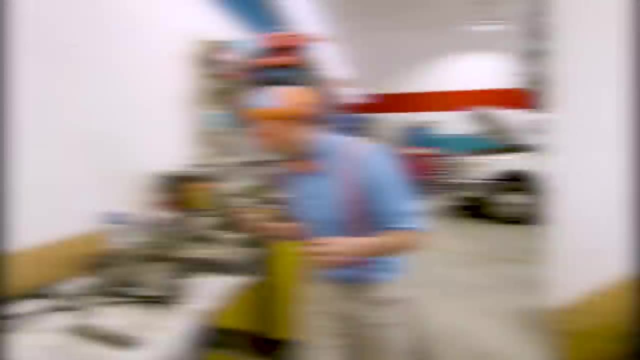 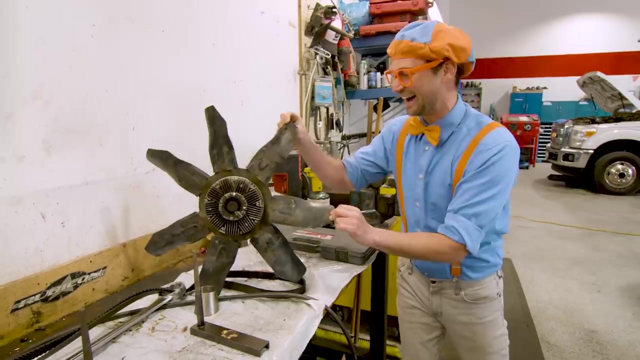 it's fun. whoa, yeah, a vice right here. yeah, you can put things in here, turn this and see it closing. yeah, keeps things held right here, so then you can work on it. yeah, looks like a fan. it looks like a fan. yeah, this looks like a fan that goes in front of the. 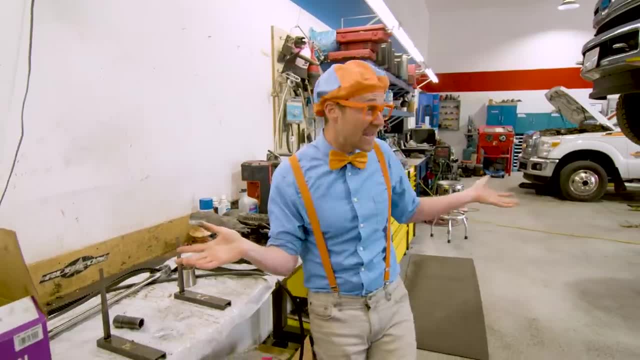 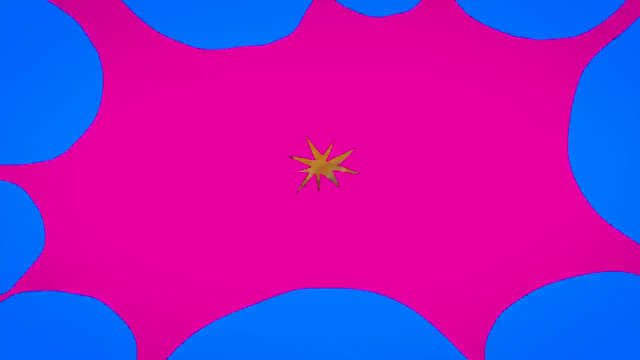 radiator. wow, i sure do love the radiator. wow, i sure do love the radiator. wow, i sure do love mechanic shots and tools. hey, i think this is the perfect time for the tool song, WHEN YOU'RE WORKING WITH TOOLS. WORKING WITH TOOLS, YOU HEAR ALL KINDS OF THINGS. 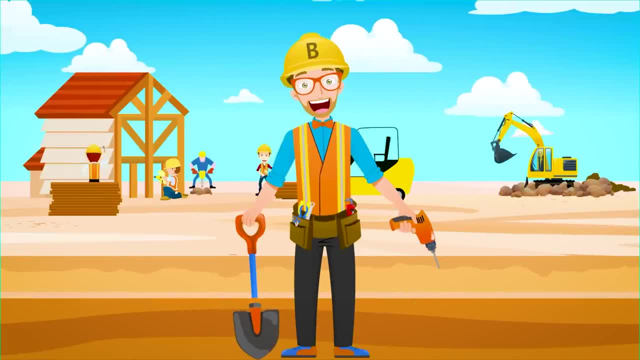 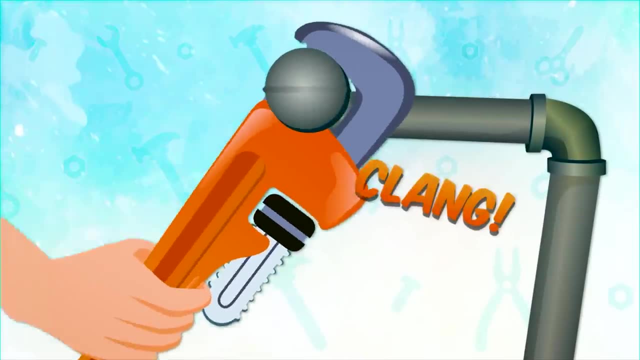 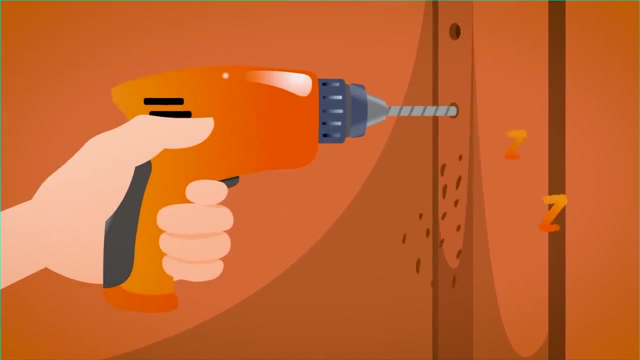 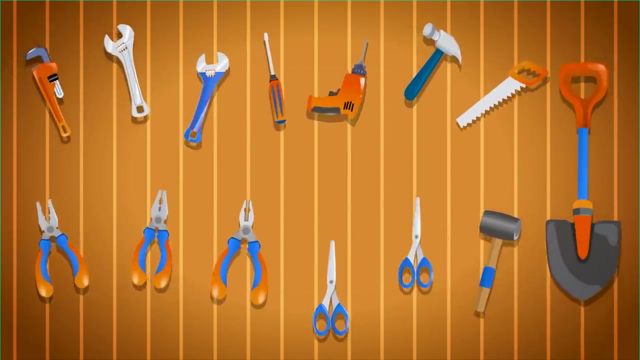 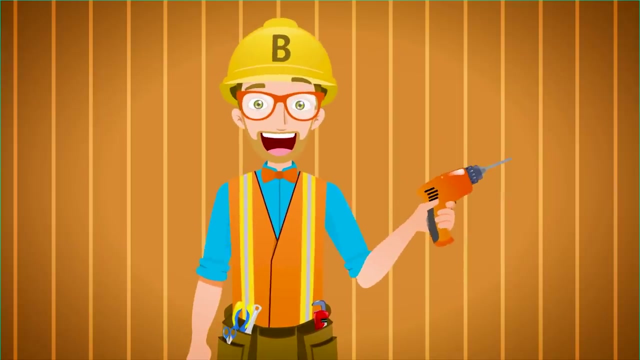 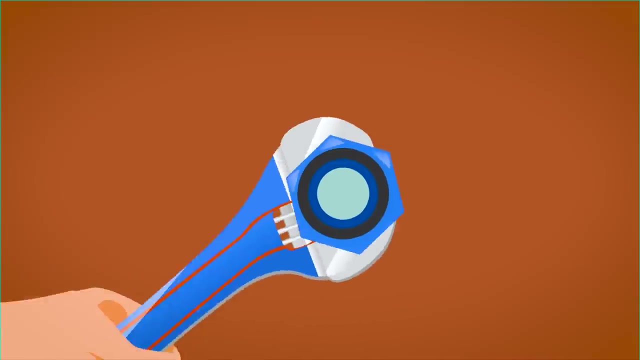 WHEN YOU'RE WORKING WITH TOOLS, YOU HEAR ALL KINDS OF THINGS: THE WзыNSCH TITANS, PIPE'S GOING CLANG, CLANG. A hammer hits a nail. going bang, bang, bang. A drill is making holes going zzzzzzzzzzzzzzzzzzzzzzzzzzzzzzzzzzzzzzzzzzzzzzzzzzzzzzzzzzzzzzzzzzzzzzzzzzzzzzzzzzzzzzzzzzzzzzzzzzzzzzzzzzzzzzzzzzzzzzzzzzzzzzzzzzzzzzzzzzzzzzzzzzzzzzzzzzzzzzzzzzzzzzzzzzzzzzzzzzzzzzzzzzzzzzzzzzzzzzzzzzzzzzzzzzzzzzzzzzzzzzzzzzzzzzzzzzzzzzzzzzzzzzzzzzzzzzzzzzzzzzzzzzzzzzzzzzzzzzzzzzzzzzzzzzzzzzzzzzzzzzzzzzzzzzzzzzzzzzzzzzzzzzzzzzzzzzzzzzzzzzzzzzzzzzzzzzzzzzzzzzzzzzzzzzzzzzzzzzzzzzzzzzzzzzzzzzzzzzzzzzzzzzzzzzz. 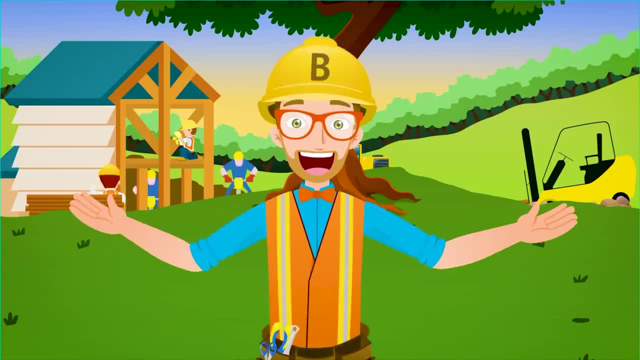 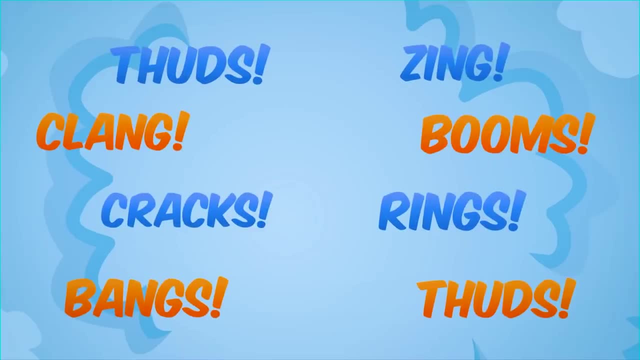 When you're working with tools, you hear all kinds of things. You hear bangs and booms, clangs and zings. When you're working with tools, you hear all kinds of things: Cutting wires with some pliers going snip, snip. 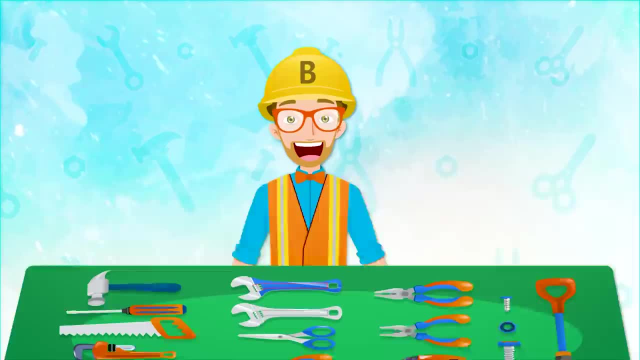 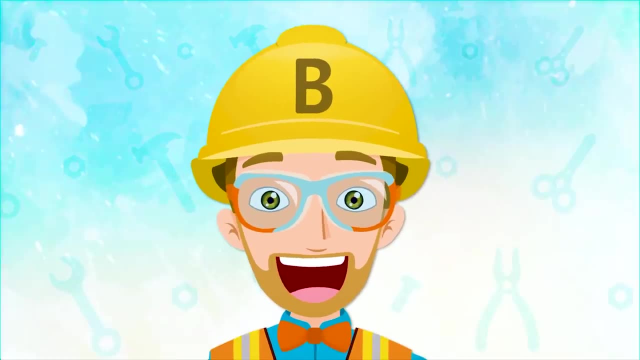 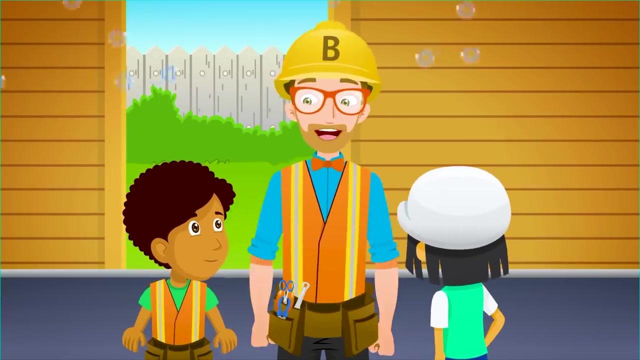 Cutting paper with some scissors going clip clip. When you're working with tools, you've got to be real safe By wearing gloves on your hands and goggles on your face. And, boys and girls, when you're working with tools, Always follow mom and dad's safety rules. 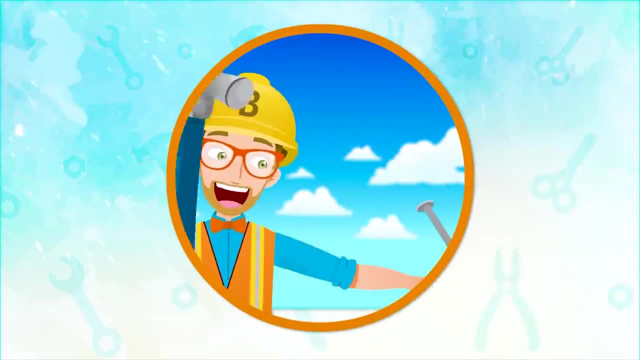 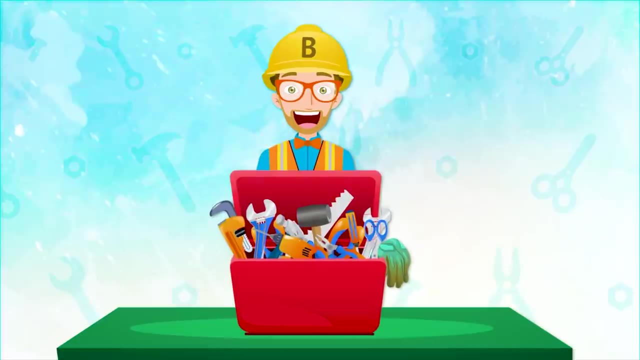 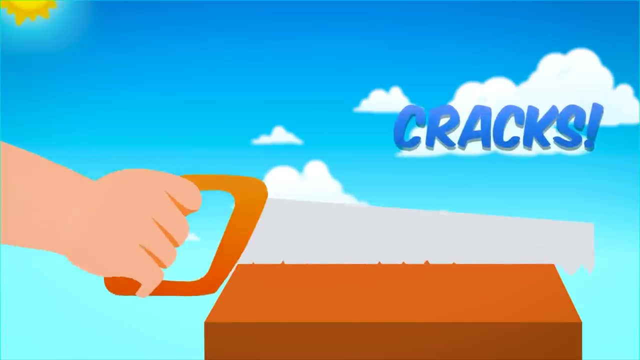 When you're working with tools- working with tools- You hear all kinds of things. When you're working with tools- working with tools- You hear all kinds of things. You hear thuds and squeaks, cracks and rings. When you're working with tools, you hear all kinds of things. 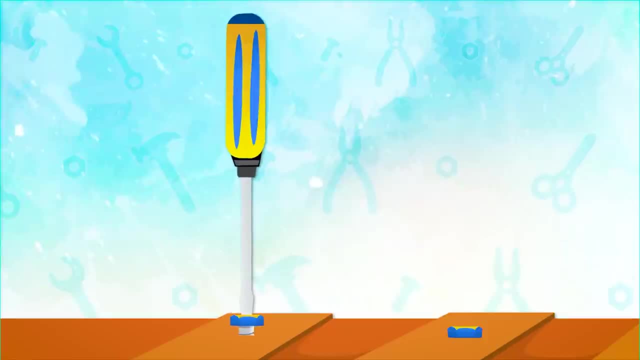 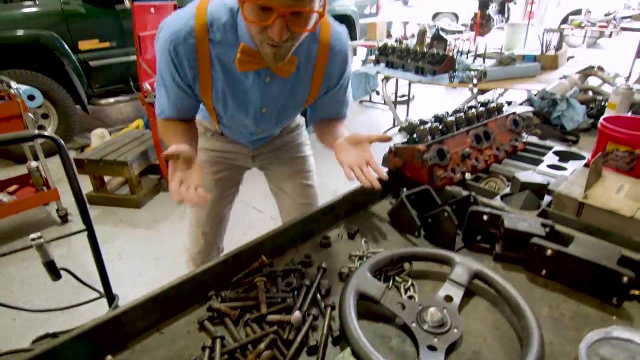 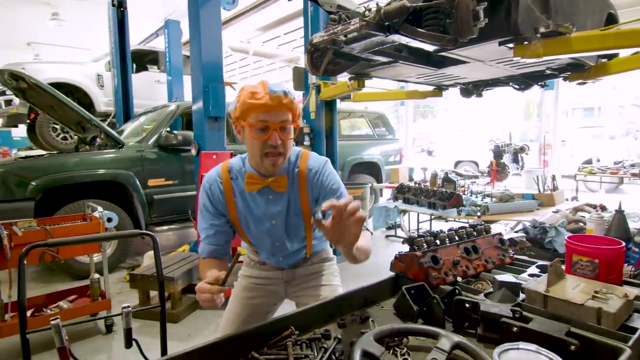 You hear bangs and booms, clangs and zings. When you're working with tools, you hear all kinds of things- Whoa. Check it out. Yeah, it looks like we have some big bolts. Whoa, And we have some big nuts. 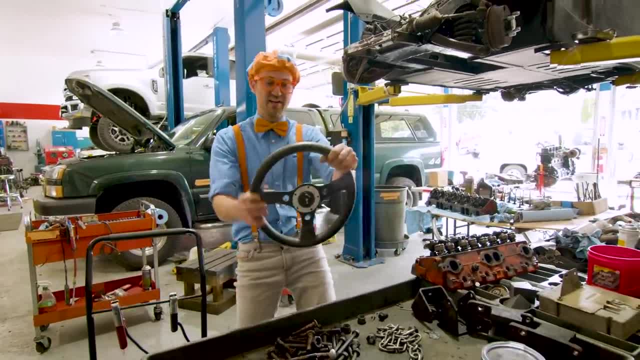 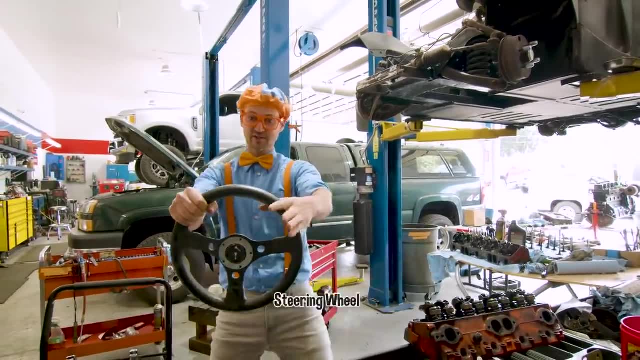 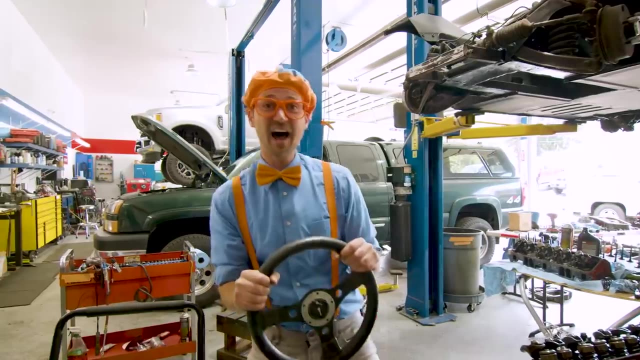 Whoa, Hey, what's this doing here? You know what this is? Yeah, it's a steering wheel. Ten and two. Driving a car is so much fun. You'll get there And you need to be very safe and always wear your seatbelt. 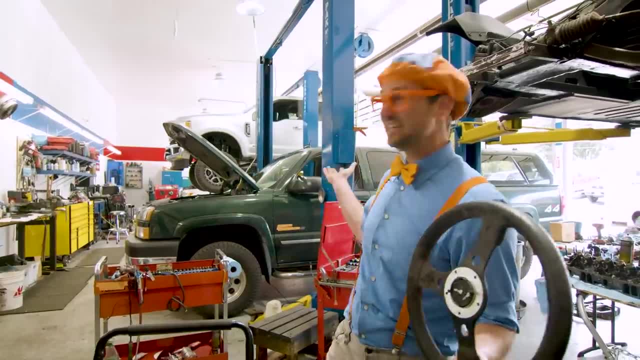 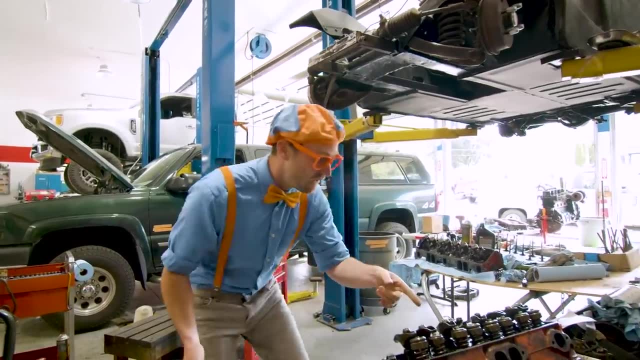 But hey, in order to drive your car, you need to maintain your vehicle. Yeah, and that is why we're at the mechanic shop. But hey, check these out. Whoa, this is the cylinder head. Whoa, There's so many parts to an engine. 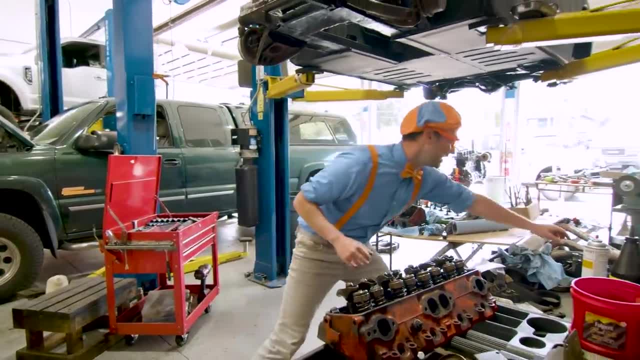 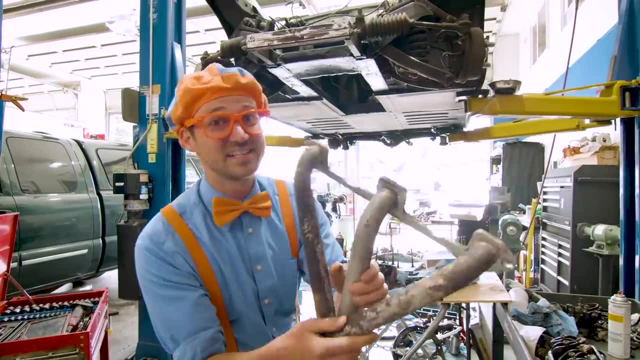 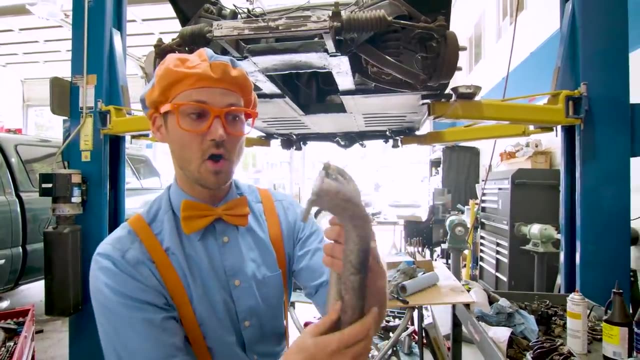 And this is just one of them. Whoa. And over here this is the exhaust manifold. Whoa. Yeah, like I said, there's a lot of parts to an engine, But this is where the engine is. And then the exhaust goes through all these pipes to the back of the vehicle. 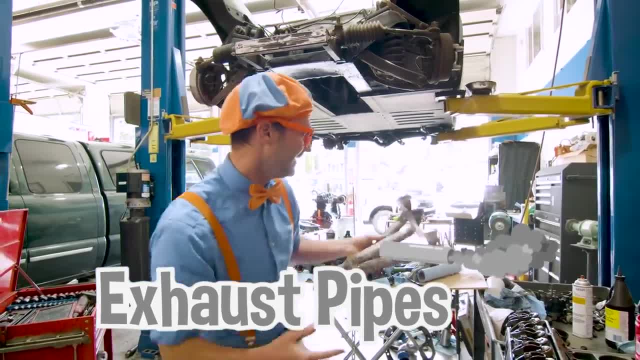 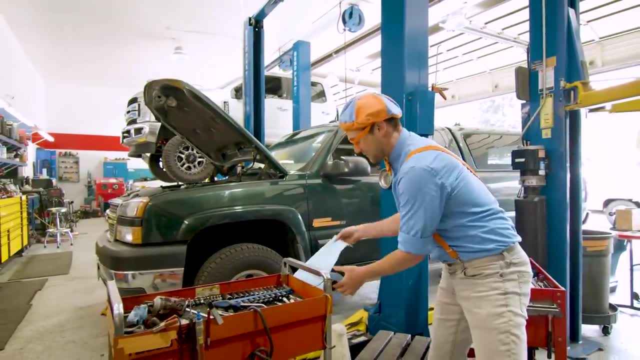 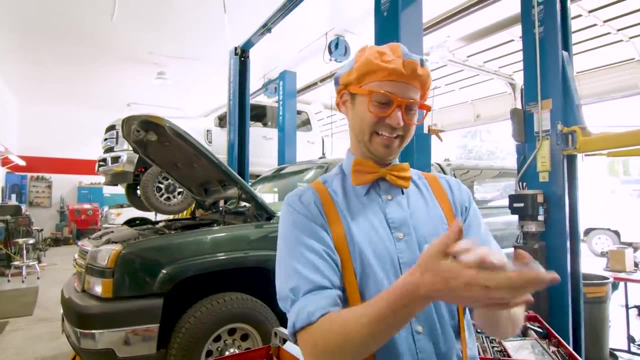 Yeah, and you've probably seen exhaust pipes before, Yeah, Well, hey, I have one last thing to show you right over here. The best part about mechanic shops is cleaning up. at the end of the day, And all your hard work pays off. Well, this has been so much fun learning about tools with you today. 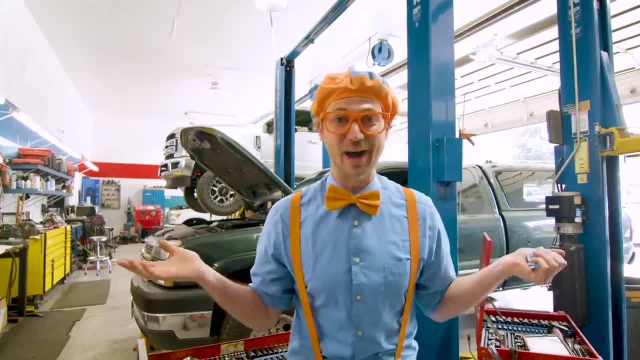 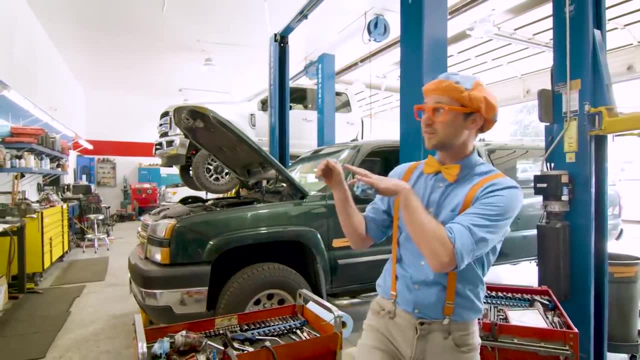 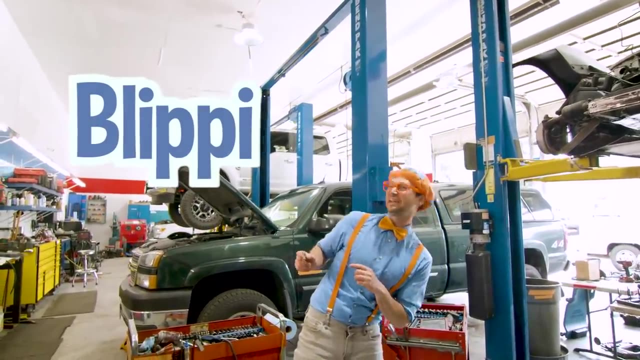 And welding and what it's like to be in a shop. Well, this is the end of this video, But if you want to watch more of my videos, all you have to do is search for my name. Will you spell my name with me? B-L-I-P-P-I, Blippi. 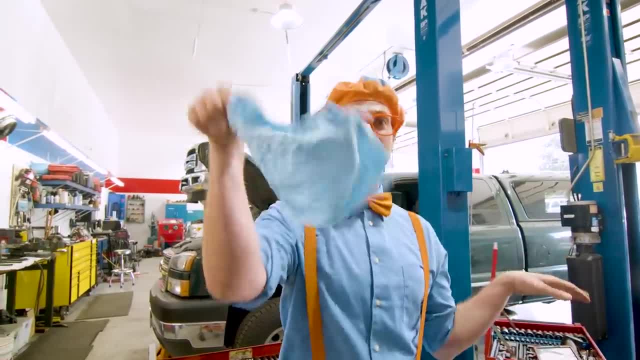 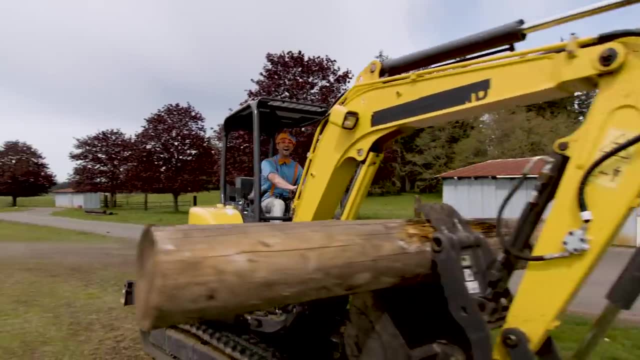 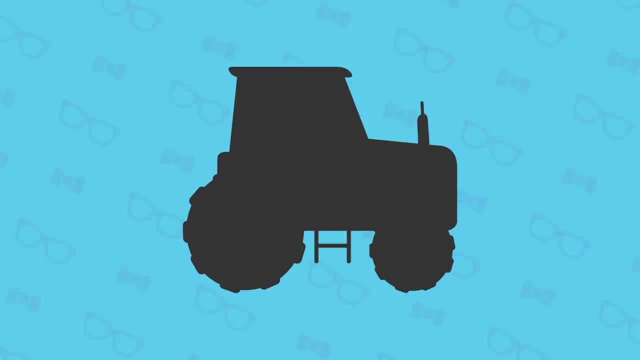 Good job, Alright, see you again. Buh-bye Wee. Hey, it's me Blippi. Today we're going to learn about some construction vehicles. They are so big and powerful. Can you guess which construction vehicle this is? 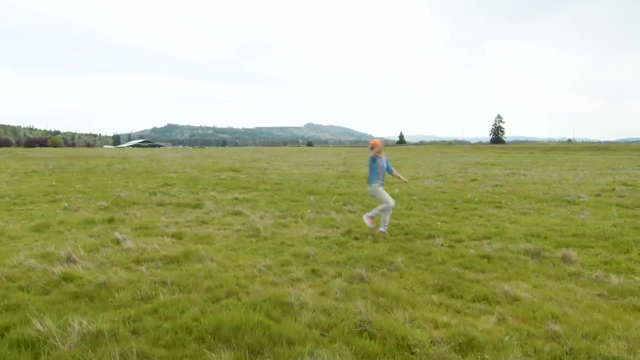 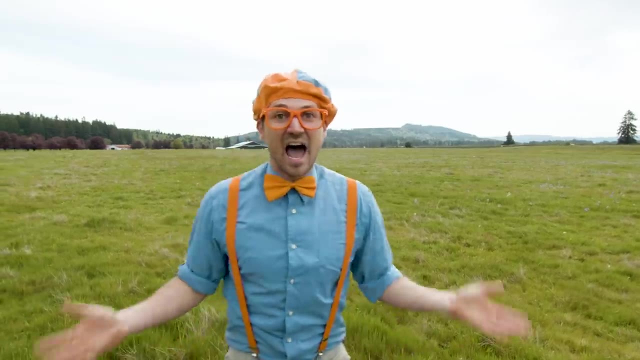 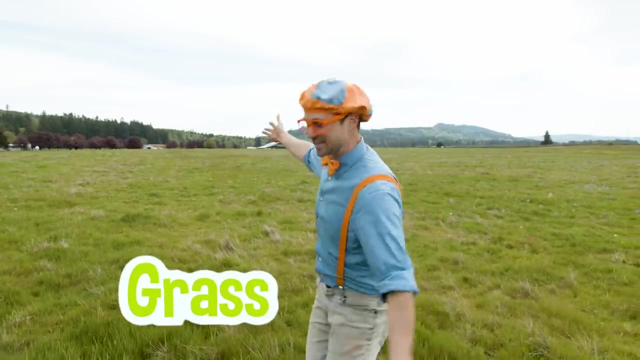 Let's go find out. Hey, it's me Blippi, And look at where I'm at. Yeah, today I'm in Tenino, Washington at a ranch. Yeah, Check it out, all this beautiful grass, Wow, Hey. but today we're going to explore a machine. 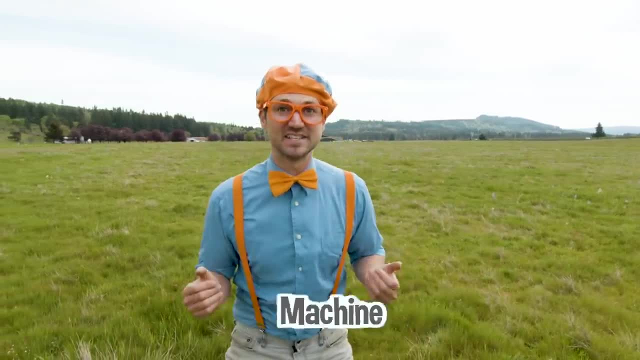 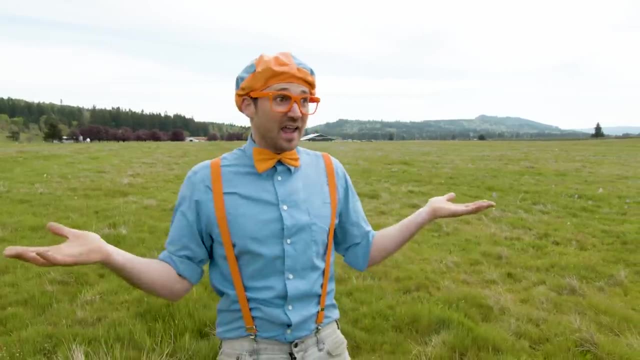 Let me give you some hints on what machine this is. So it's a machine that you can use in this big open field. Yeah, for crops. Yeah, It starts with the letter T. You can have a lot of attachments on it. Do you know what it is? 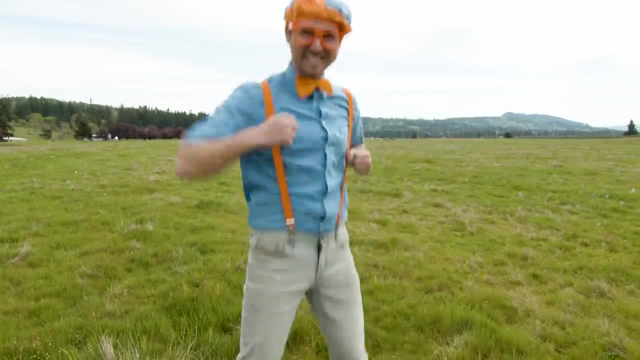 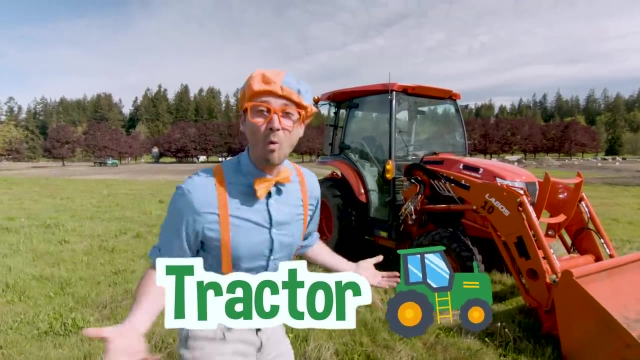 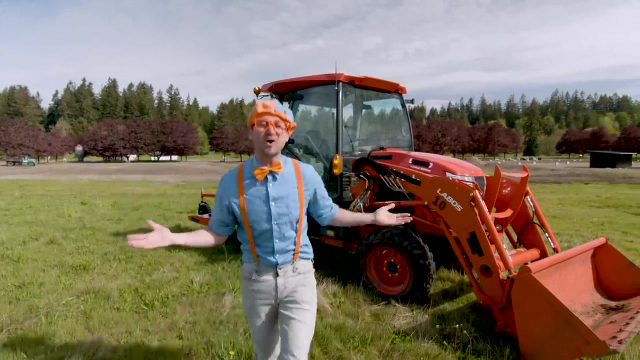 Yeah, let's go. Whoa, Check it out. This is a tractor. Whoa, Tractors are so cool. Typically you use them on farms and ranches. They get so much work done. Hey, check it out, Whoa. 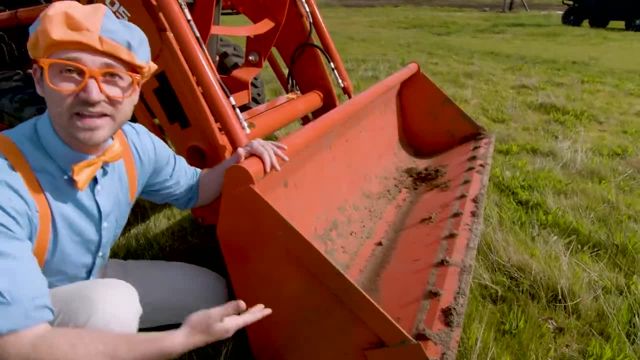 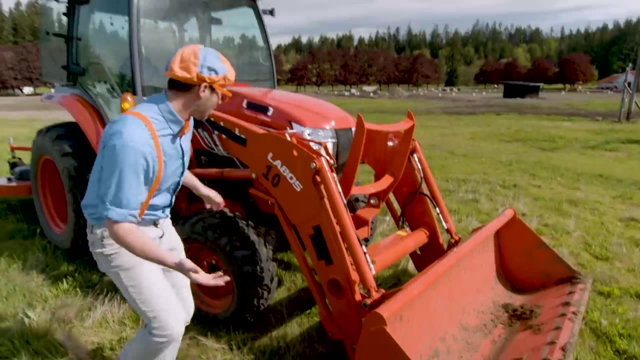 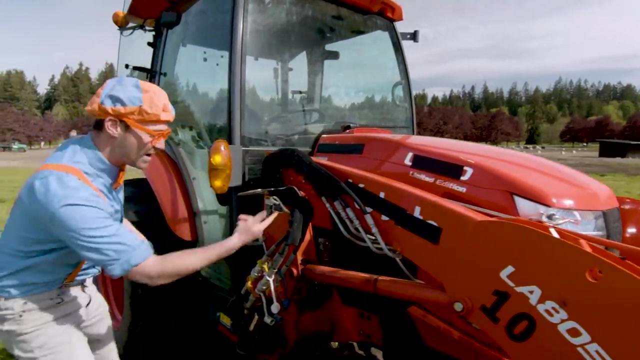 Whoa, Do you see this? This is a big bucket And it can scoop a lot of dirt and gravel and things like that. Whoa, Wow, These are the bucket arms which help lift the bucket. Whoa, Right here. these are the hydraulic hoses. 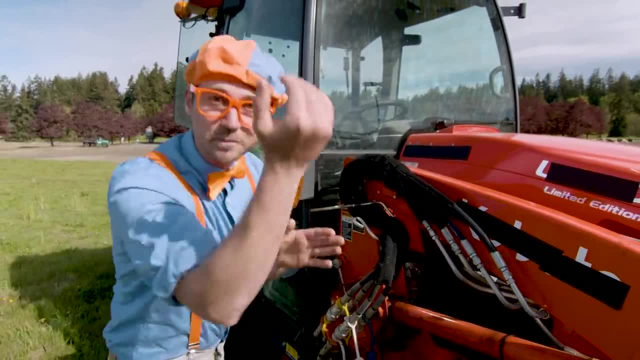 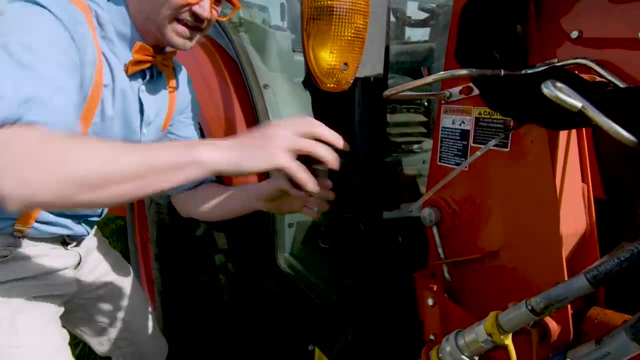 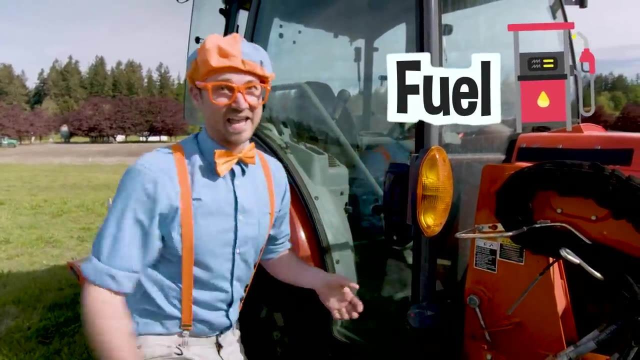 Which help tilt and scoop things up and lift up the bucket. Oh, And you know what this is? Yeah, This is where you fill up the tractor with fuel, And this tractor doesn't take gas, It takes diesel. Yeah, Whoa, That right, there is the cab. 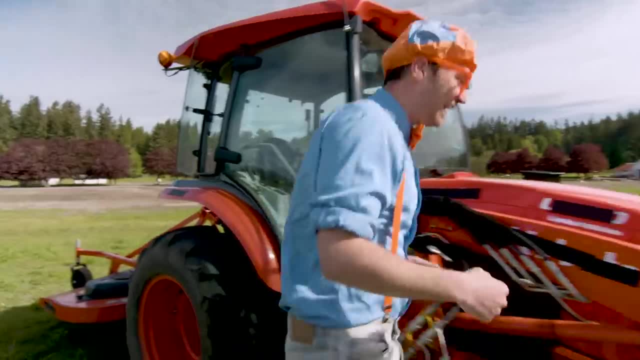 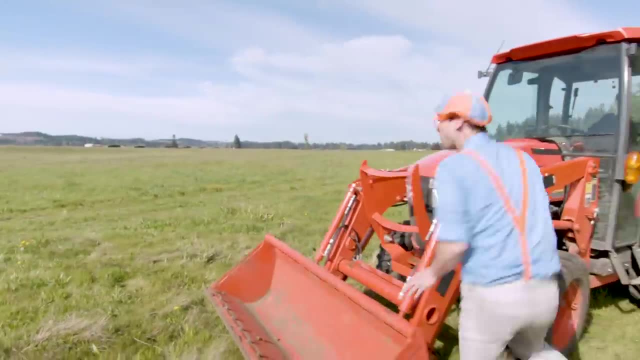 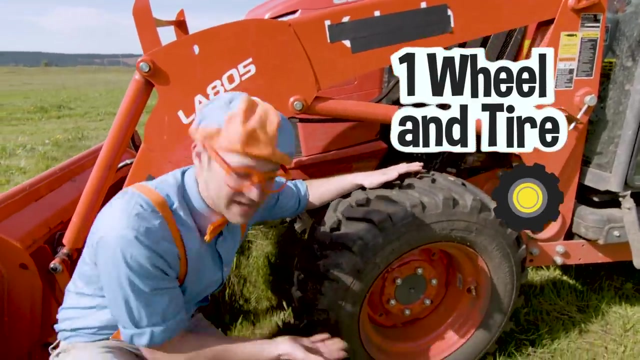 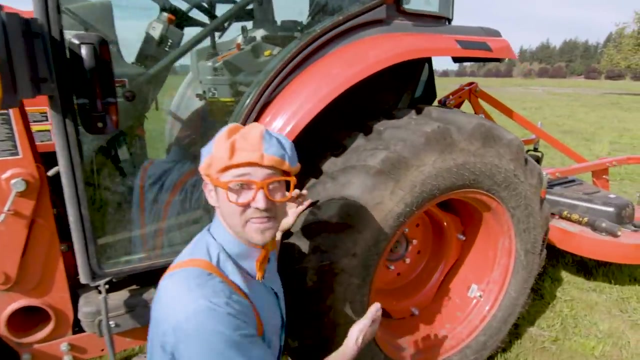 Here. come on to the other side. Let's go: Whoa, Hey, This tractor, Yeah, Has one big wheel and tire. Yeah, Whoa, Look at this over here. Whoo, Now, this is a big wheel and tire, Hey. 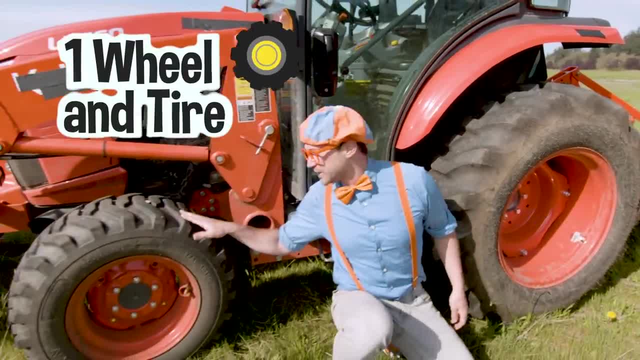 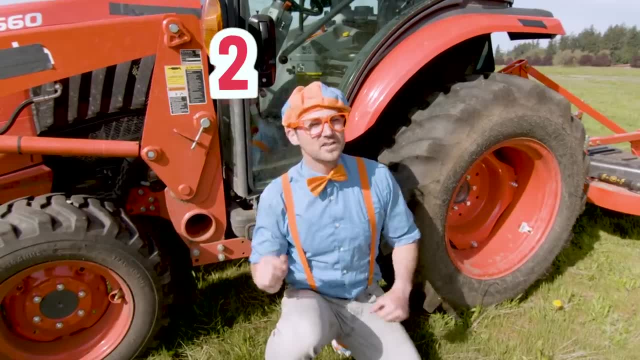 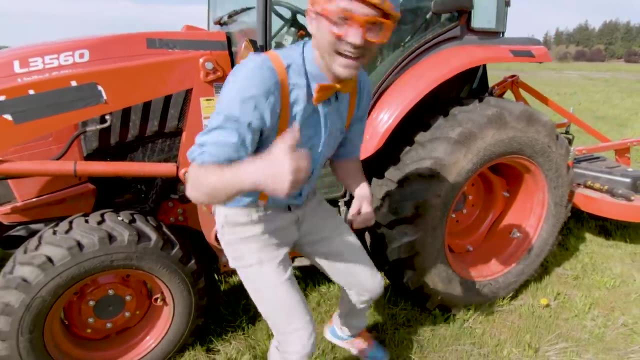 Did you notice? It has one wheel and tire, Two wheel and tires, And the other side have two more. So that means two plus two equals four. Yeah, Good job. Wow, Check out the back of the tractor. Yeah, This is a mower attachment. 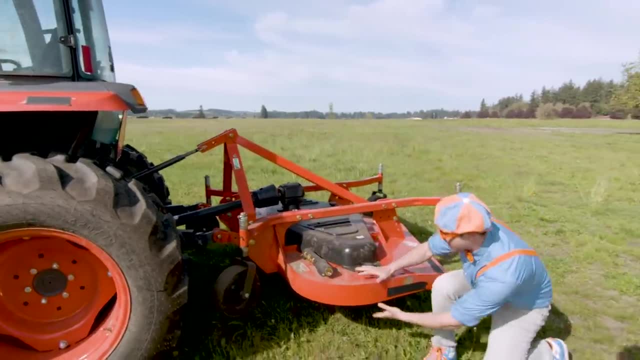 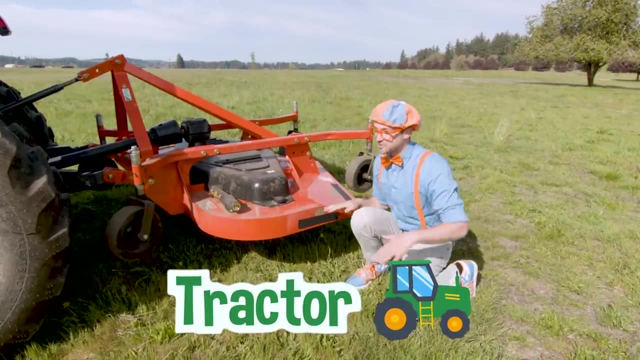 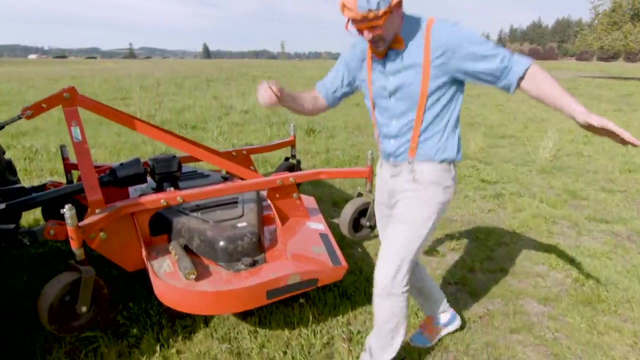 Wow, On the back right here there's some blades And this attaches to the tractor And this is what you use to go across grass like this. Chop it down and then you have a nice yard to play in. Woohoo, Haha, Yeah. 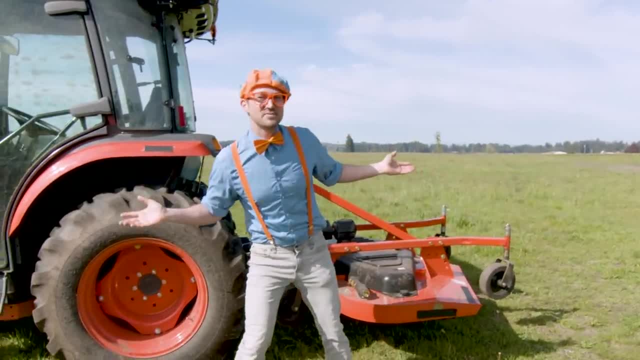 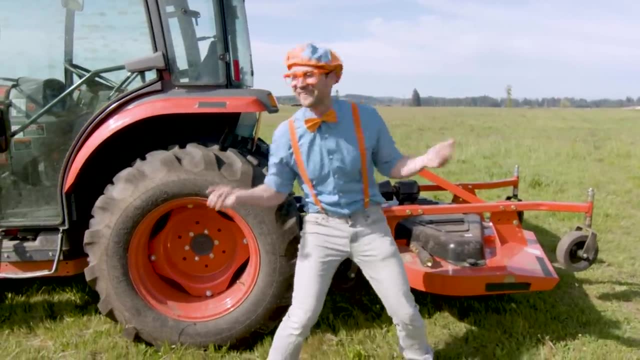 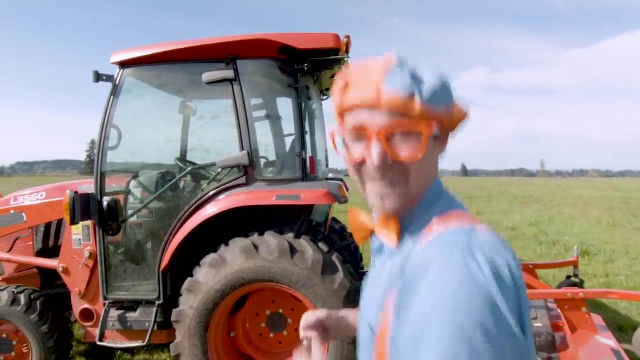 But hey, tractors have a lot of attachments. they can have Like augers or balers or hay fluffers. Whoa, That is awesome. Hey, now I think we should head inside and drive the tractor. Yeah, Let's go. Whoa. 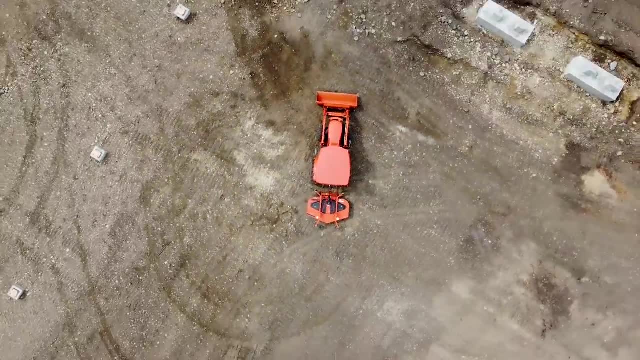 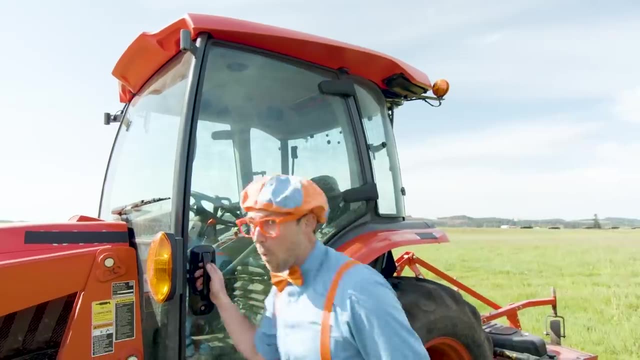 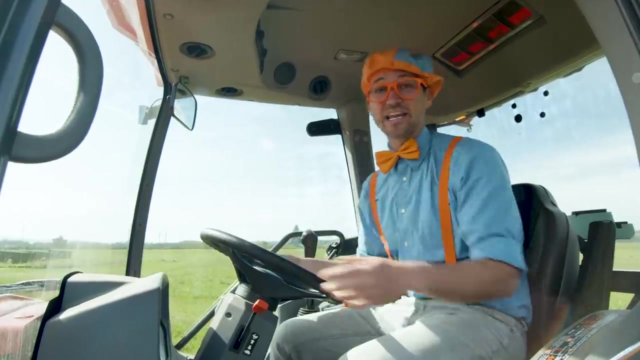 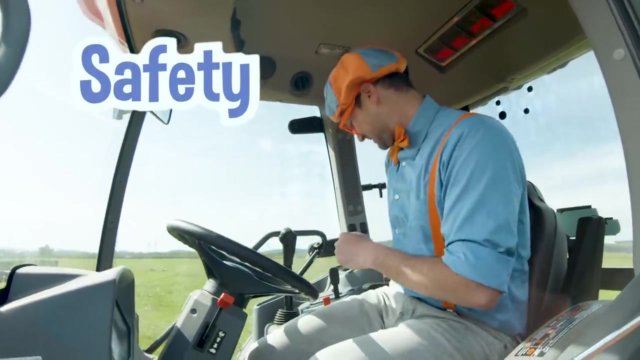 Here we go. Haha, Whoa, Check this out. Yeah, We're inside the cab of the tractor. Okay, first things first. Yeah, Safety first. Yep, That means we have to wear our seat belt. Perfect, Alright. 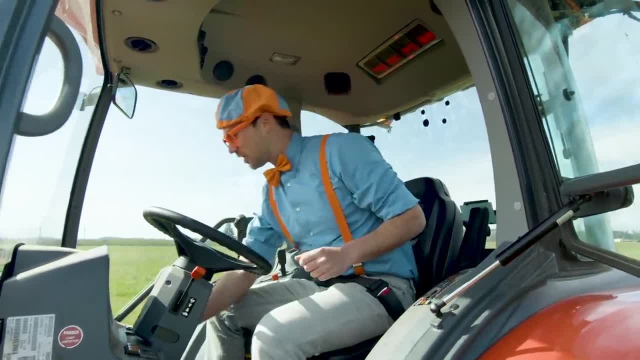 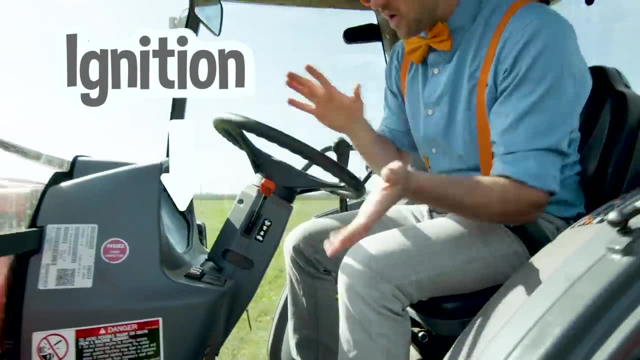 There we go. Now that we're all buckled up, we can take the key and put it in the ignition and start it up, But for now let me show you all the things in here. Yeah, Down here, these are the brakes of the tractor. 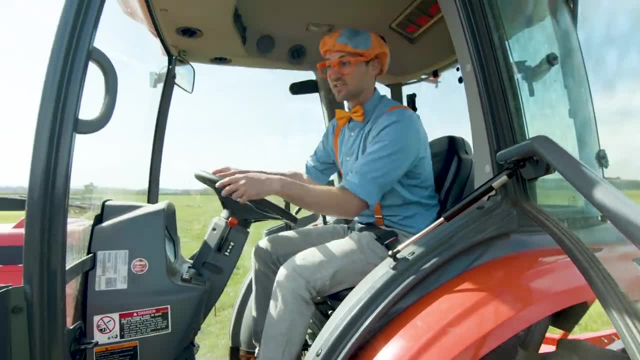 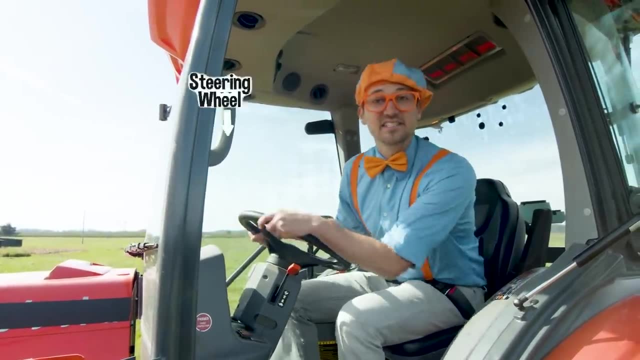 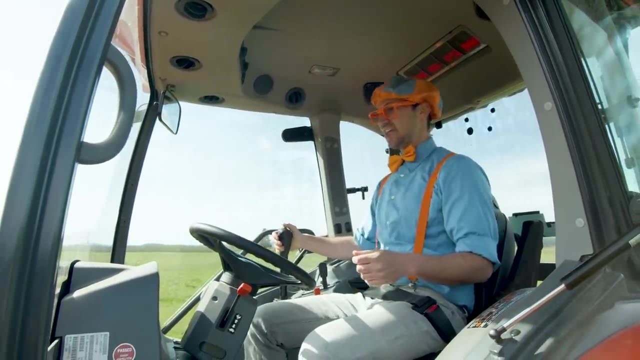 Yeah, Those are what you put your feet on. so then you stop the tractor in its tracks or tires, Haha, Yeah, And this right here. This is the steering wheel. This is how you operate and drive the tractor. Yeah, And this handle right here. you pull back to lift up the bucket, you push forward to 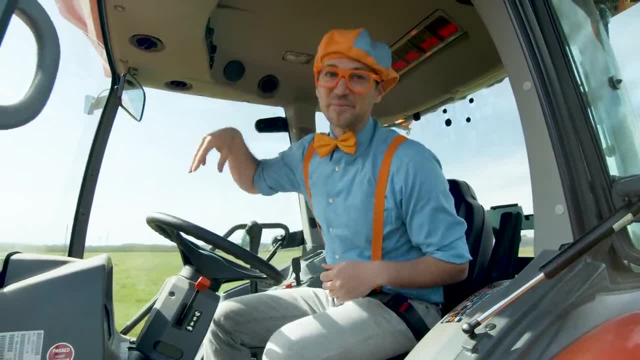 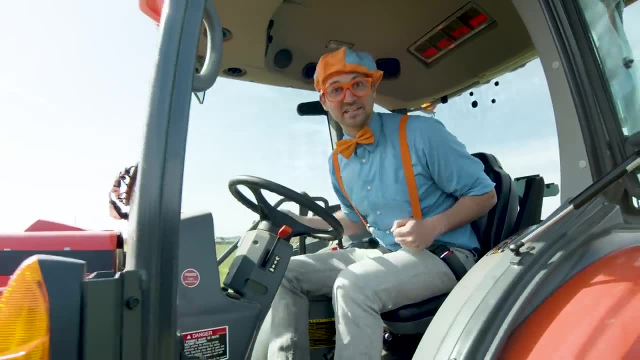 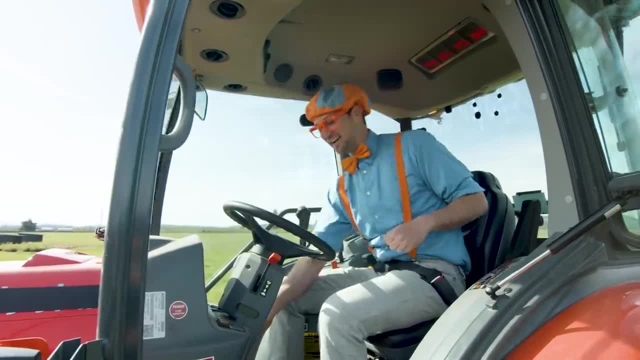 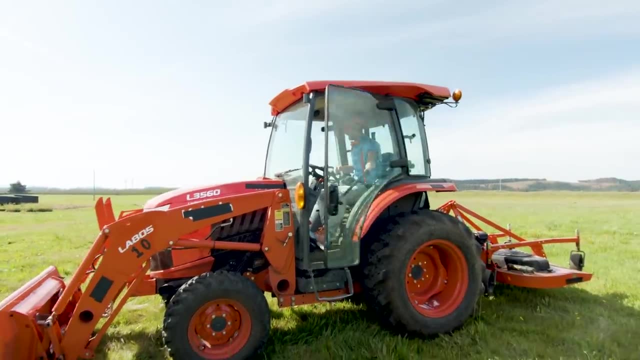 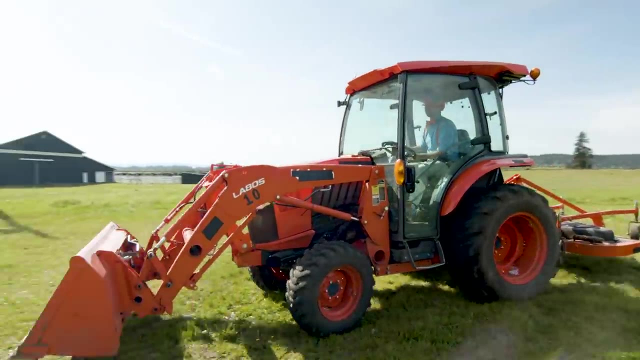 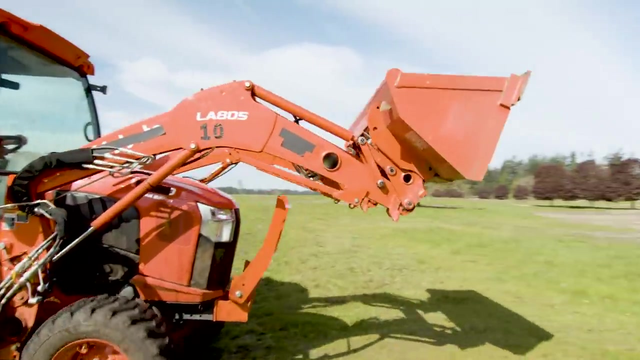 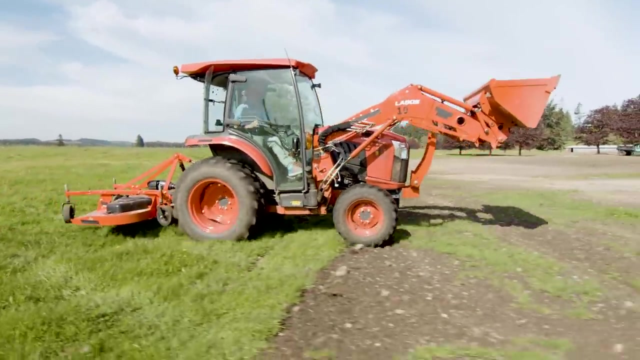 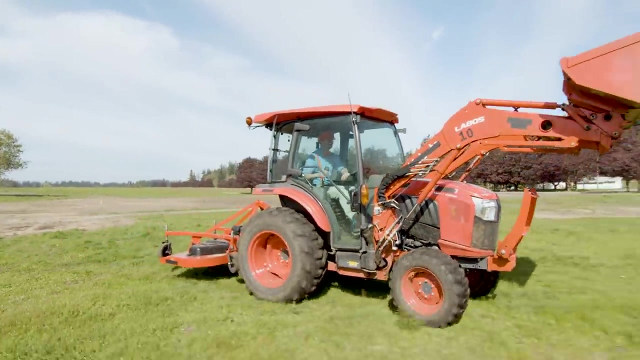 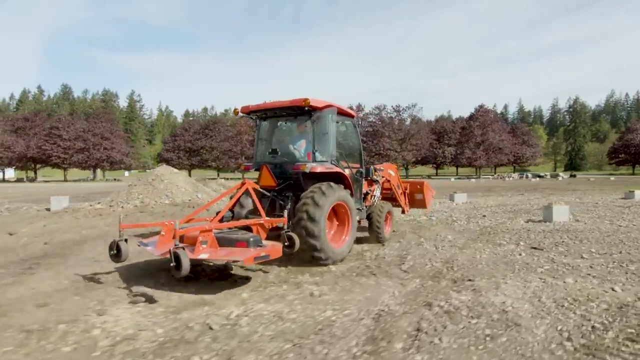 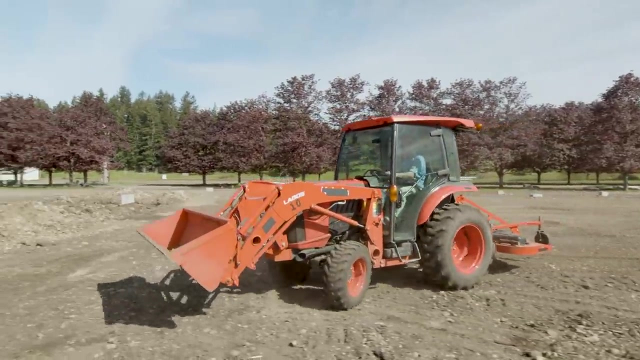 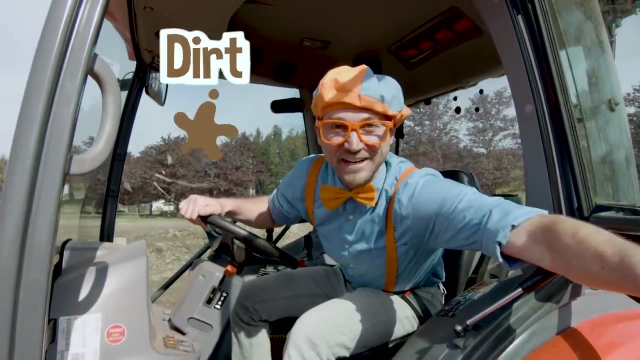 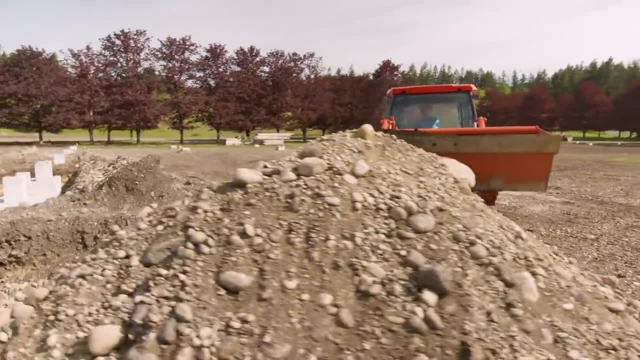 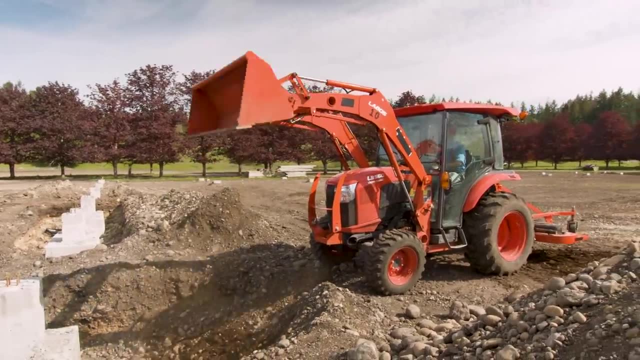 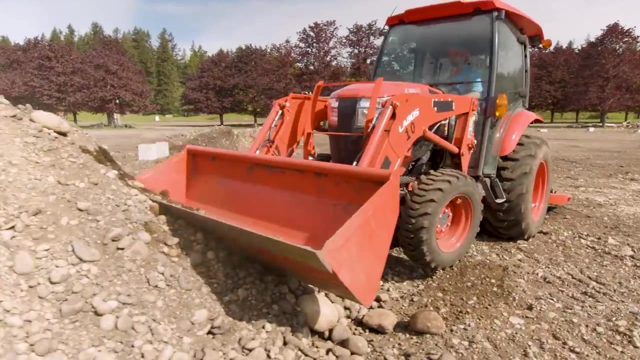 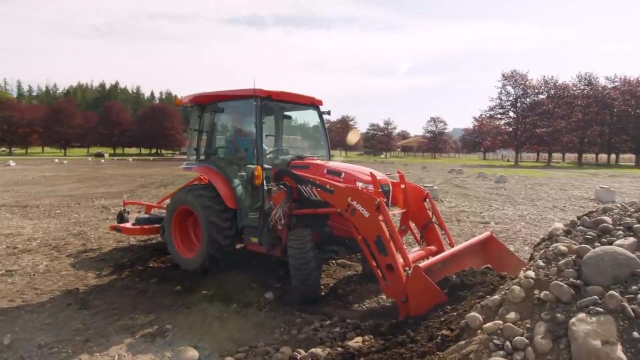 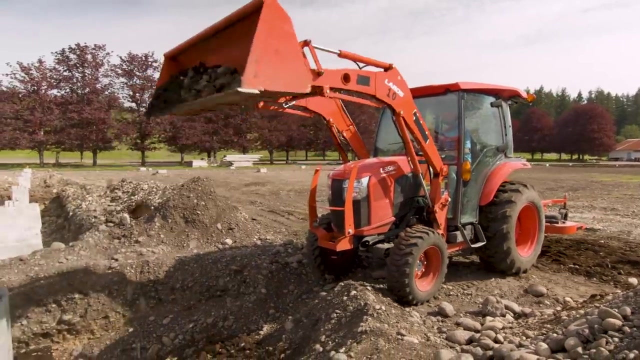 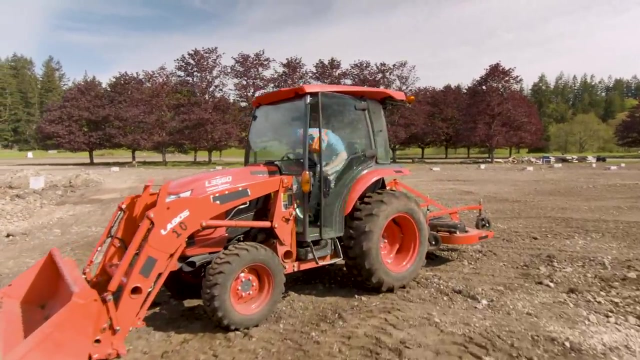 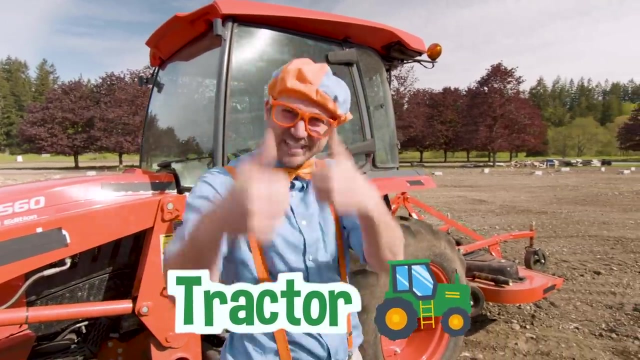 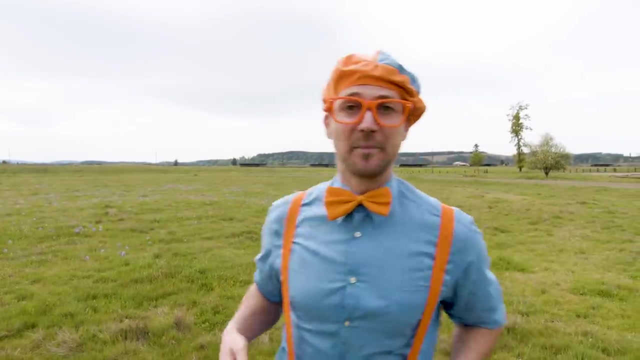 Now it's time to scoop up some dirt. Whoa, did you see that? Yeah, this tractor is so useful. Good job. Whoa, isn't that a cool machine? Yeah, it was so fun operating and driving that tractor. 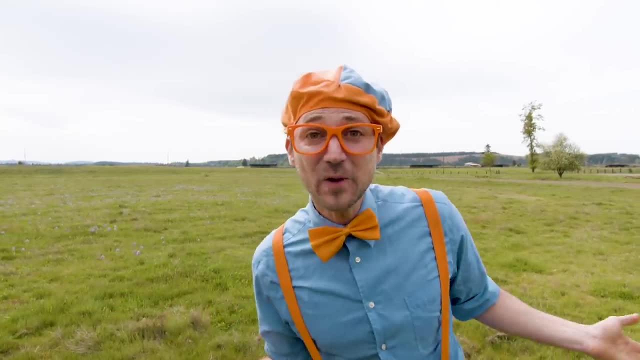 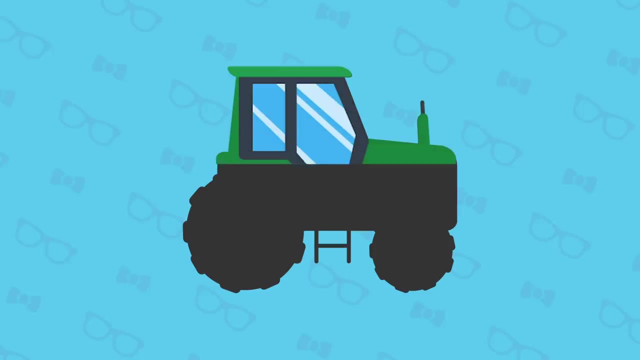 Wow, what a useful machine that you can use on farms and ranches. Whoa, Whoa, so cool. So many attachments and so many uses. Yeah, we learned about a tractor. Construction vehicles are awesome. Can you guess what this construction vehicle is? 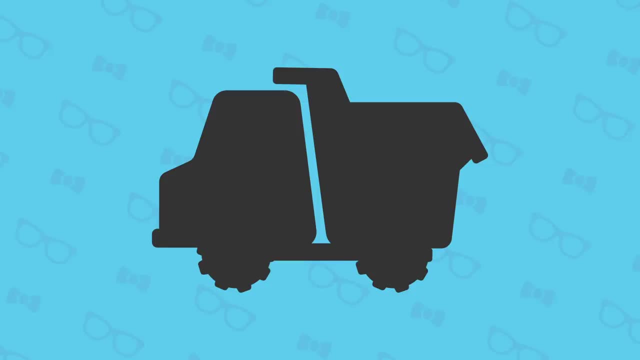 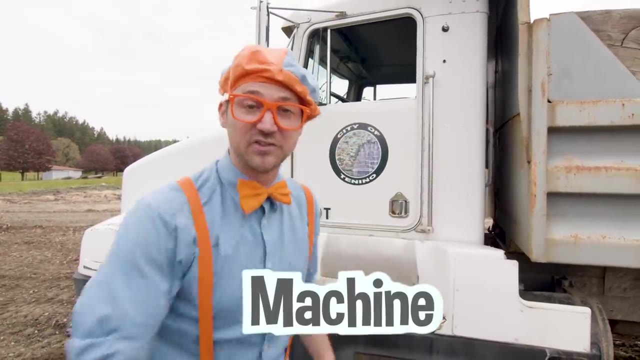 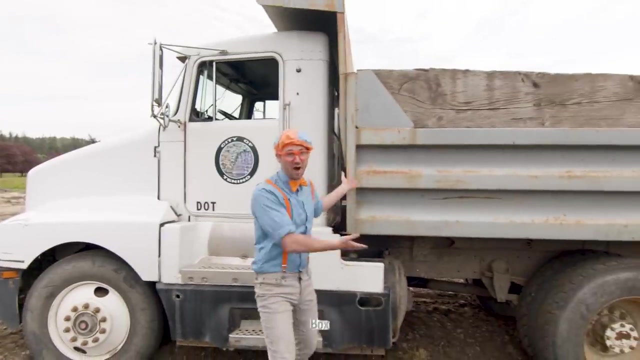 It has huge wheels. Let's go find out. Wow, check out this machine. Do you know what machine this is? Yeah, it looks kind of like a truck, But it has a giant body And right here, it does not have an echelon in this adapted vehicle. 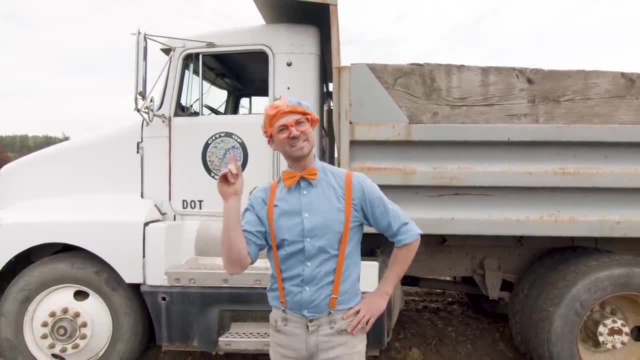 It's just a little bit that sucks in a little bit And it's very small And it storms It just few of itself. So basically it is a very big thing. We're going to go back to the rigging. 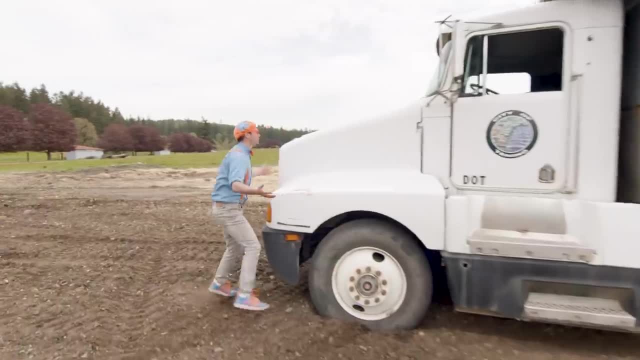 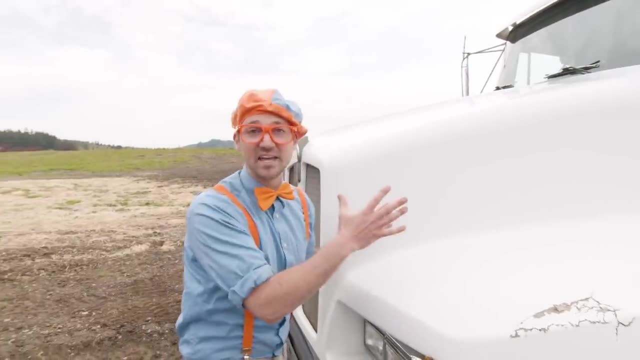 And after some work we're going to go back out there and take a look at the structure of this truck. Let's see how we did it. This little piece of junk is the bottom, with a lot of pressure. Let's look at the vent. 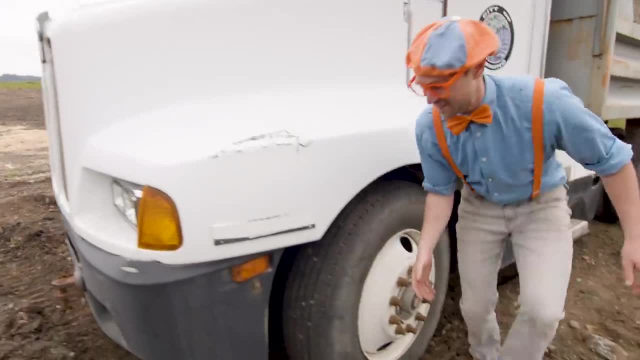 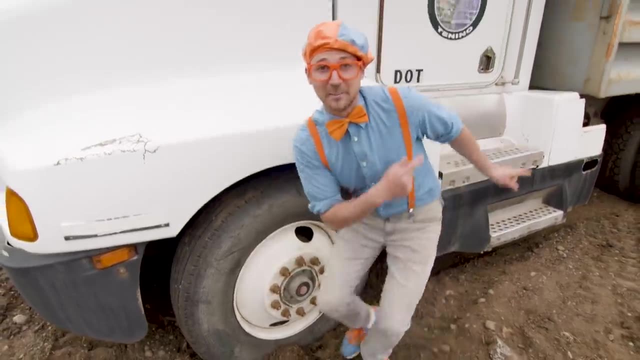 The vent must have a lot of pressure. Right underneath it. It's completely locked. You don't want to do this, Yeah right, Yeah, Yeah Yeah. these are wheels and tires. Whoa, this vehicle is really cool because in back there's a lot of them. 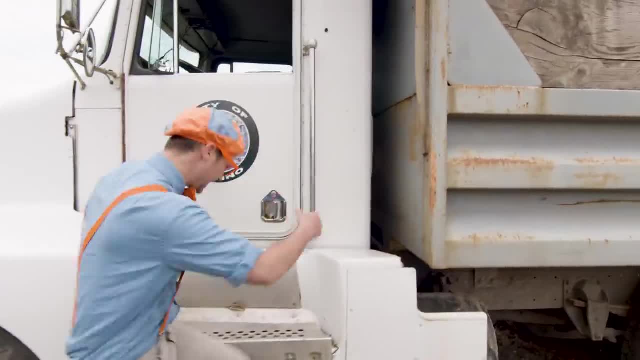 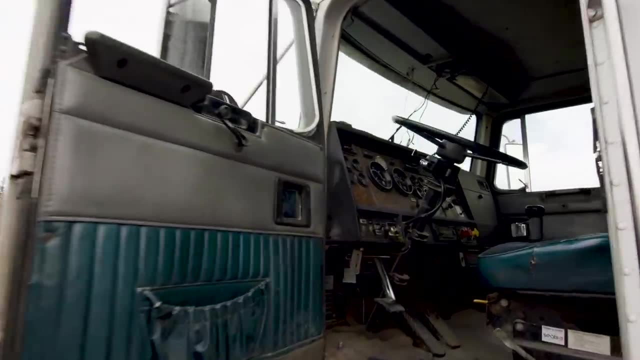 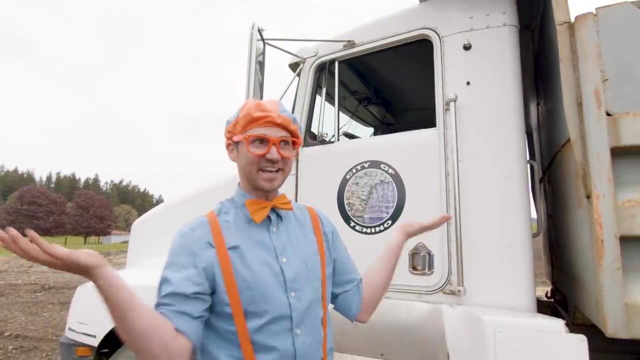 I'll show you that now, But first we need to check out the cab. Whoa, This is where the operator sits. Whoa, check it out. Whoa, there's a lot of things in there, just like a normal vehicle. 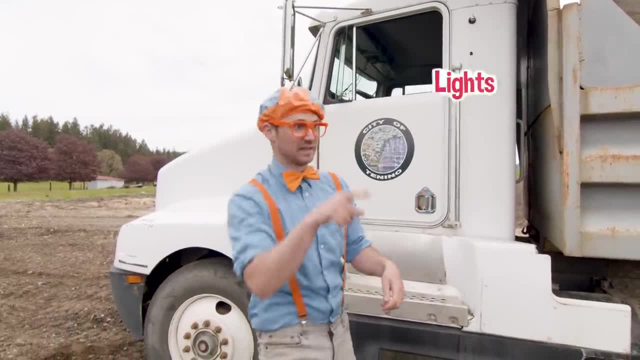 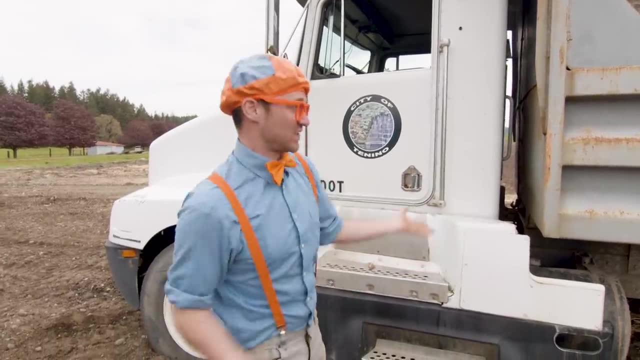 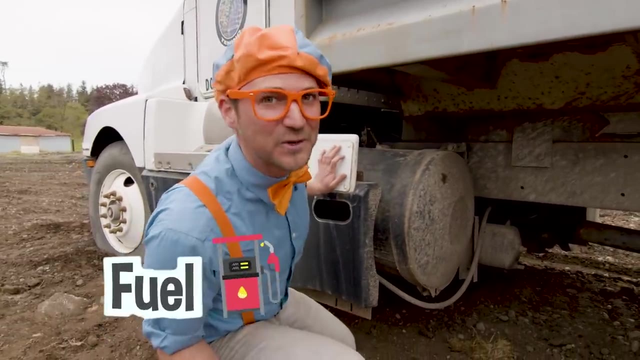 A steering wheel, some lights, there's also a mirror, there's a key to start it and a bunch of gauges and gadgets, so then you can operate it. Whoa, But this machine needs a lot of fuel to run. Yeah, I called it fuel, because it's not gas, it's diesel. 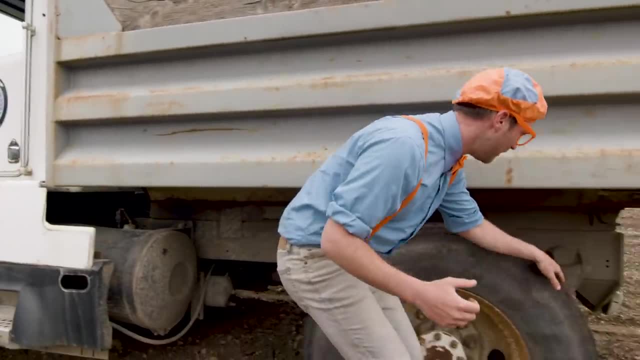 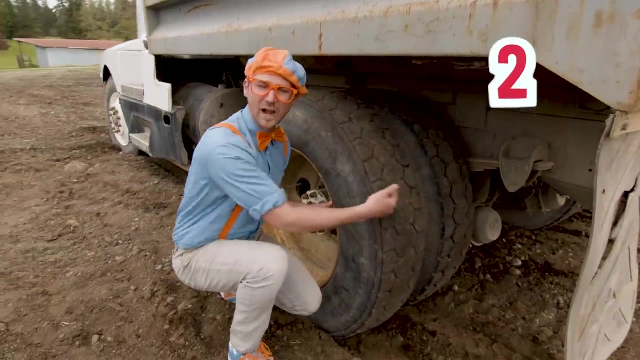 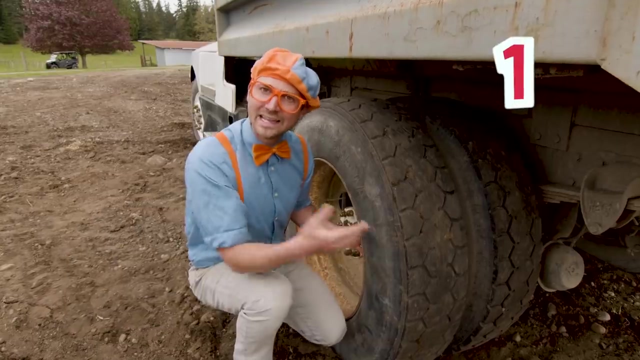 Whoa, Look Yeah, Do you see how many wheels and tires This vehicle has? Look, there's two right here. Normally they only have one in the front and one in the back, but this has two in the back. 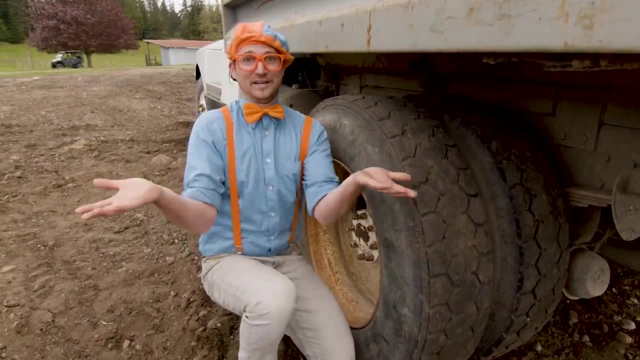 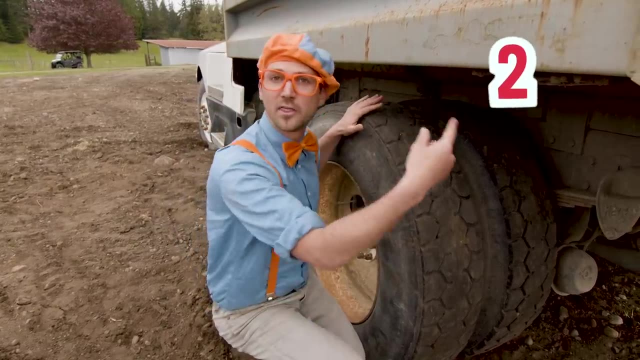 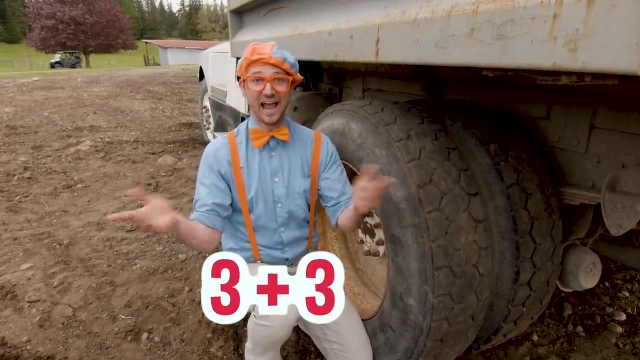 Yeah, and that is multiplied by two because it's on each side. So that means on one side there is one, two, three, Yeah, And you can add three on this side to the other, And on the other side, three plus three yeah is six. 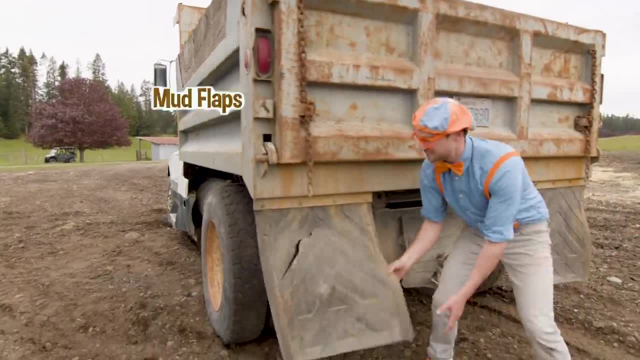 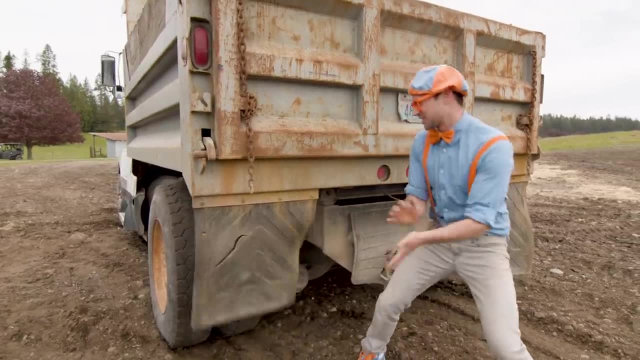 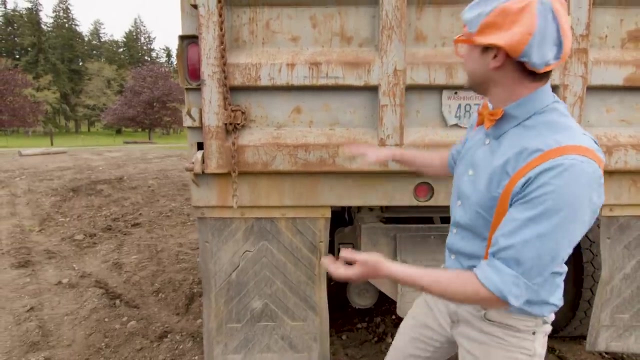 Whoa, these are called mud flaps. woohoo, because they flap like a dog's ear. woohoo, Actually, what it's used for is so then mud doesn't fling out to the vehicles trailing it. Yeah, and look at this. 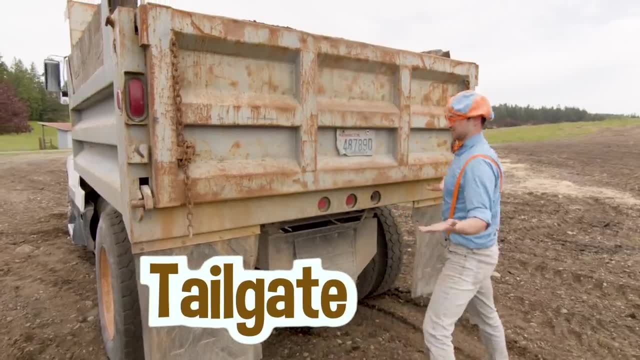 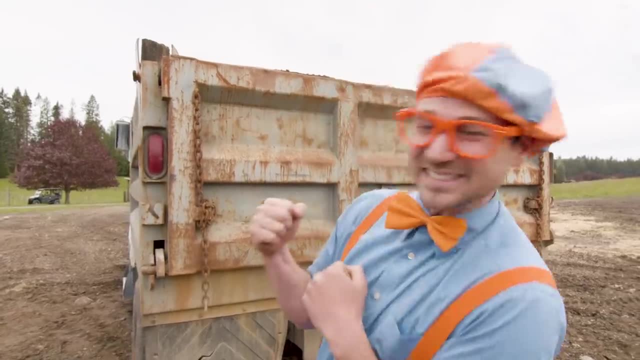 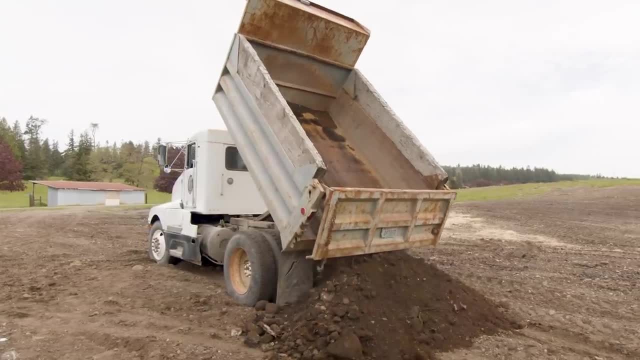 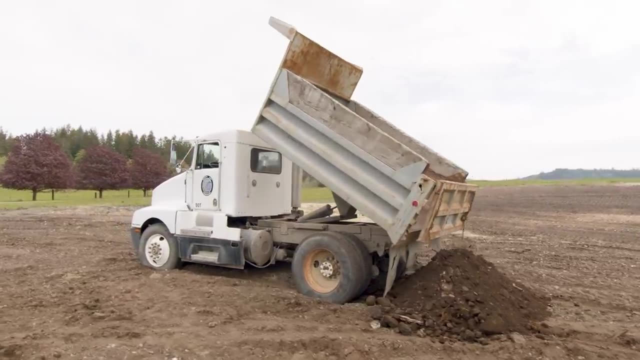 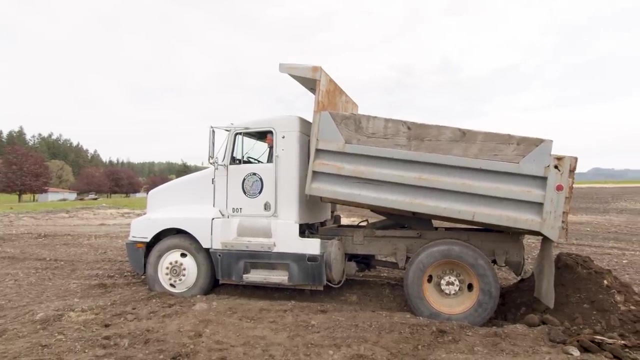 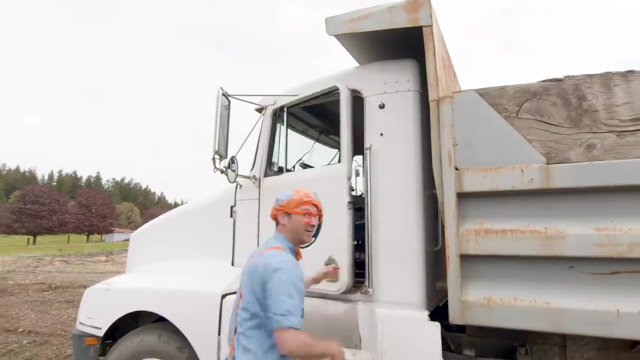 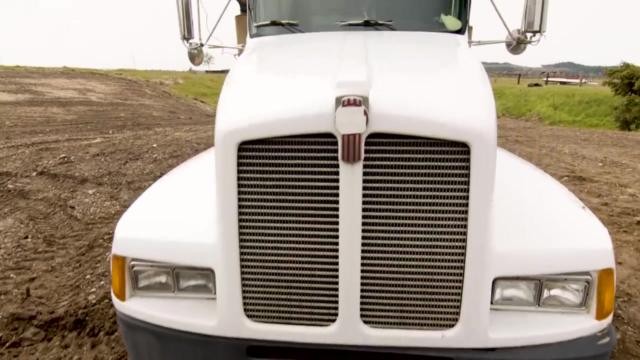 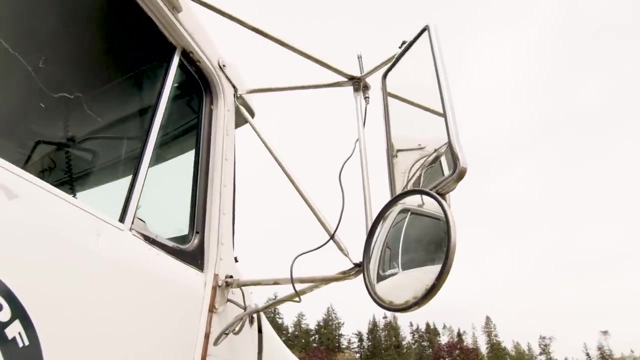 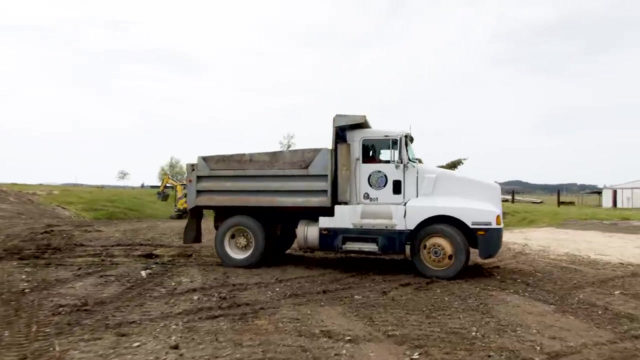 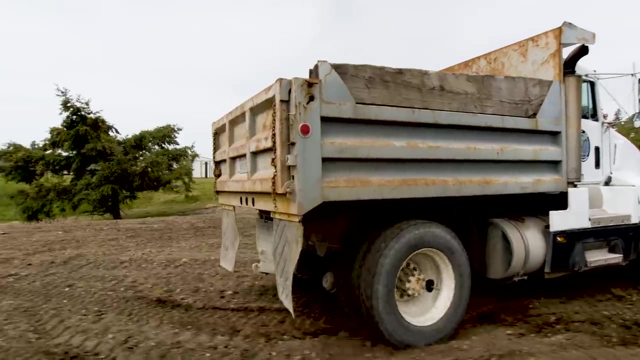 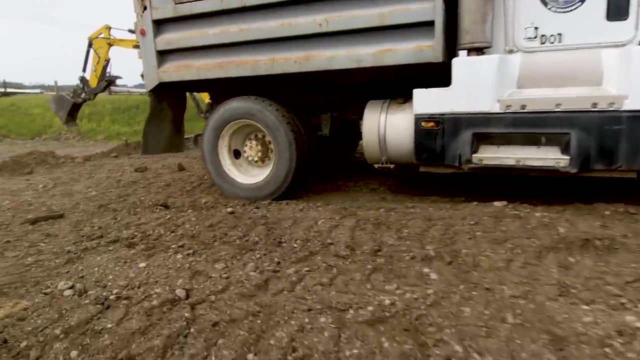 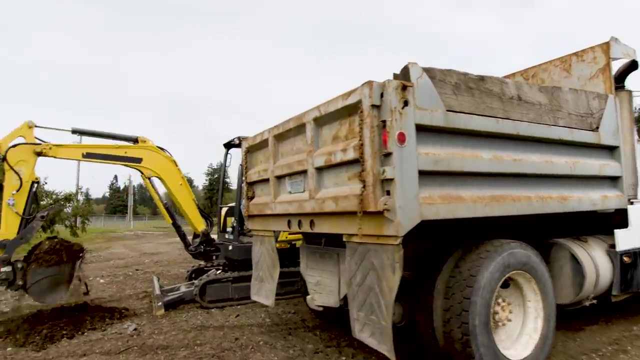 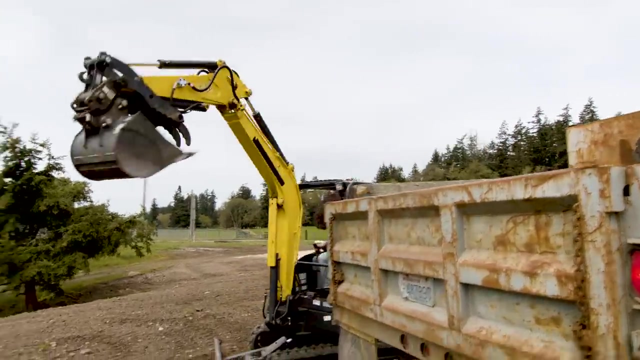 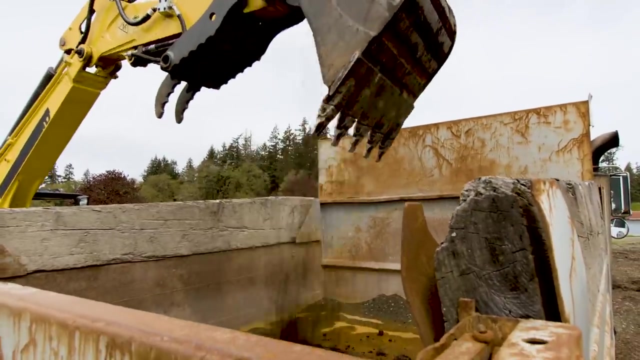 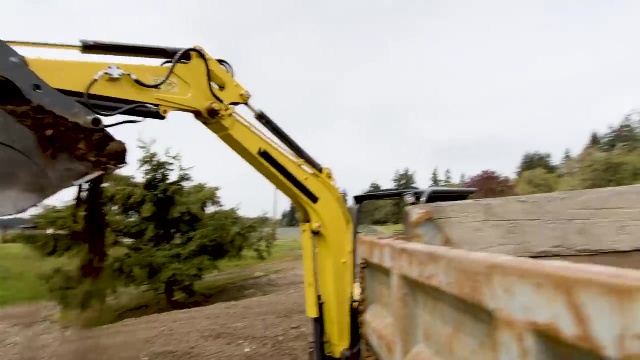 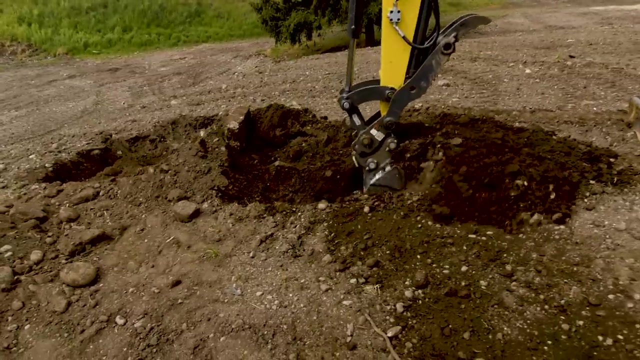 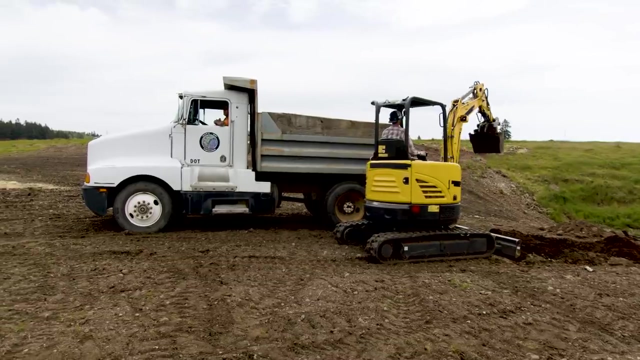 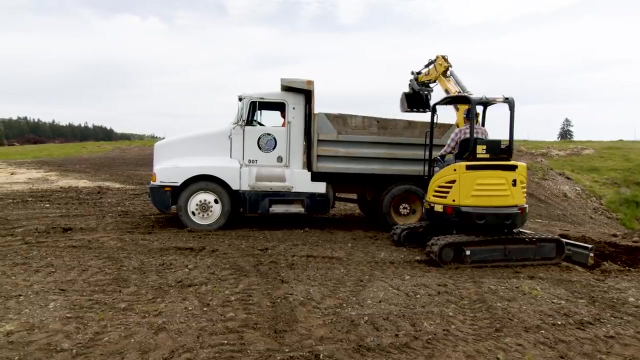 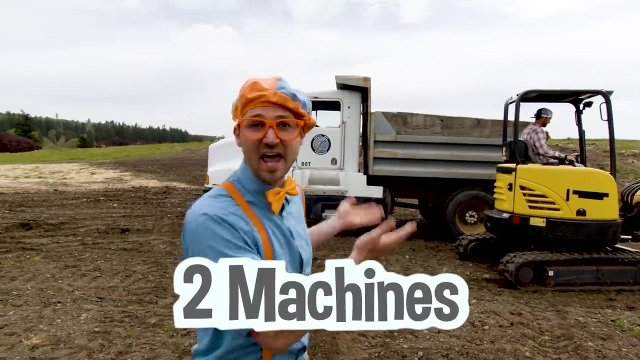 Let's go Now. that was awesome. Yeah, Yeah, Yeah, Yeah, Yeah, Yeah, Thank you. Thank you, Whoa, check it out. Do you see these two machines? Yeah, the excavator is loading up the dump truck. 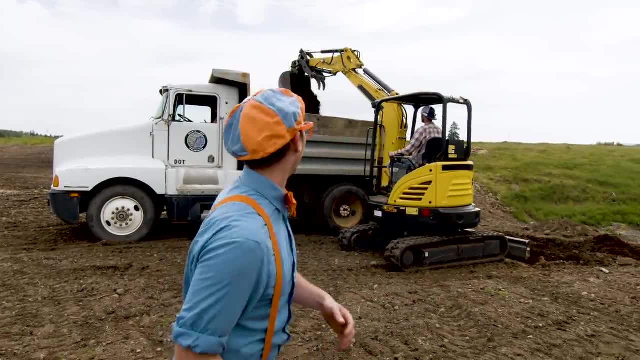 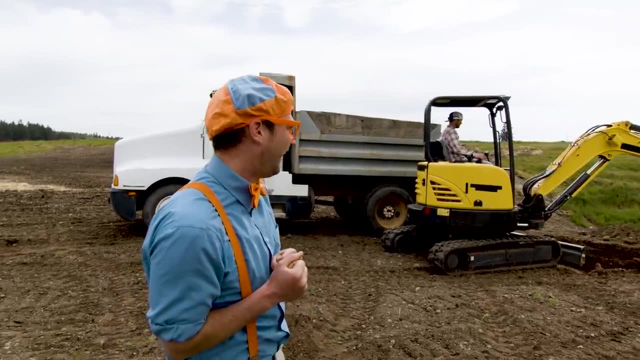 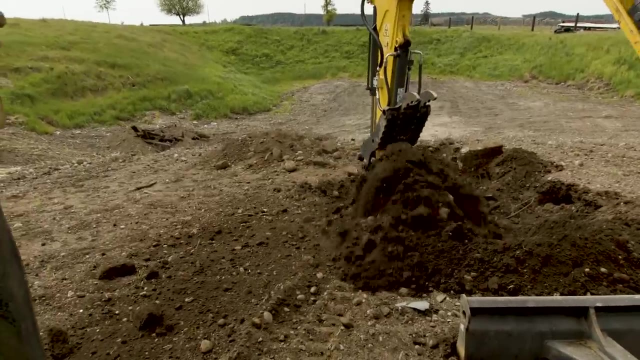 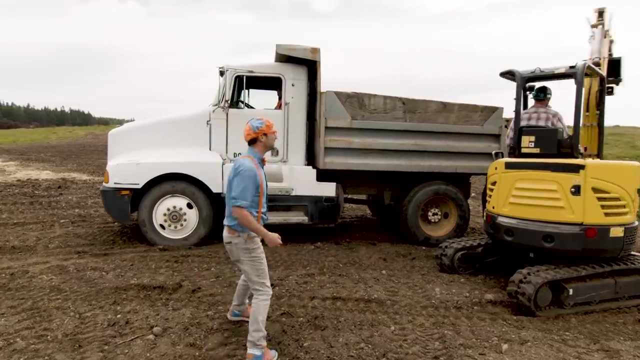 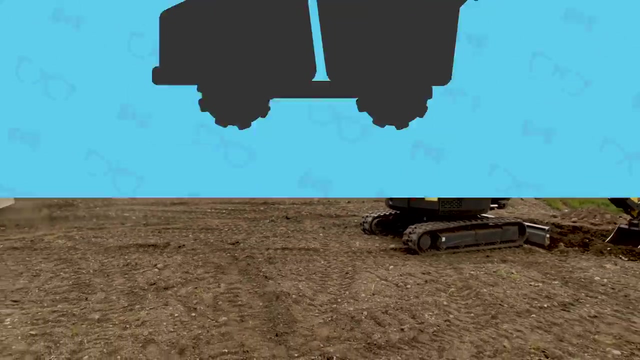 Wow, What great teamwork. Whoa, Those are some big scoops. that excavator is putting in that dump truck. Whoa, Wow, It looks nice and full. Woo-hoo, Woo-hoo. I sure do love dump trucks. 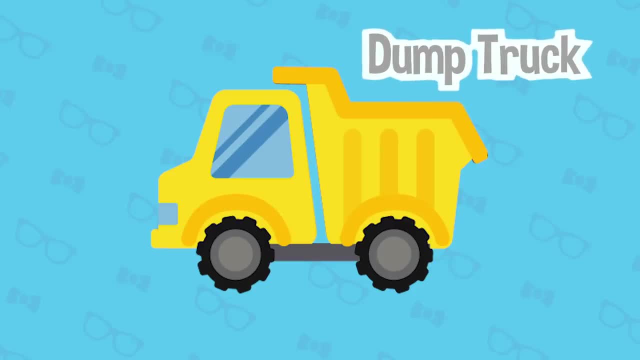 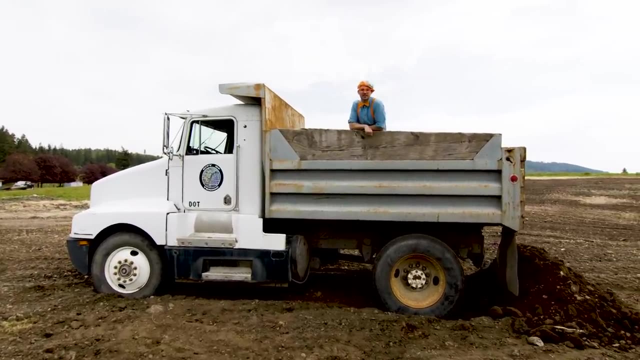 They're so tall, so powerful and so useful on the job site- Woo-hoo. Well, this is the end of this video, But if you want to watch more of my videos, all you have to do is search for my name. 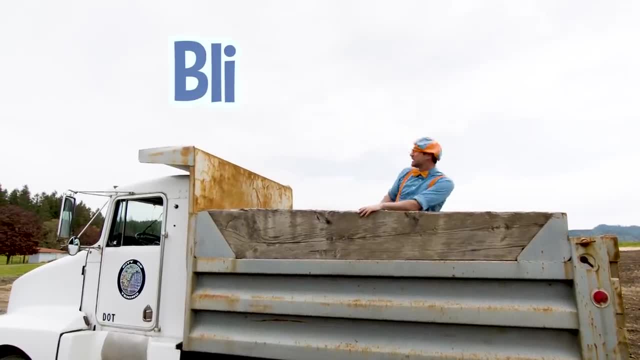 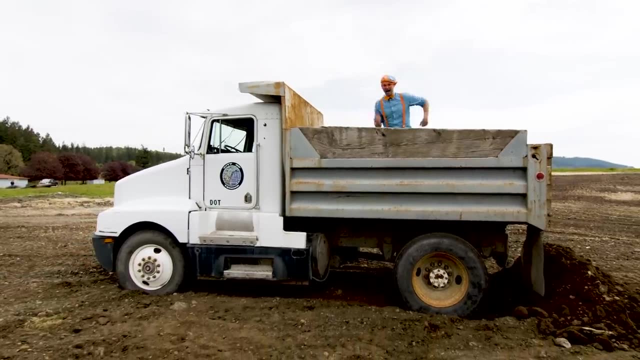 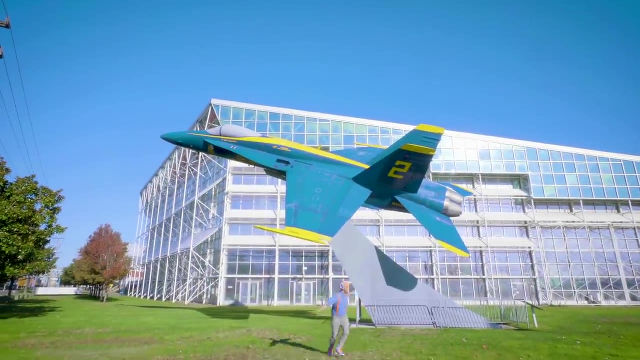 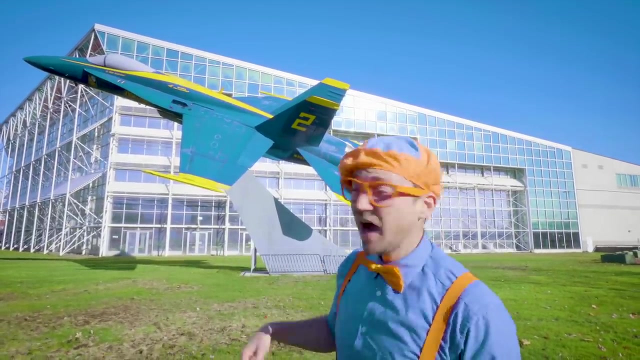 Will you spell my name with me: B-L-I-P-P-I, Flippy. Good job, All right, See you later. Bye-bye, Hey, it's me Blippy. And look at what's behind me. Whoa, a blue and yellow airplane. 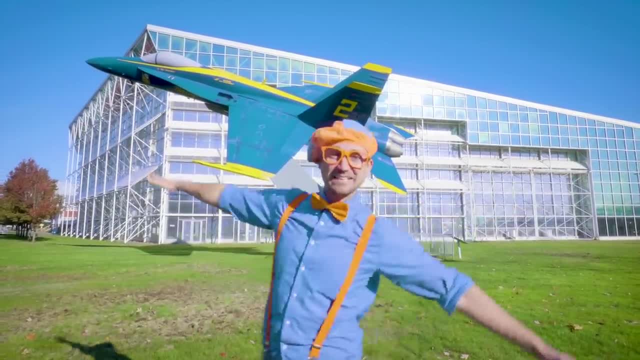 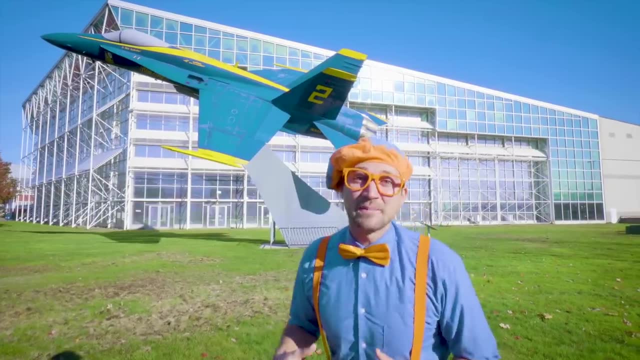 Yeah, Did you see how I was acting like an airplane? Woo-hoo, I sure do love airplanes, But hey, today I'm at the Museum of Flight in Seattle Washington, And today you and I are going to learn about airplanes. 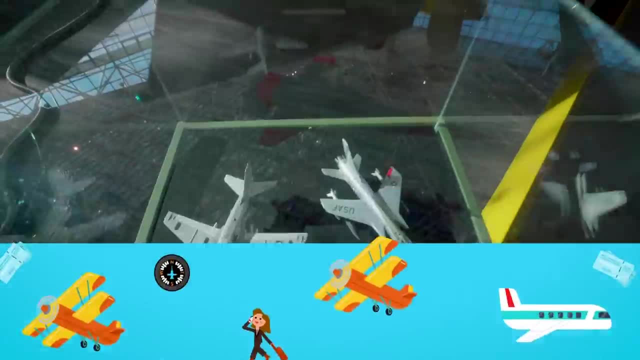 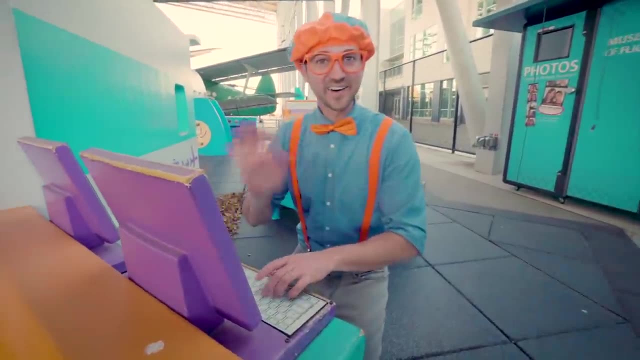 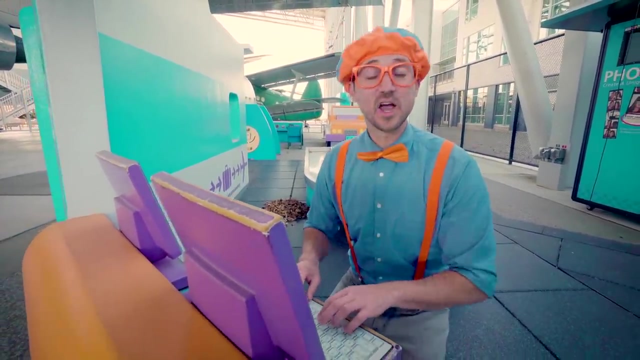 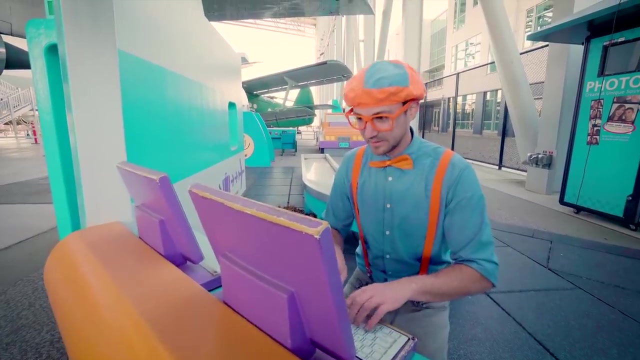 Yeah, Let's go. Oh hello, Welcome to Blippy Airlines. Where are you heading today? Wow, That sounds like a great destination. Is it for business or pleasure? Awesome, All right. Uh, let's see You are all checked in. 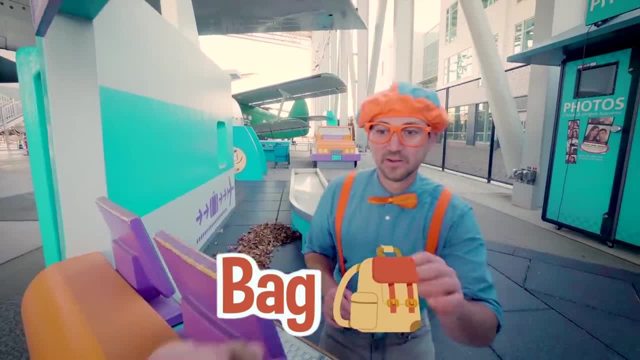 Do you have a bag? Ha-ha Okay, Perfect, Ooh, Thank you, Ha-ha Okay, Let's put the bag on the scale. All right, Looks like you're within the limitations, So let me put this on the conveyor belt. 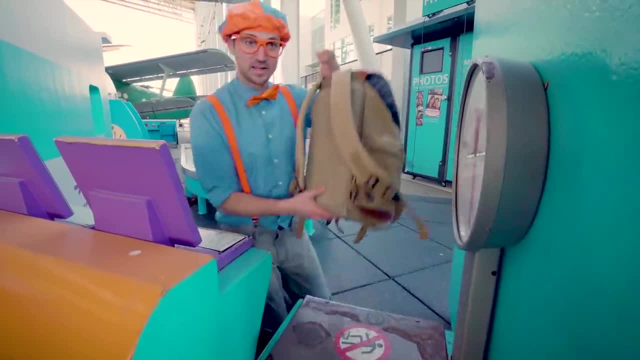 Okay, Well, have a great flight, But wait a second. That sounds like so much fun, Do you mind if I come? Ha-ha, Perfect, All right, Ha-ha, There we go. Now I have a ticket. 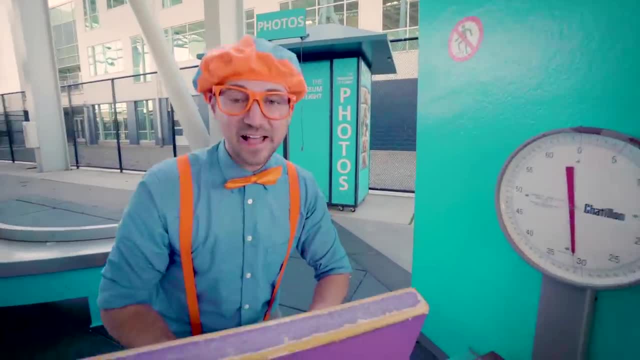 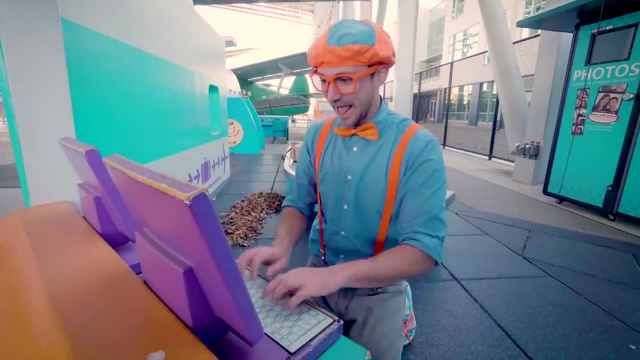 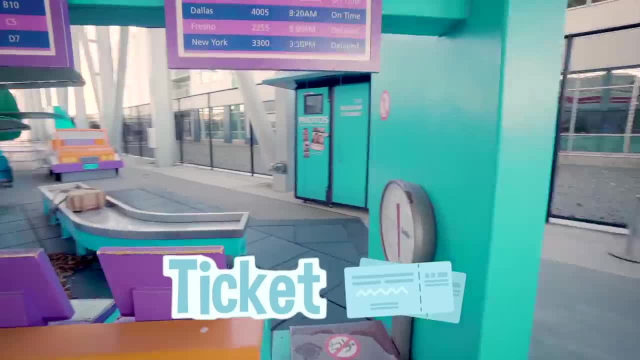 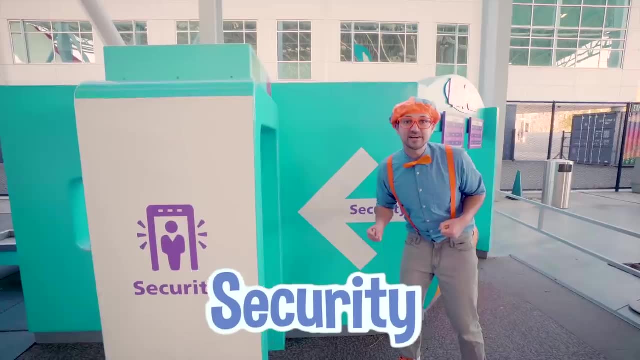 Now I have a ticket too. Okay, Let me come around. Whoa, Ha-ha, I am so excited for our trip together. Ha-ha, Hey, We have to go through security, All right, Ha-ha. 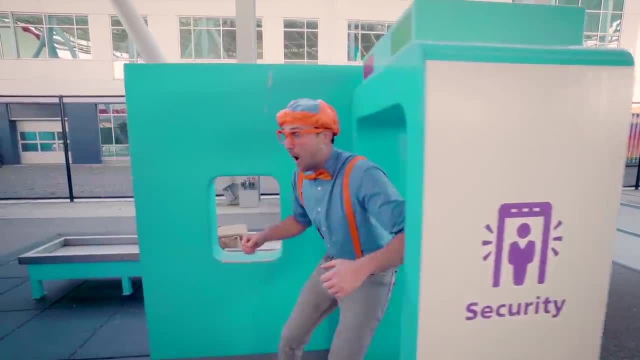 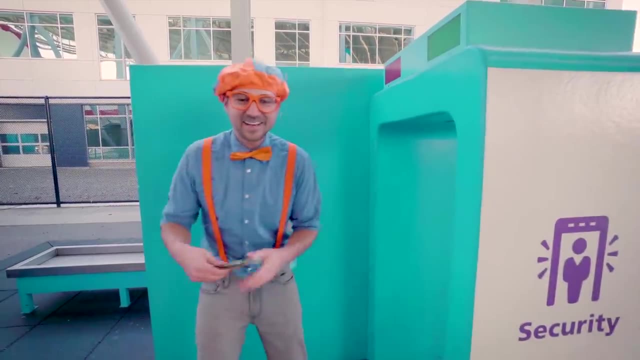 Oh, Did you hear that? Oh, That means, I must have something I shouldn't have on me. Oh, I know what it is. It's just my cell phone. Ha-ha, Oh, Oh, Oh, I know what it is. 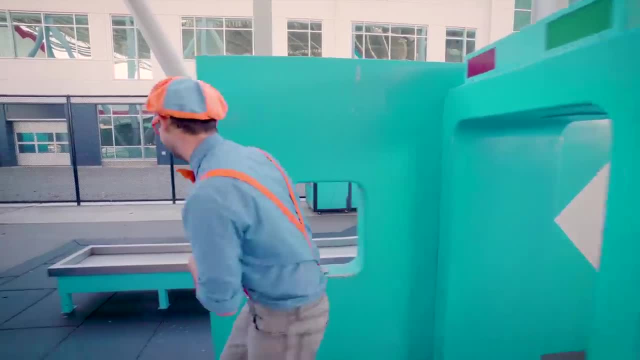 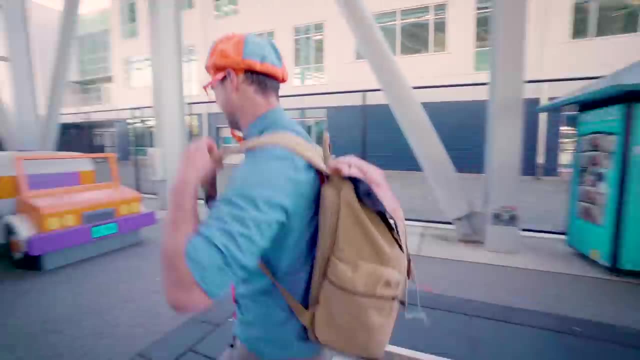 It's just my cell phone. Oh, I know what it is. All right, I'll put that there. Ha-ha, Come on. All right, Here we go. Ha-ha, Perfect, Let's go. Wow, Look at the airplane. 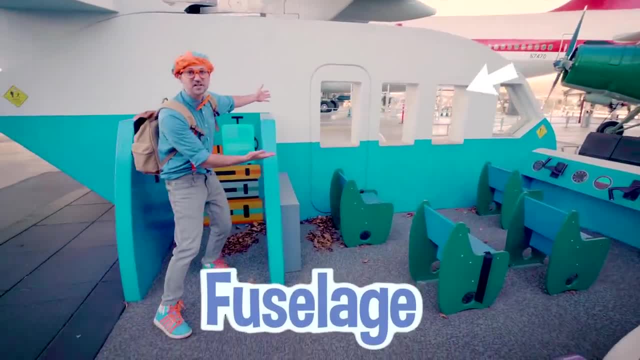 Whoa, Look at the fuselage, The cabin, And look at the tail up there. Whoa, This is going to be such a fun flight. All right, Let me put your bag down right here. There you go, bag. 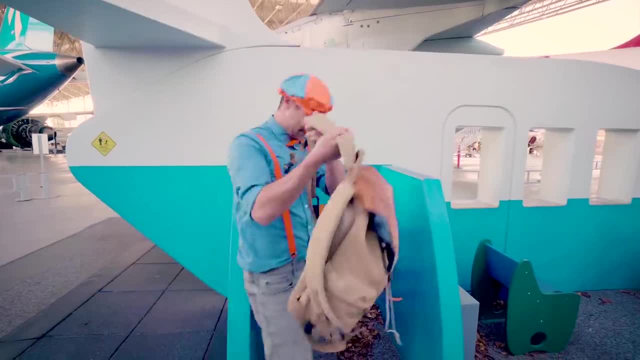 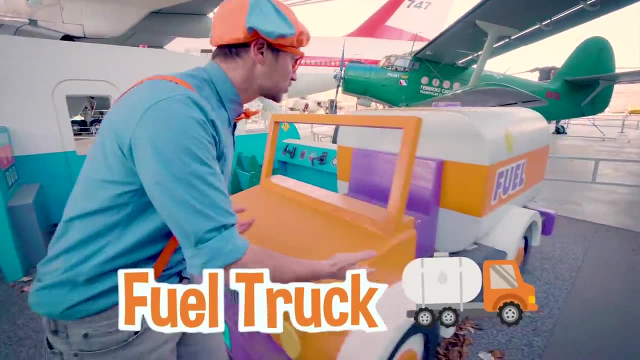 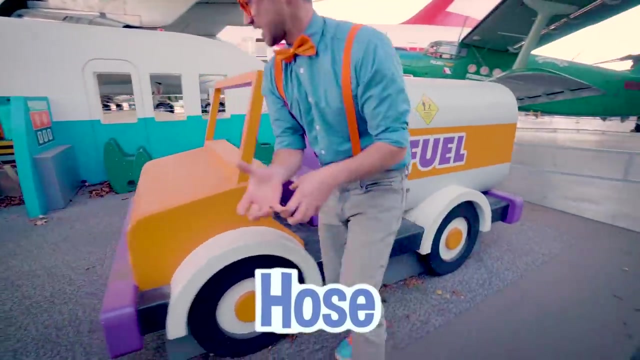 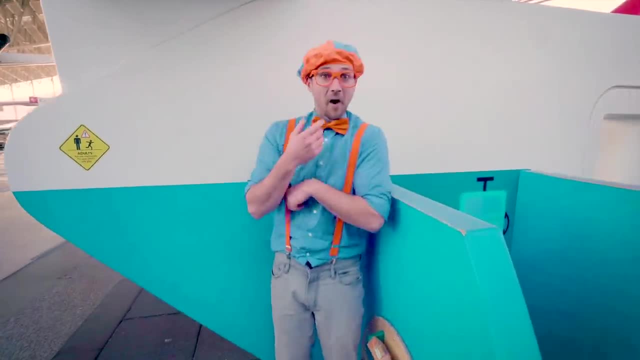 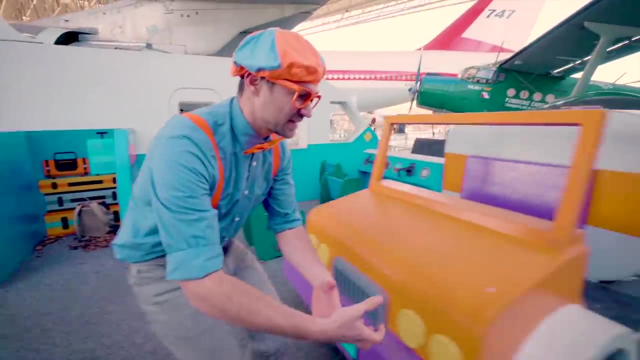 Here we go, Let's connect it. Oh Perfect, It's full. All right, Here we go. Okay, Now that the aircraft has a lot of fuel, now we can buckle up. Okay, First thing we're going to do is we're going to get the fuel. 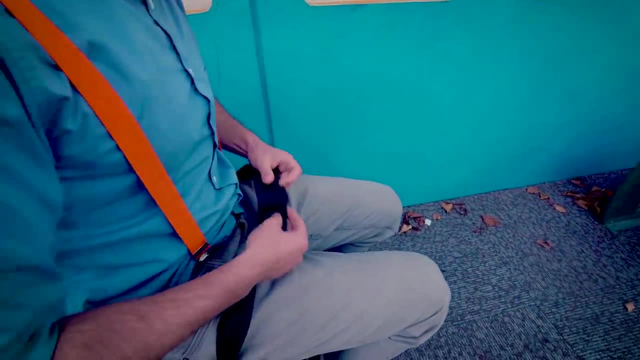 First, let's put on our seatbelt. There we go. Okay, Now we'll listen for instructions for the flight Ha-ha. Thank you for choosing Blippi Airlines. Please mind the aisles and be sure to find the nearest emergency exit. 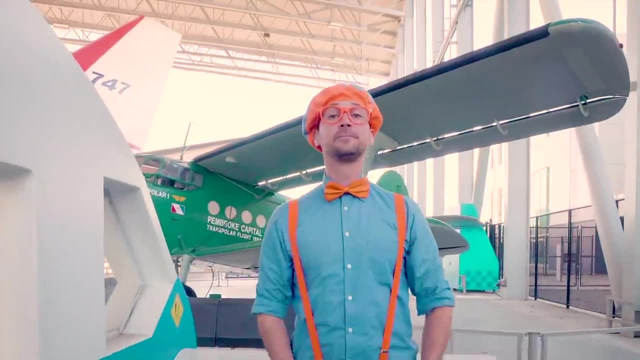 Buckle your seatbelt and make sure it's nice and tight And in case you need an air mask, it will come down from above. All right. Now that we've got the safety briefing and passengers are seated, now we can get on the. 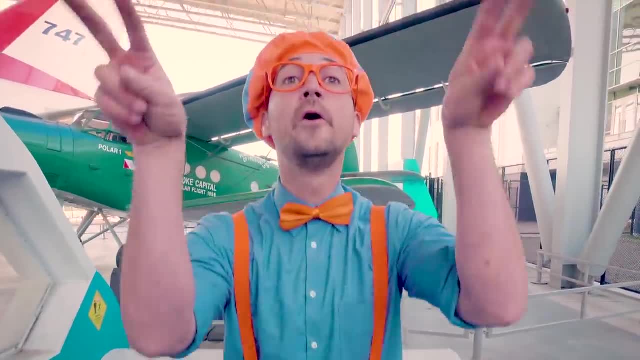 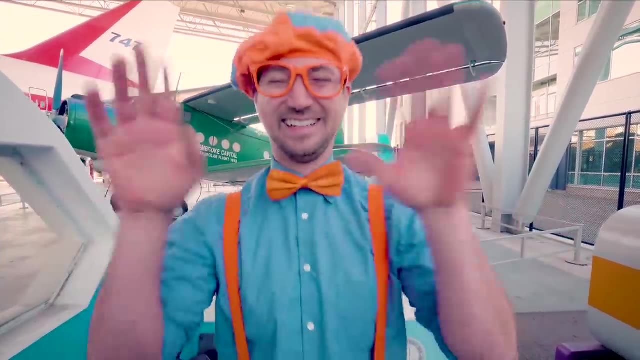 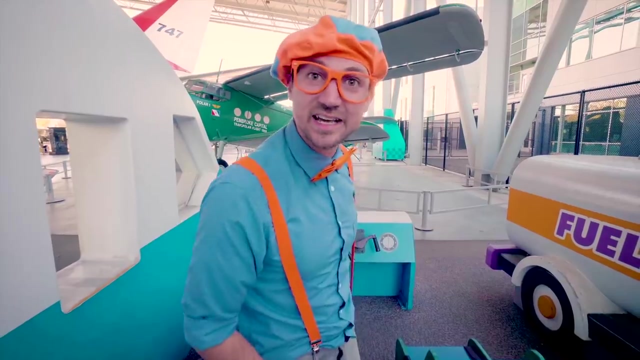 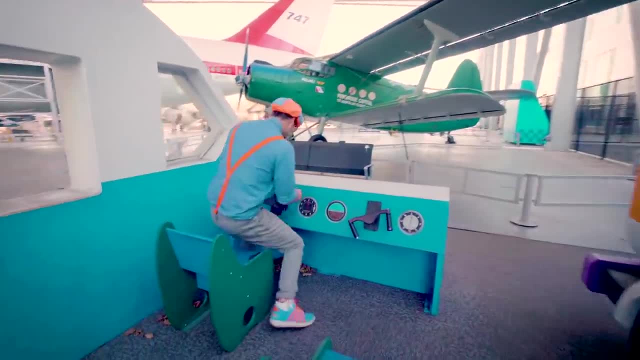 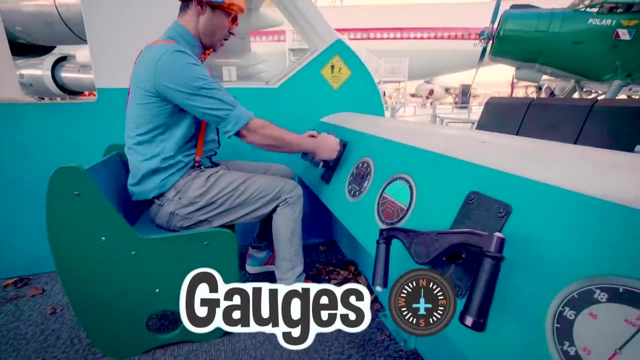 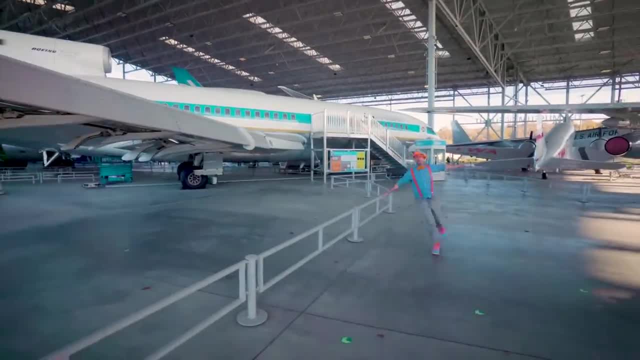 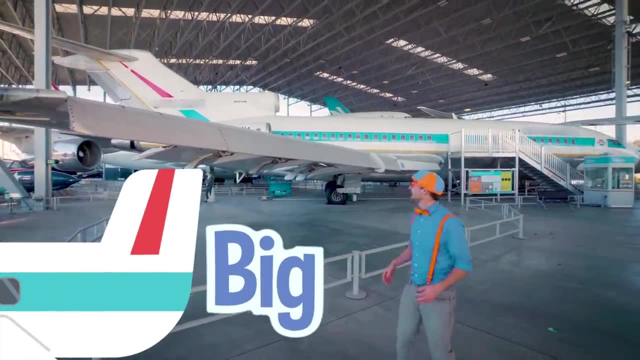 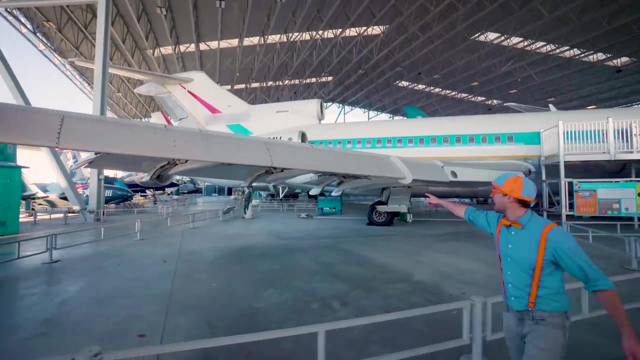 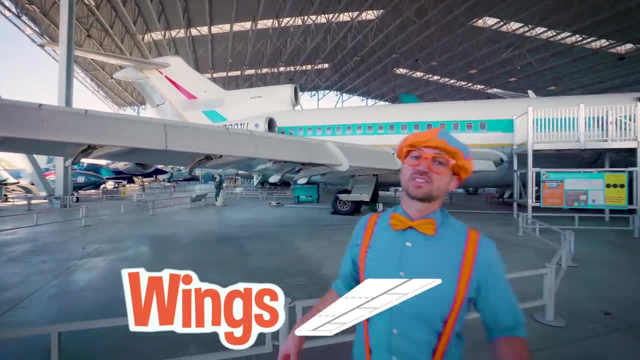 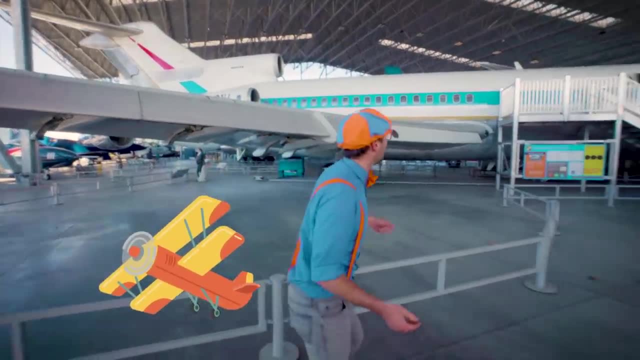 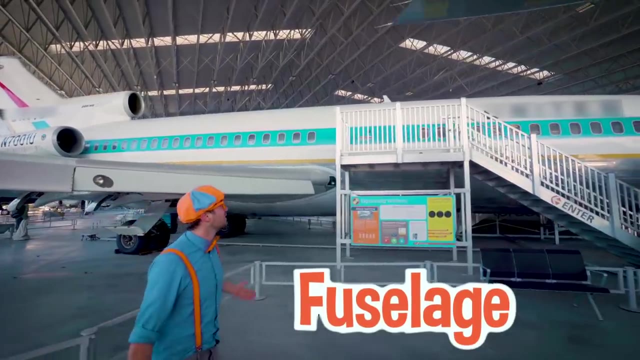 These are called wings. Most airplanes have two wings that go from the side, but not all of them. Some have more Whoa and look at this. See, the main body of the airplane is called the fuselage. Wow, This airplane is actually used to put people inside. 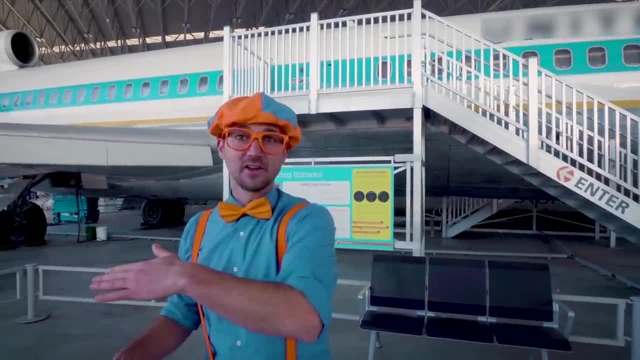 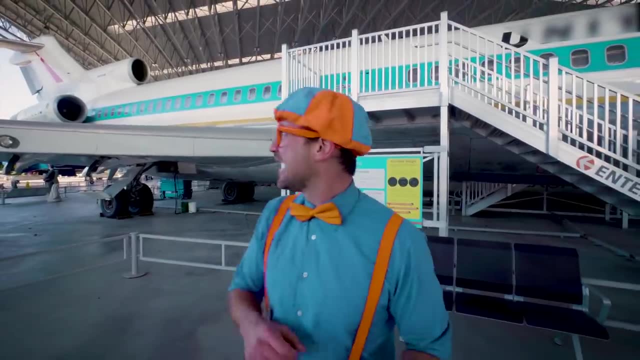 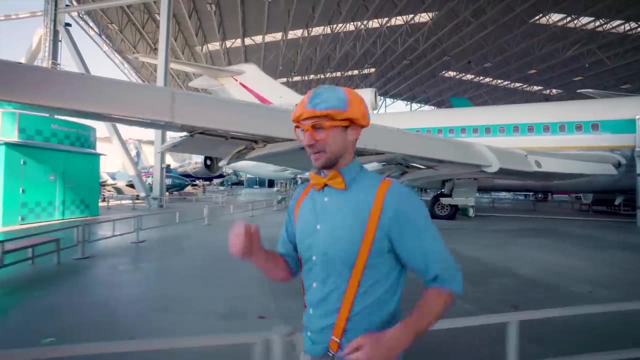 and transport them from one location to the other location, just like, say, a car or a boat or a bicycle, but way quicker. But hey, remember how I said: this airplane is so big. Here, come follow me and I have another airplane for you. 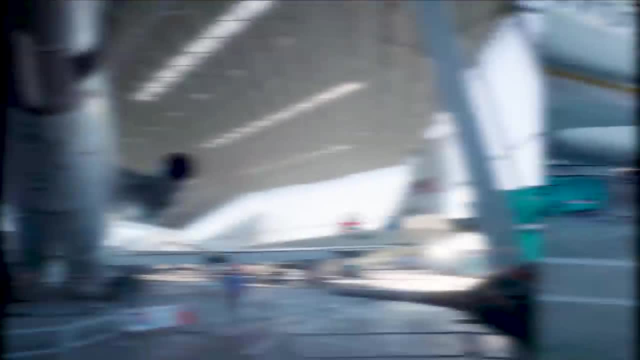 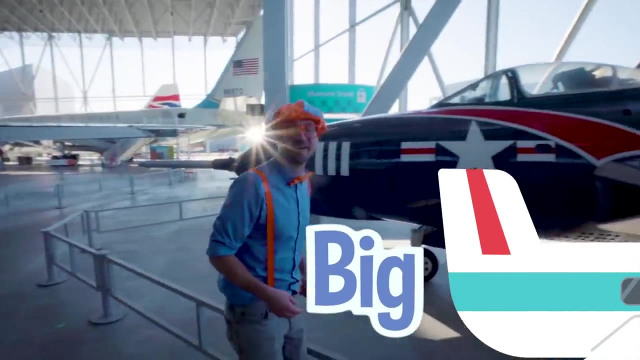 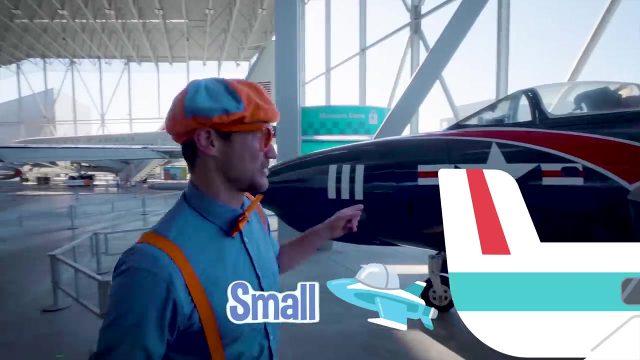 And it is not very big. Remember how I said, that plane is really big. Check this one out. Whoa, Yeah, this plane is small. Well, it's smaller compared to that plane, but I'm sure there's smaller airplanes than that one. 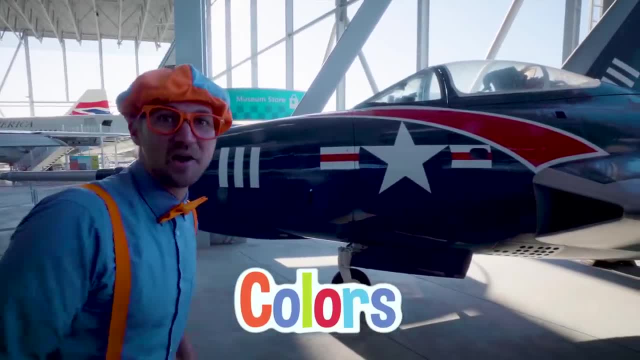 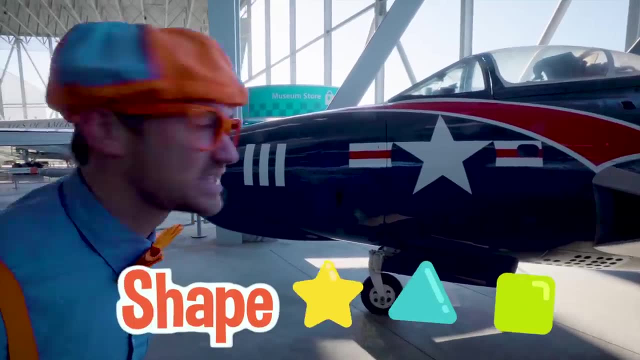 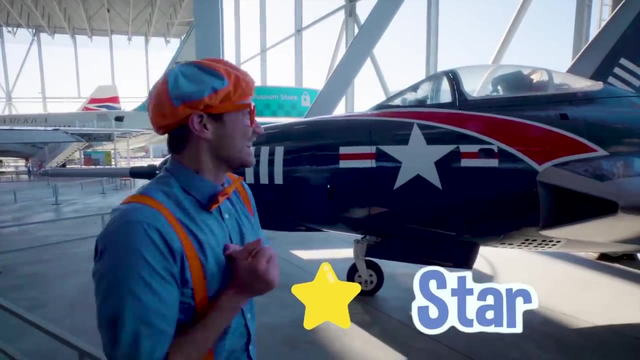 But hey, what colors do you see on it? Yeah, red, white and blue. Yeah, woo-hoo. And what shape is that? Oh yeah, that looks like a star. Whoa, this plane looks like it goes so fast. 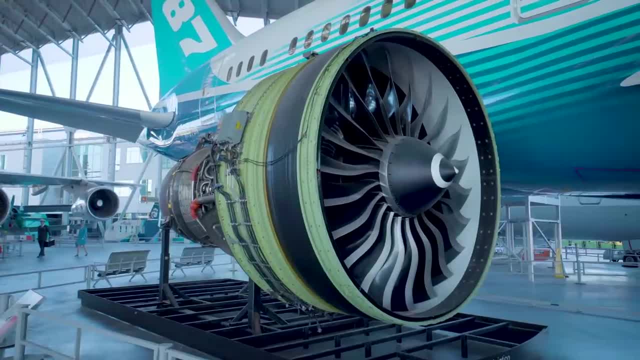 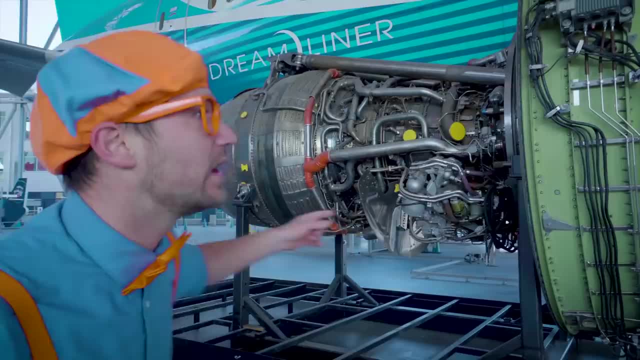 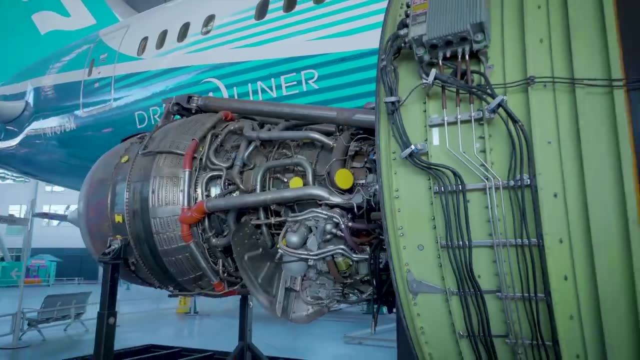 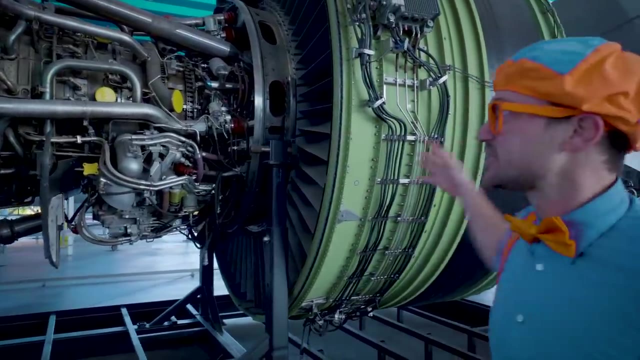 Yeah, but there's no outside casing around it. Whoa, it is so big. Look how big it is compared to me. Do you see everything in there? There's so many hoses and tubes and oh geez. So the air goes in right here, gets compressed. 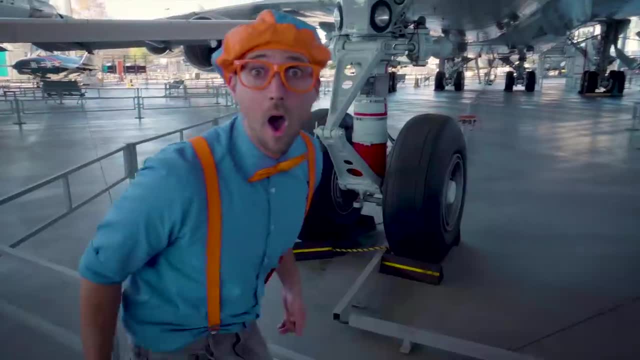 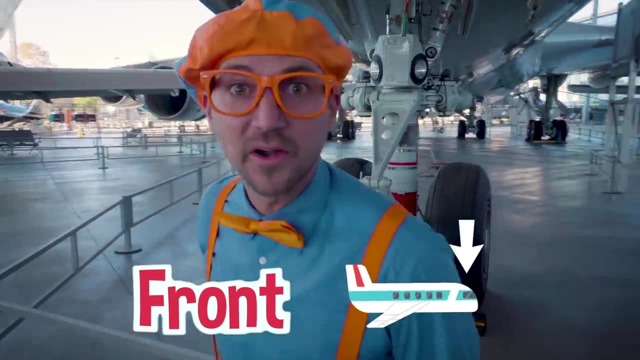 fire and then boom, Whoa, Whoa, these tires are so big And there's actually two tires right there. Yeah, we're at the front of the air craft, So let's head to the back of the aircraft and see how many tires are back here. 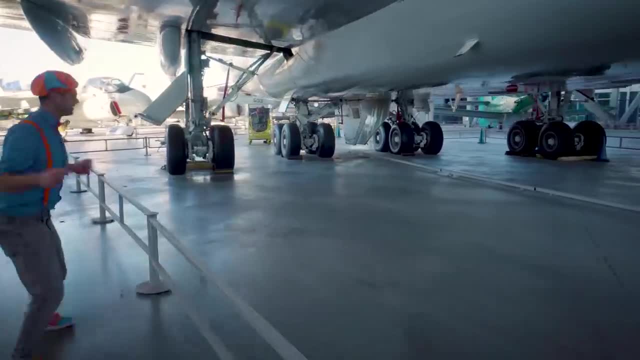 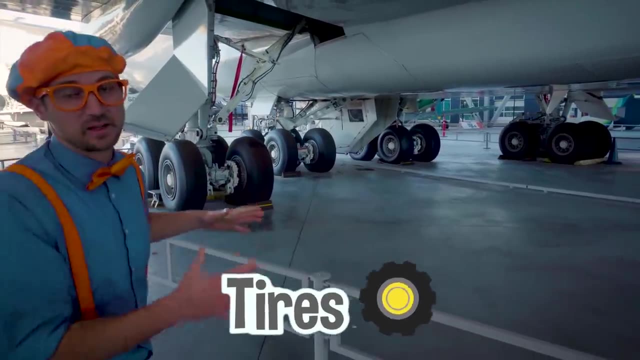 Whoa, do you see them? Wow, there's so many more tires back here. Wow, this plane must be really heavy. Yeah, that's probably why they have so many tires. Whoa, And look how big this wing is. 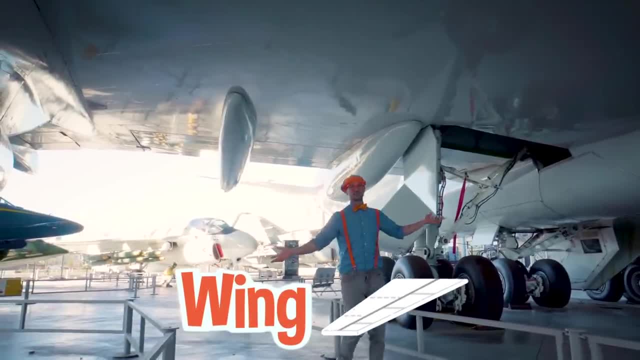 If it was raining, I definitely would not get wet. Whoa, check out this airplane. It looks like it goes really fast. Hey, what color of airplane is it? Yeah, you're right, It's blue With a little bit of yellow. 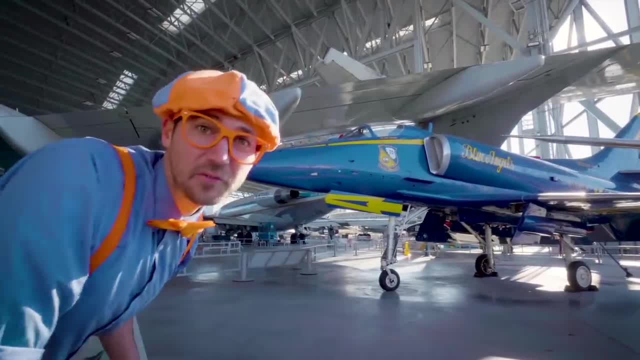 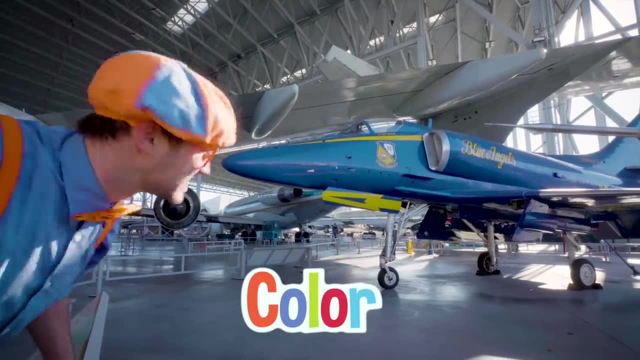 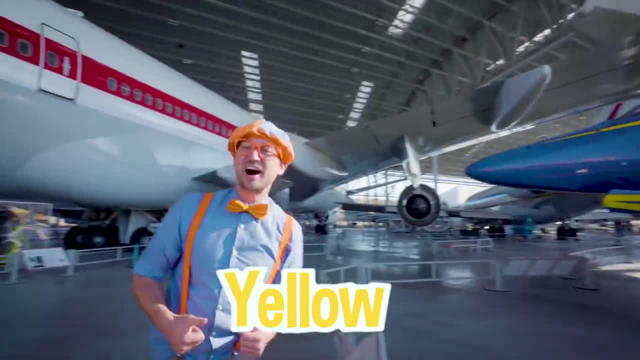 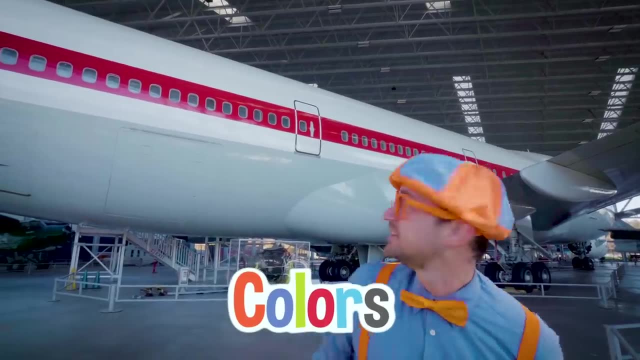 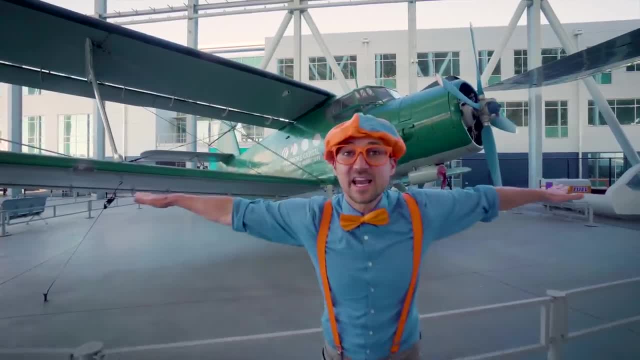 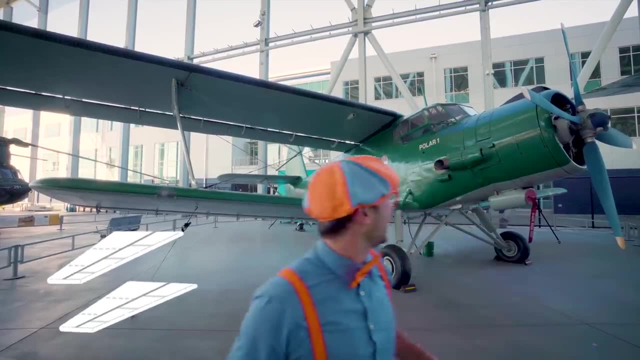 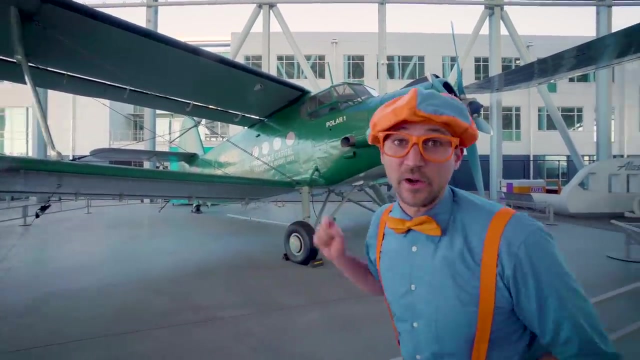 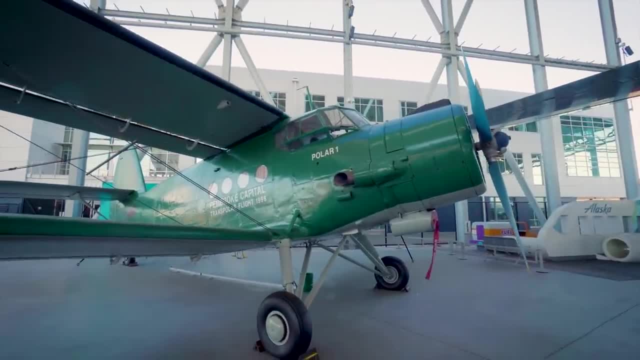 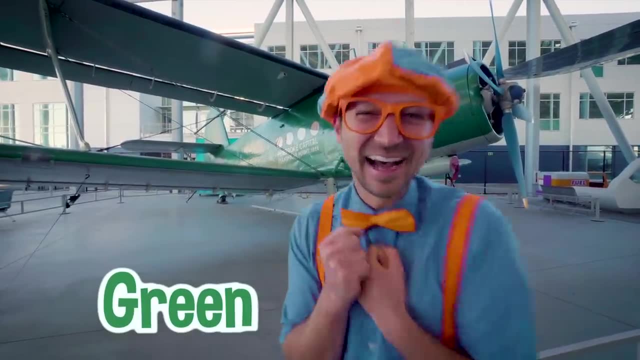 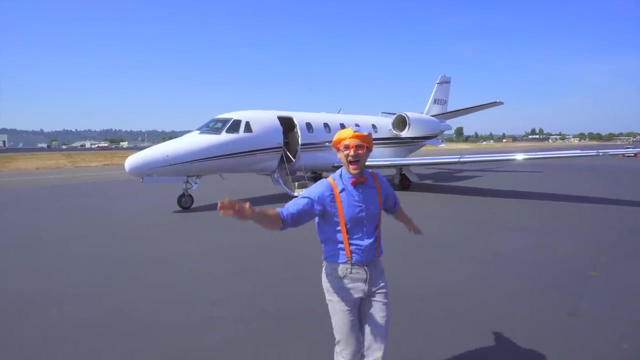 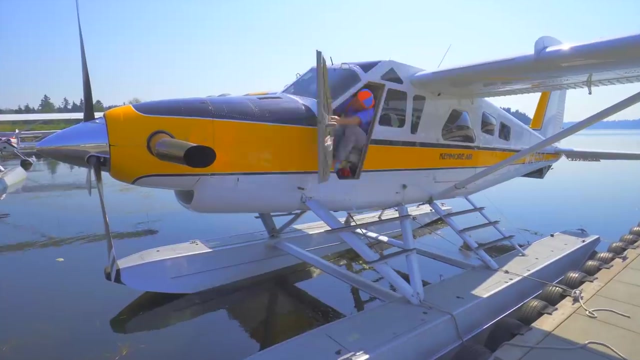 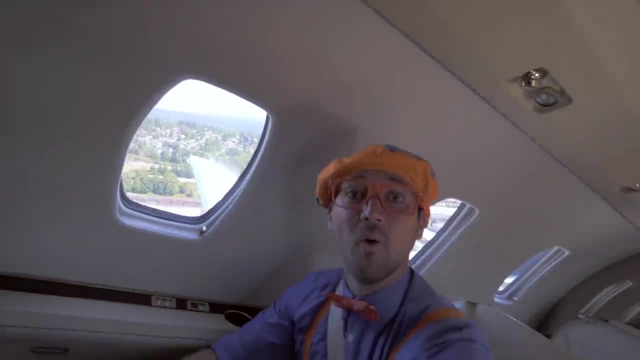 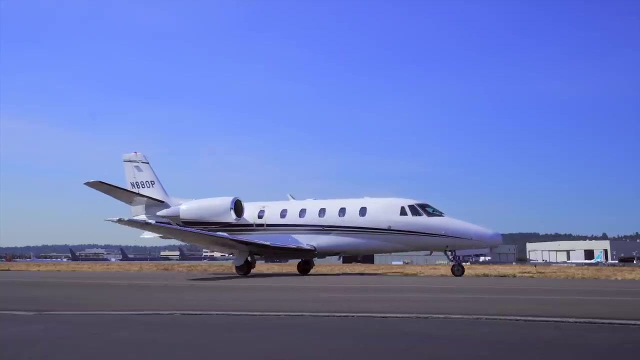 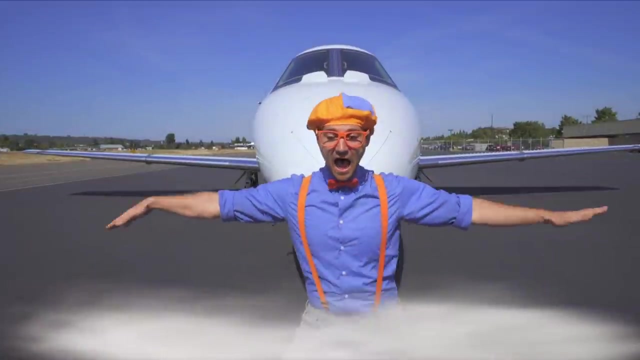 is this airplane? Yeah, you're right, You said green. Good job, All the people. they look like ants. when we're up with the birds On the airplane, the wings keep us gliding. We're on top of the world, So keep that worrying engine and look out. 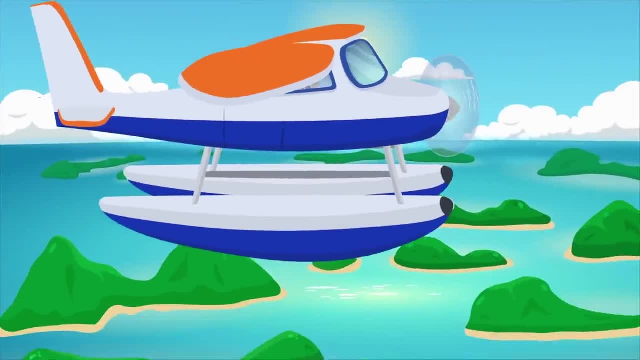 on the wing. We're gonna fly, fly, fly till we can touch the sky. We're gonna fly, fly, fly till we can touch the sky. We're gonna fly, fly, fly till we can touch the sky We're. 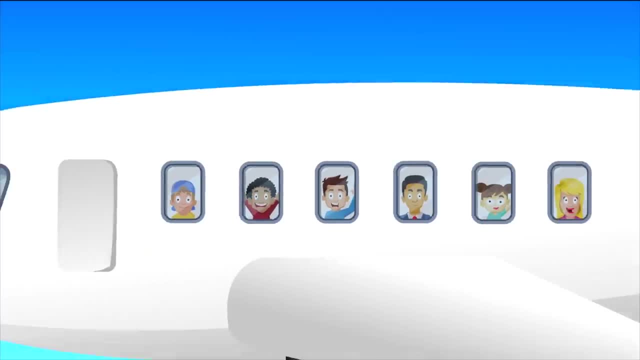 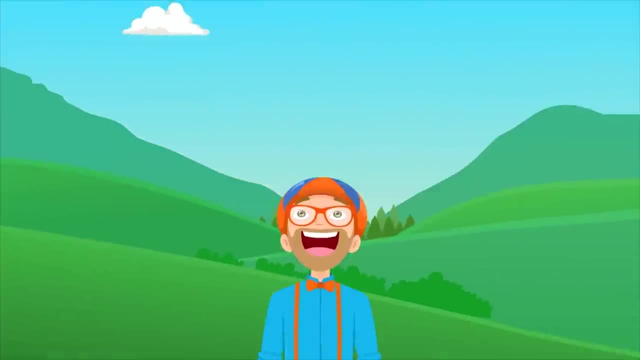 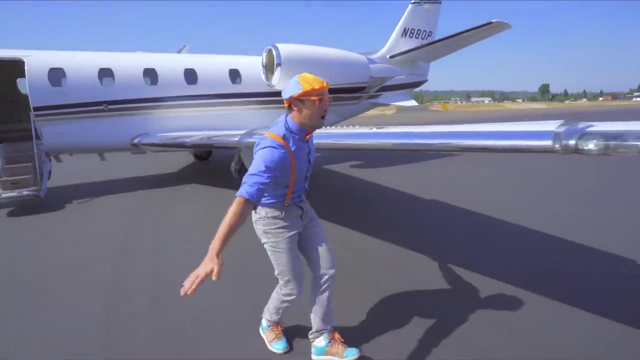 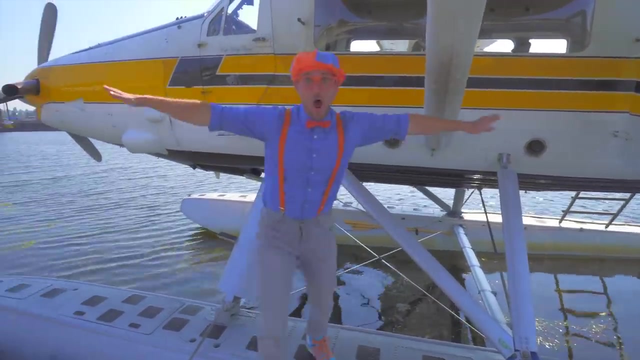 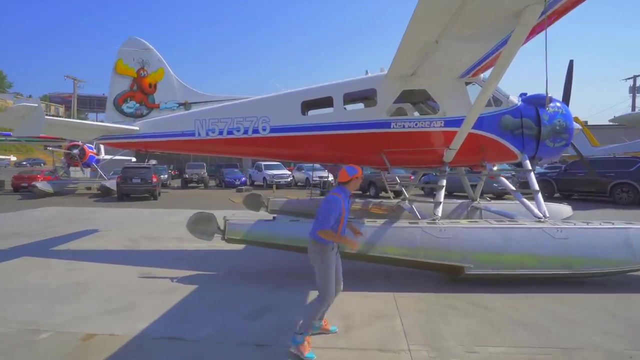 We're gonna soar right through the clouds. We're gonna fly, fly, fly. We're going way up high On the airplane in the sky. We're going to fly. Yeah, yeah, We're going to fly. Yeah, yeah. Get your passport, Get your luggage too. 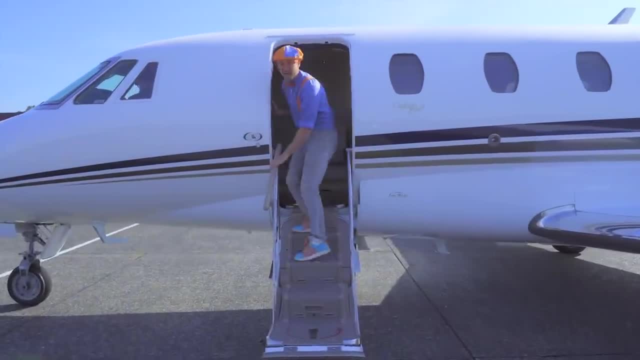 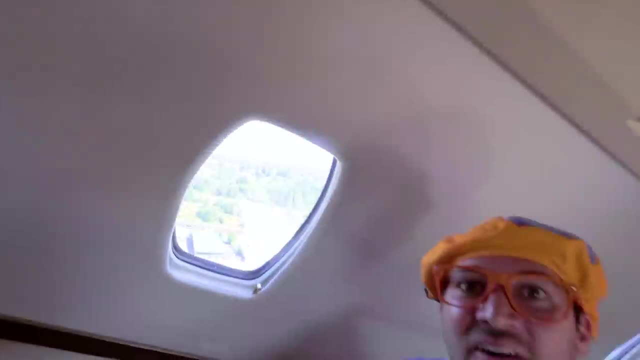 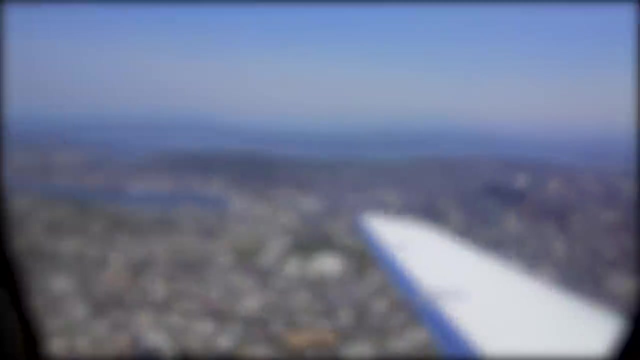 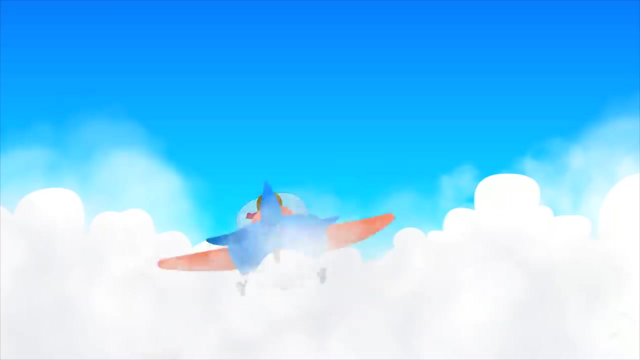 We're going on an adventure. Wear your seatbelt, Feel the plane taking off And take in the view. So keep that worrying engine Better look out on the wing. We're gonna fly, fly, fly Till we can touch the sky. We're gonna soar right through the clouds. 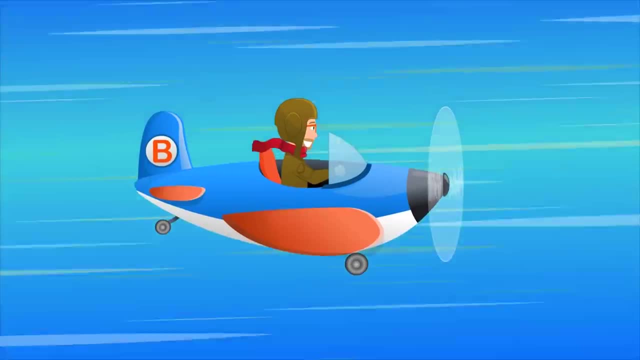 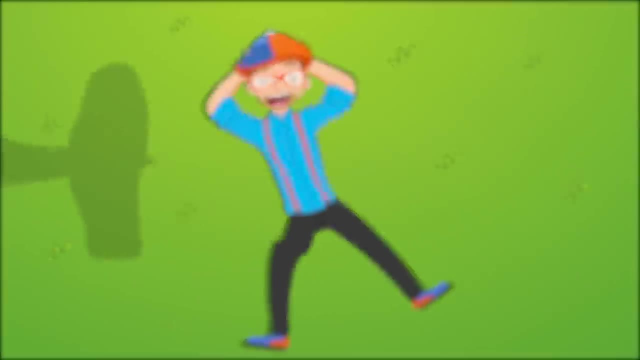 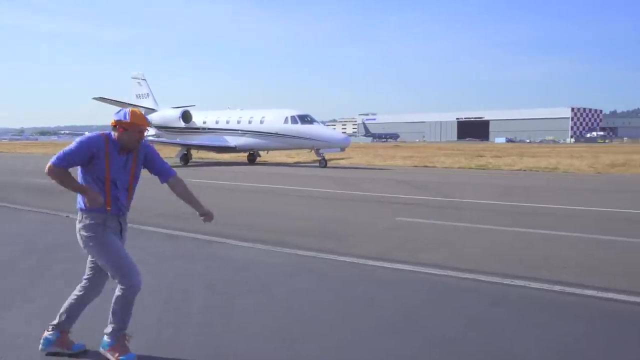 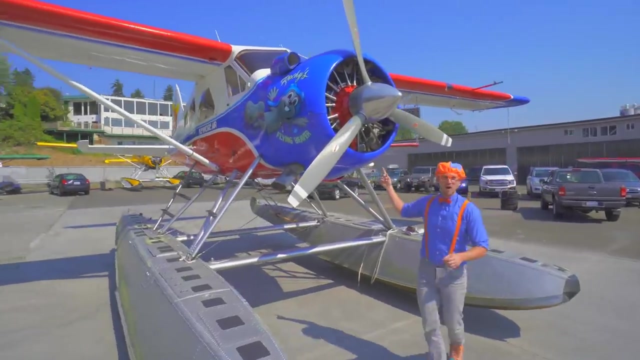 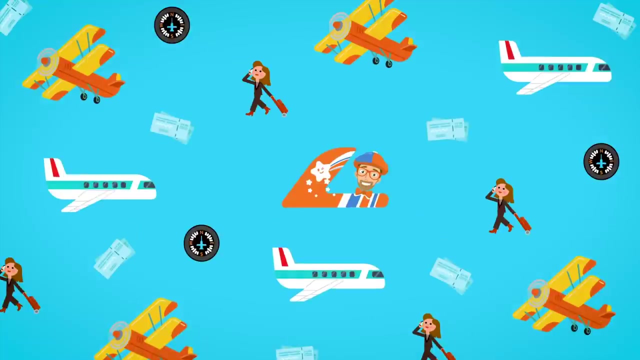 Yeah, yeah, We're gonna fly, fly, fly. We're going way up high On the airplane in the sky. We're going to fly. Yeah, yeah, We're going to fly. Yeah, yeah, We're going to fly. Yeah, yeah, We're going to fly. 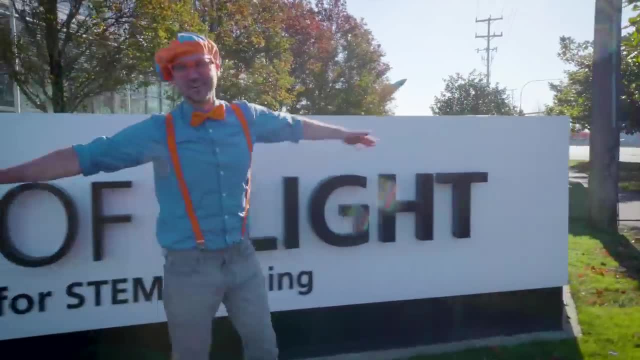 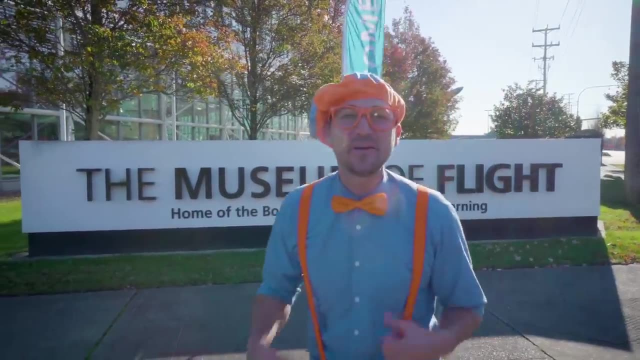 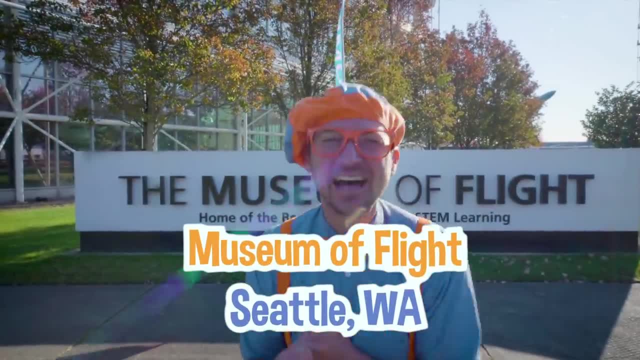 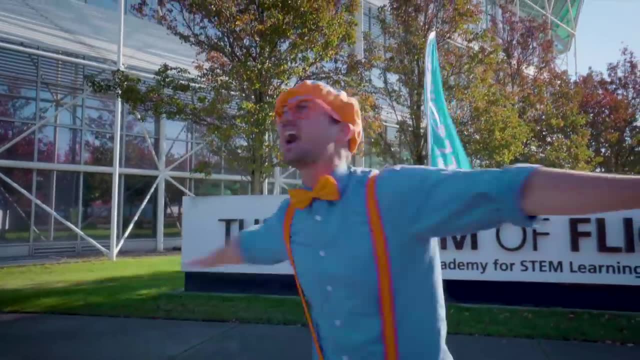 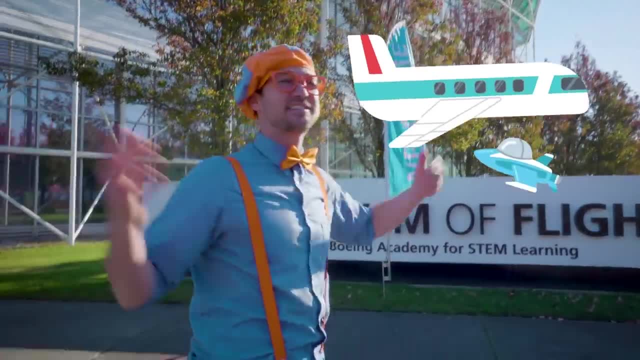 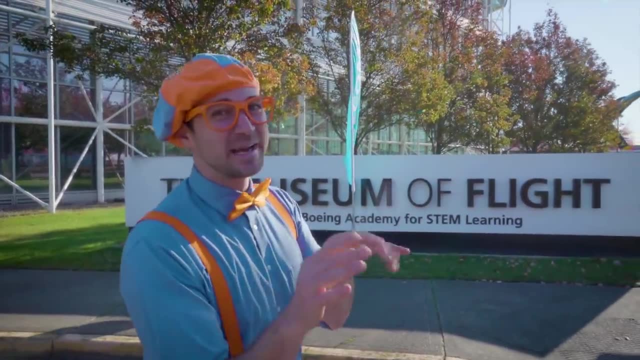 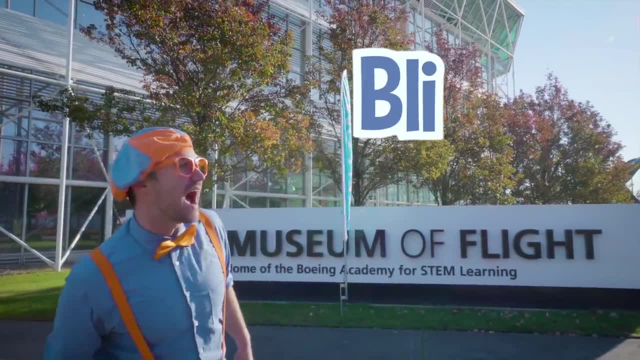 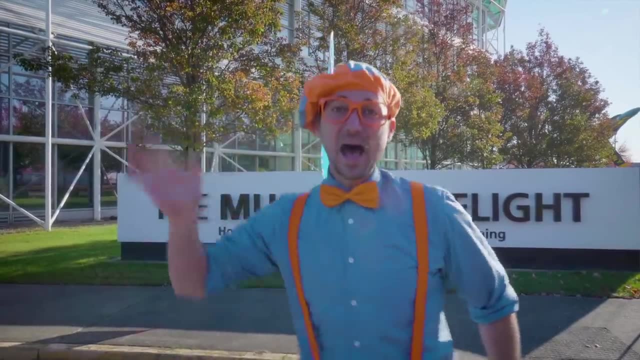 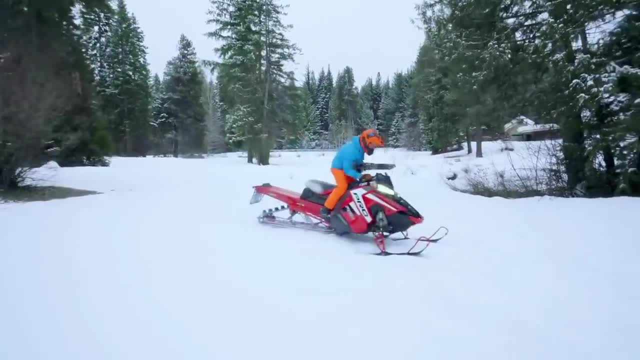 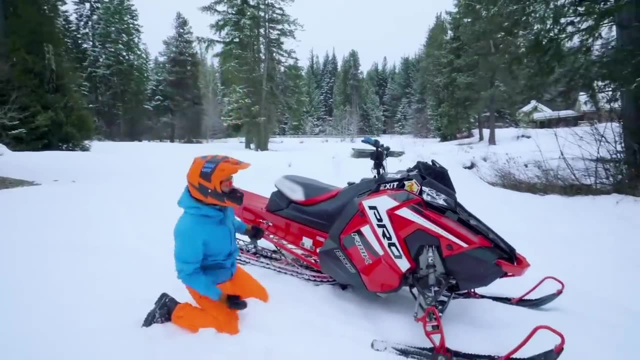 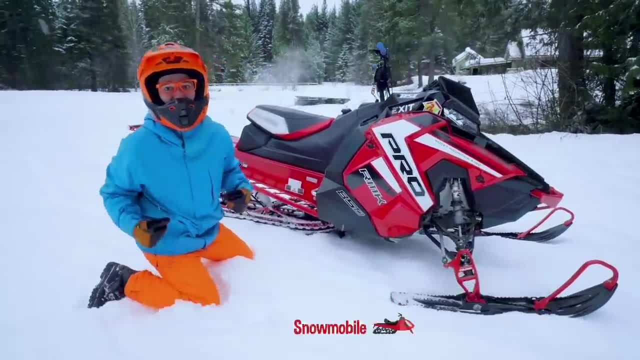 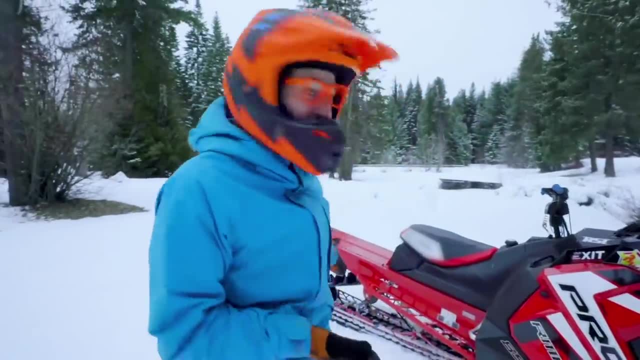 We're going to fly. Yeah, yeah, We're going to fly, Yeah, yeah. Hey, it's me, Blippi, And look at what's behind me. Whoa, This is a snow mobile, And this snow mobile belongs to my friends Magnus and Hans, And today you and I are going to learn about. 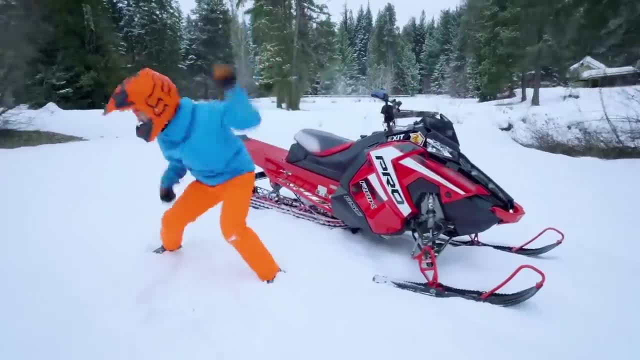 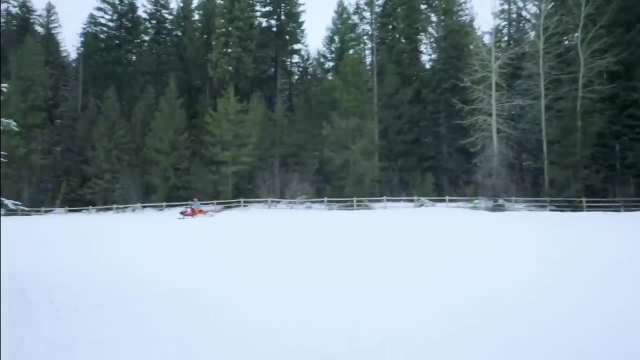 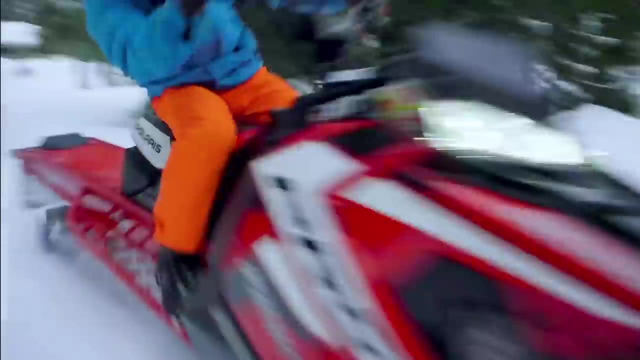 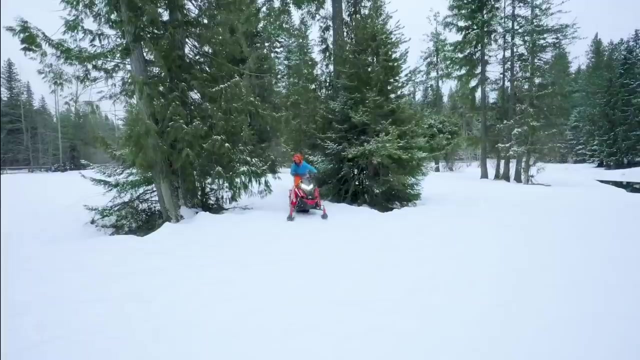 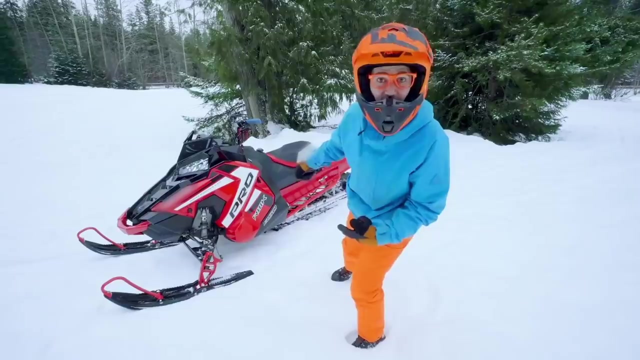 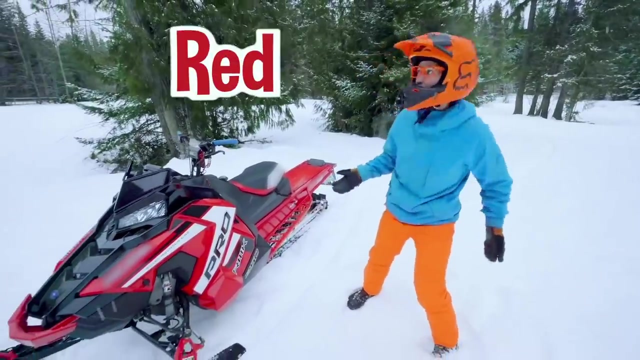 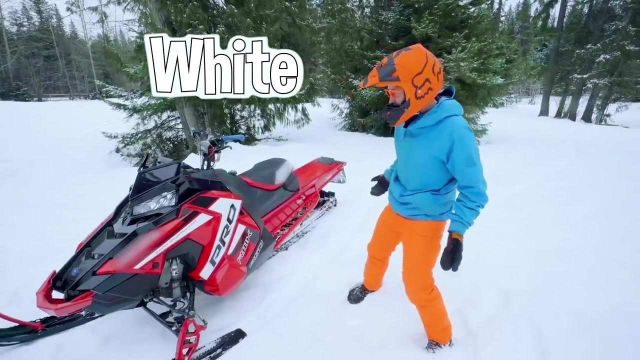 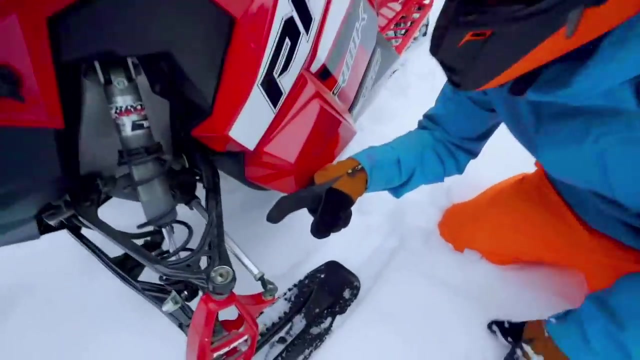 Snowmobiles- Yeah, Hey, I forgot to ask you what colors do you see on this snowmobile? Yeah, I see the color red, black, white and hey, look down here, there's some silver. Hey, come back here. 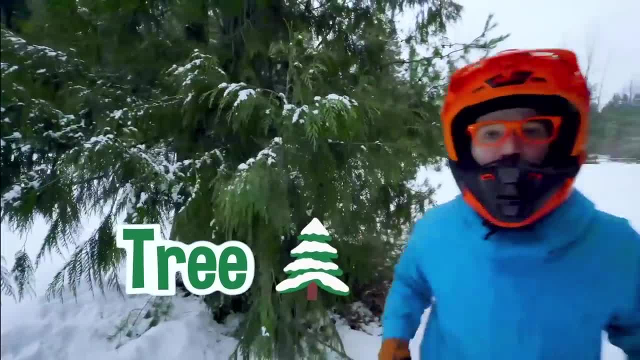 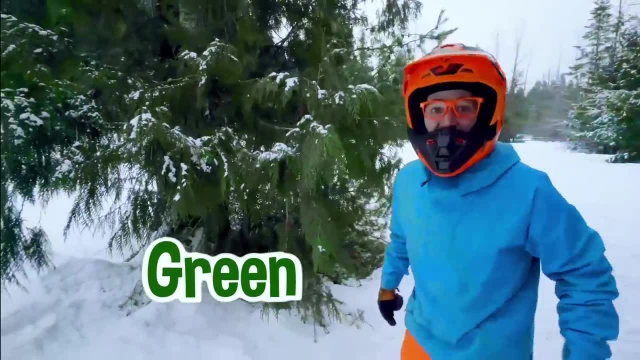 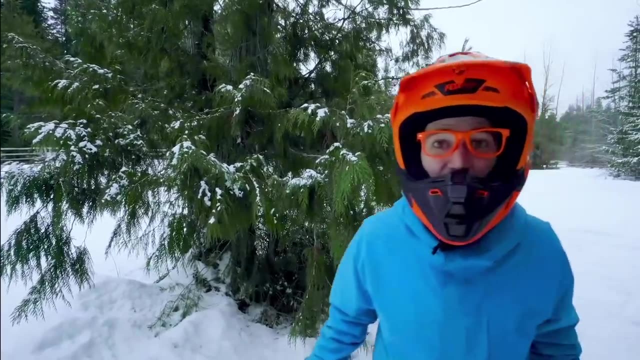 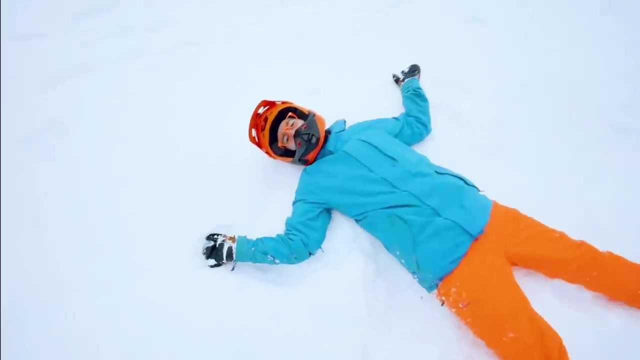 Whoa, look at this tree. What color is this tree Looks like icy, green and brown, and what else? Yeah, the snow is white. Let's go. I love playing in the snow, but it's so cold I know. 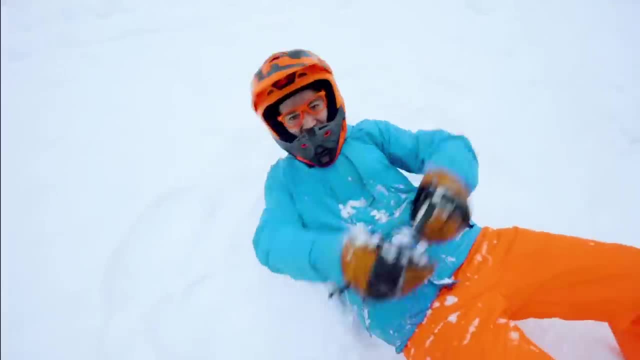 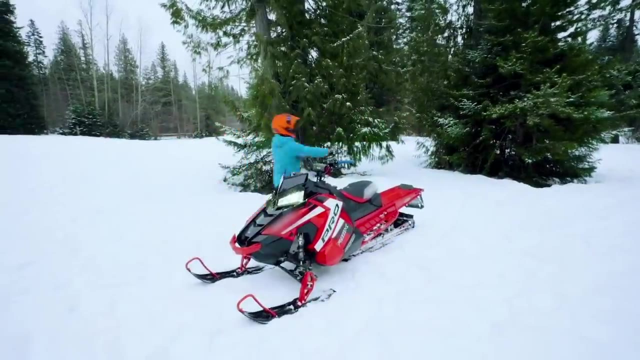 Whoa, Yeah, Yeah, Whoa. Oh my gosh, What a view. Can you see the snow? Oh yeah, Whoa, Hey. can you see the snow? What color is the snow? Gray, Oh yeah. 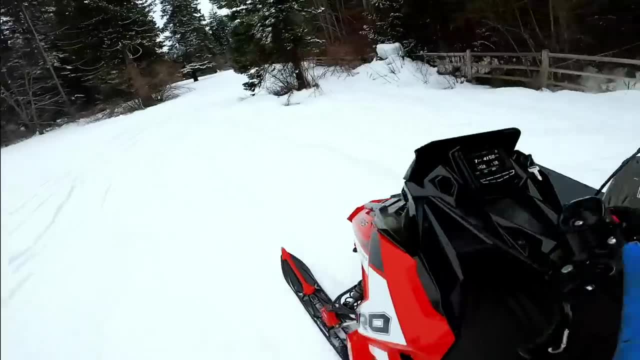 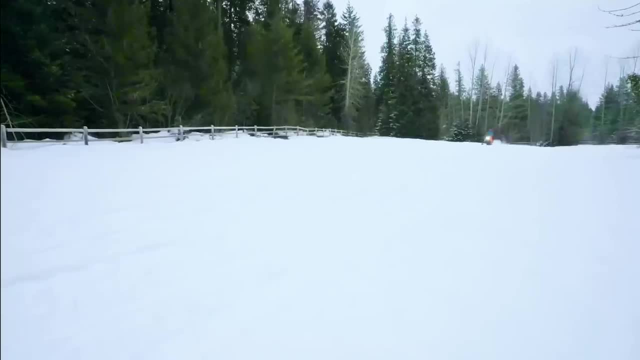 What a view. Hey, can you see the snow? Yeah, Oh yeah. Can you see the snow? Oh, yeah, Yeah, Whoa, Yeah, I hope this is successful. This is the best snow I've ever seen. 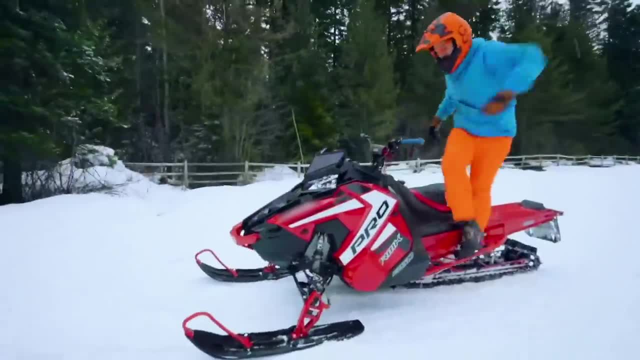 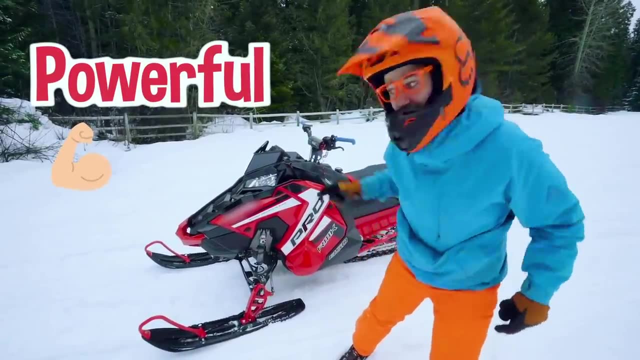 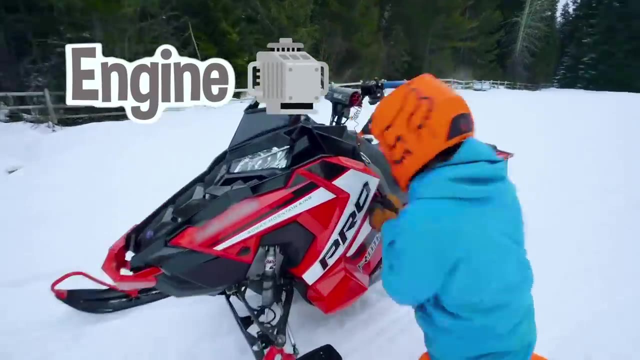 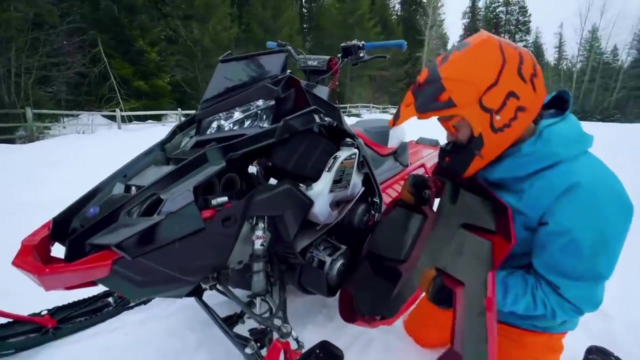 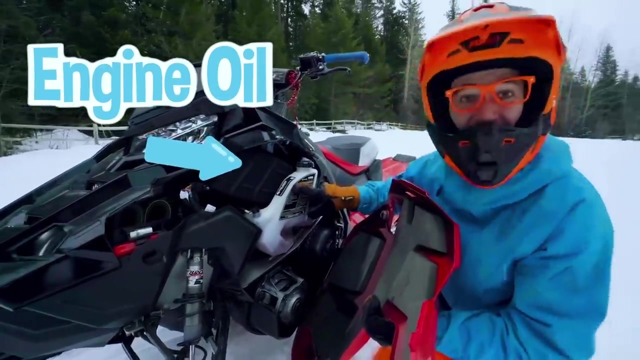 Whoa, Oh, wow, Wow, Oh wow, Wow. this snowmobile is so powerful. do you know how the snowmobile gets all of its power? yeah, the engine. whoa, check that out, looks like we have. oh, this looks like maybe the engine oil. whoa, that's what helps cool the engine. um, let's see. 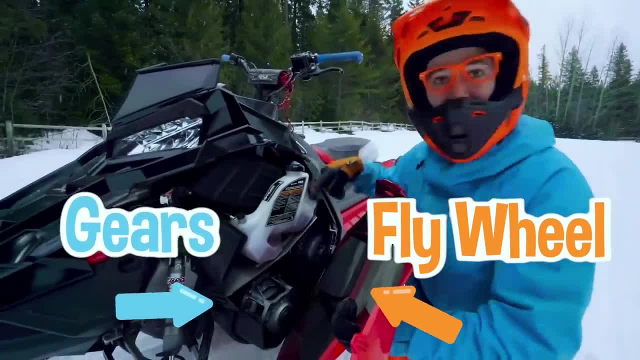 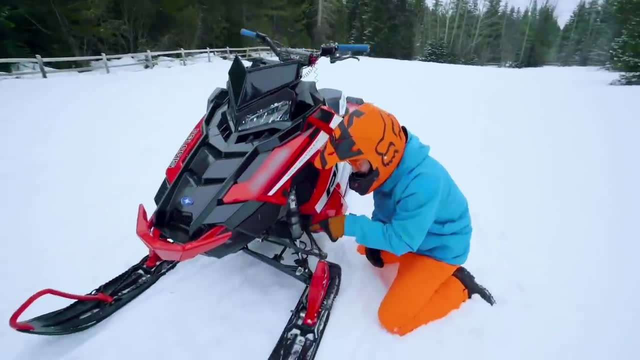 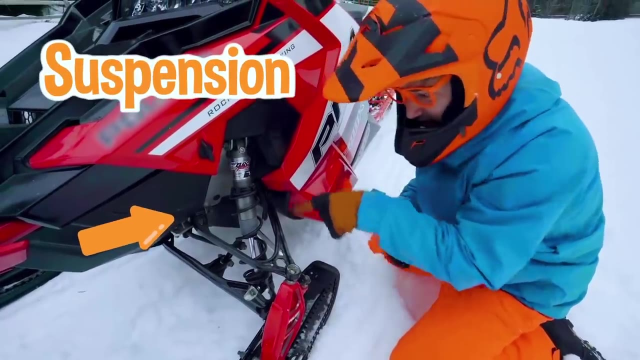 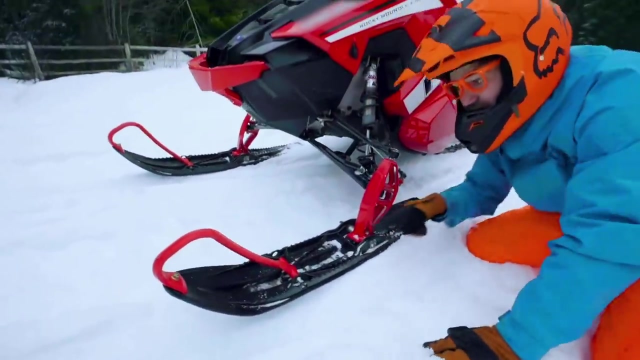 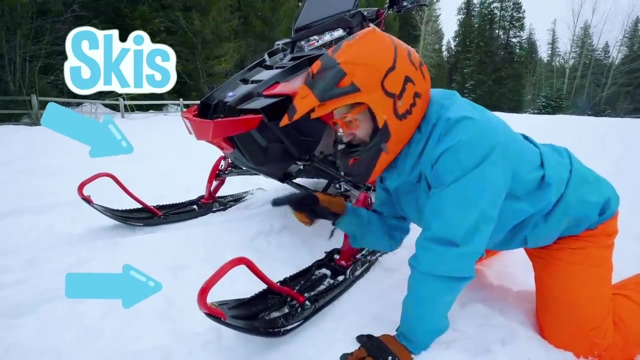 whoo, looks like the flywheel. some gears. oh, and look at this. this is a front shock. yeah, this is part of the suspension of the snowmobile. whoa, and look down here. oh, this snowmobile has two skis, one right here and one over there. whoa, that is what's on the 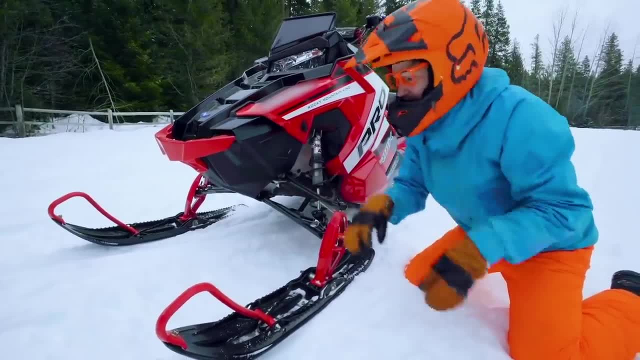 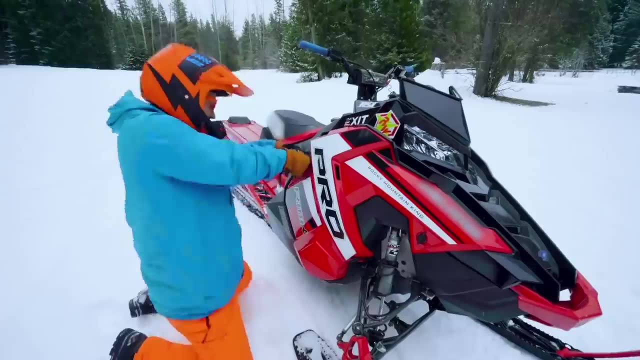 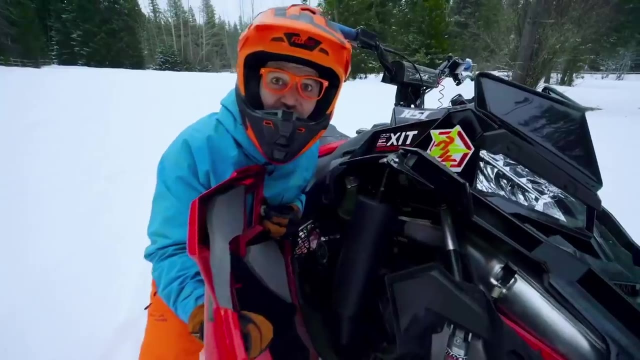 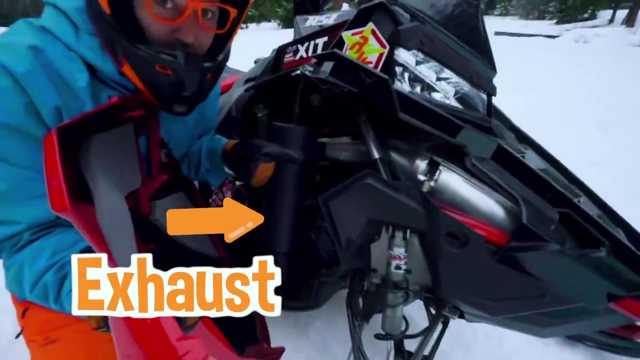 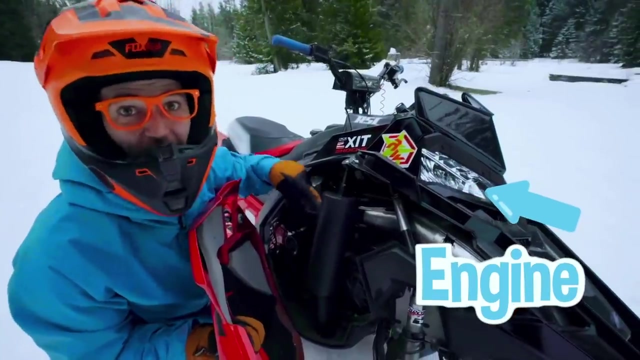 front to help steer the snowmobile. come on to the other side, whoa, the other engine compartment. whoa, looks like we have the exhaust in there. you definitely don't want to touch that. that is really hot. oh, and we have the intake and we have the engine way down in there. whoa, this engine is. 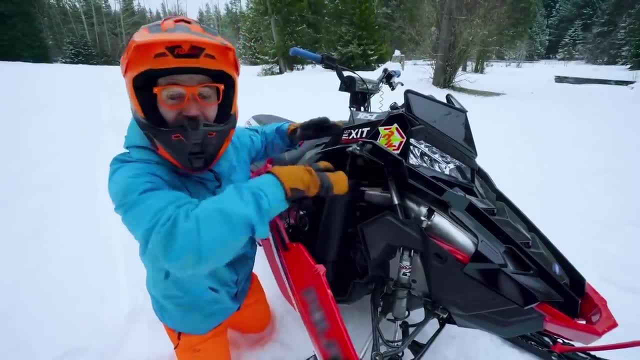 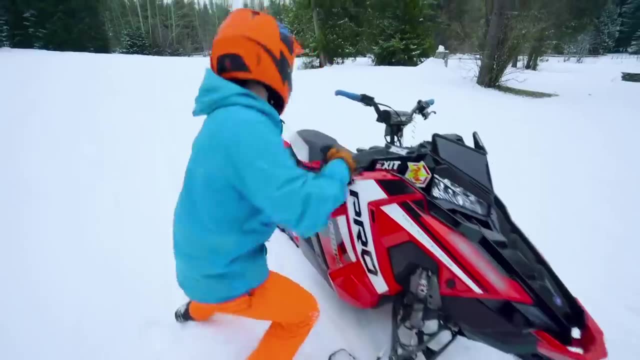 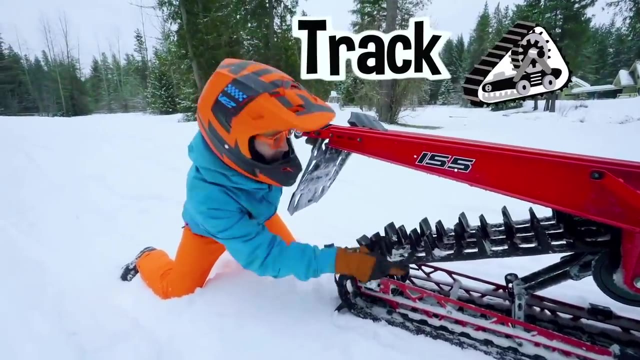 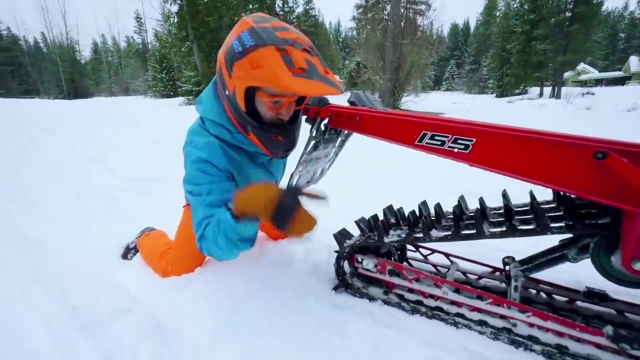 so compact, with so much power. all in the front of the snowmobile. come to the back. check this out. wow, this is the track of the snowmobile. you see these big things poking up. wow, that helps it grip into the snow so it doesn't slip and slide. yeah, that's. 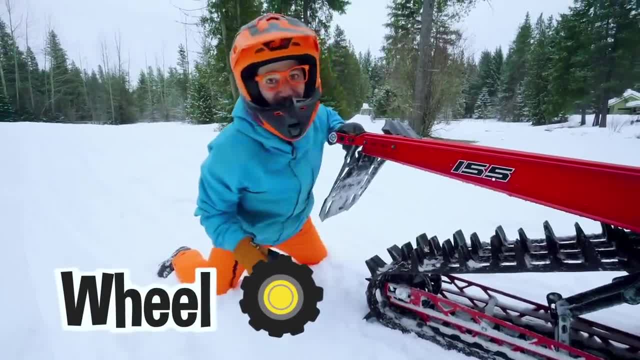 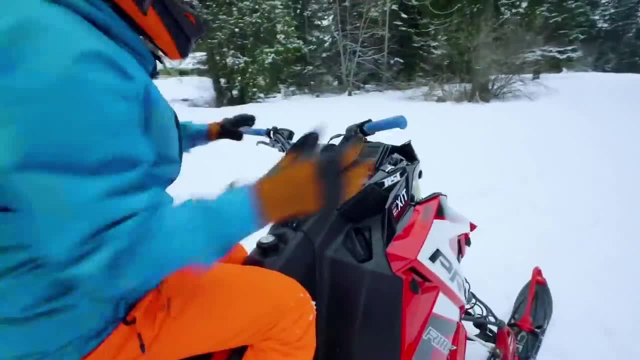 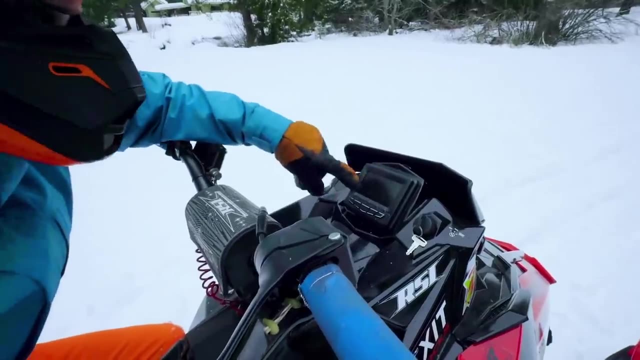 kind of like the tread on a wheel and tire, but this snowmobile does not have a wheel or a tire. oh, come check this out. all right, this is the dash of the snowmobile. This is where it tells you how fast you're going, your engine temperature, Oh, 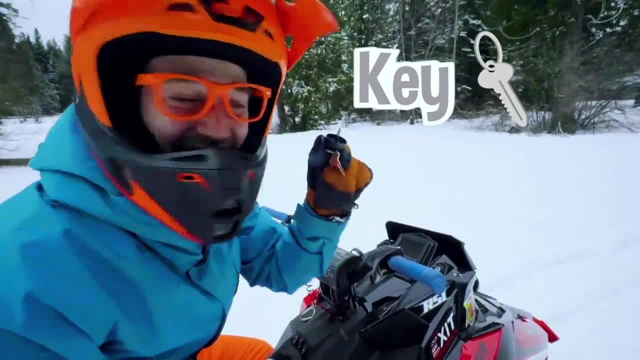 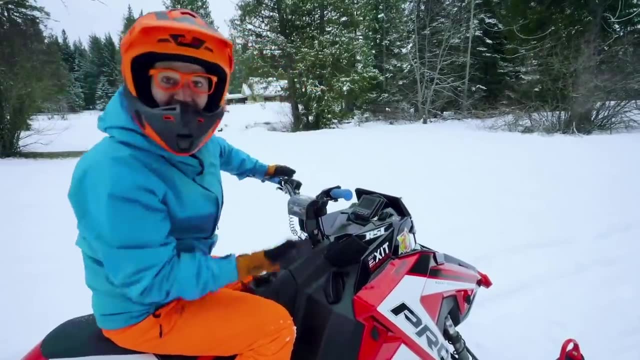 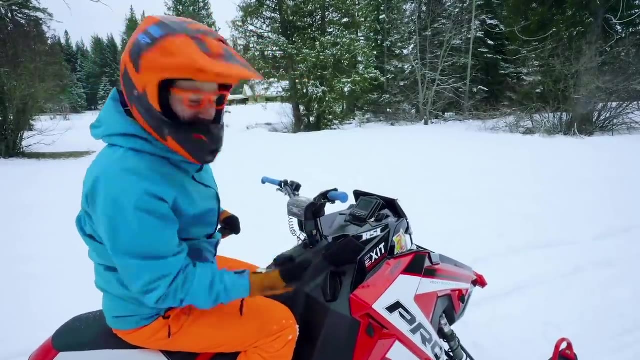 Look it right here. Yeah, the key. Yeah, you know what that does. when you have that in, Then you turn it and that is how you start The snowmobile. but it's not like a car where you just start it with a key. You have to pull. 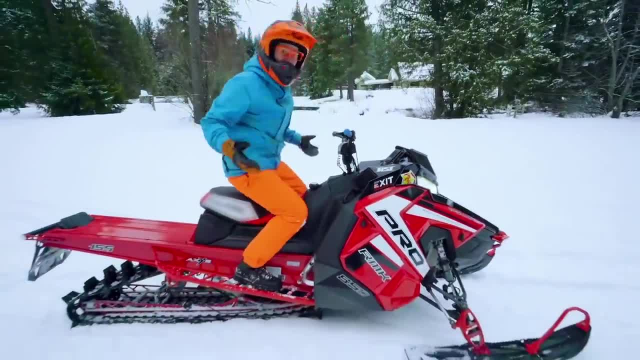 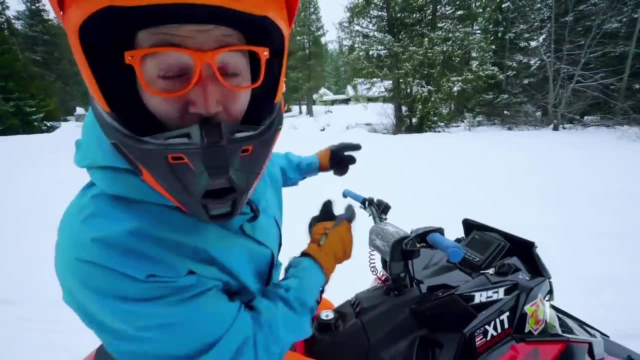 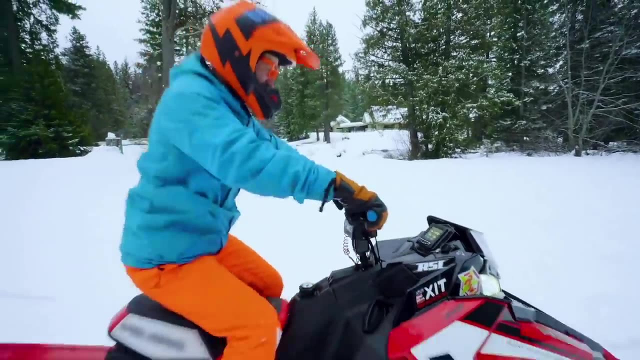 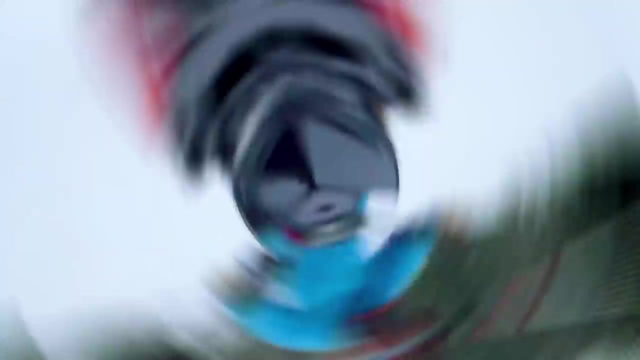 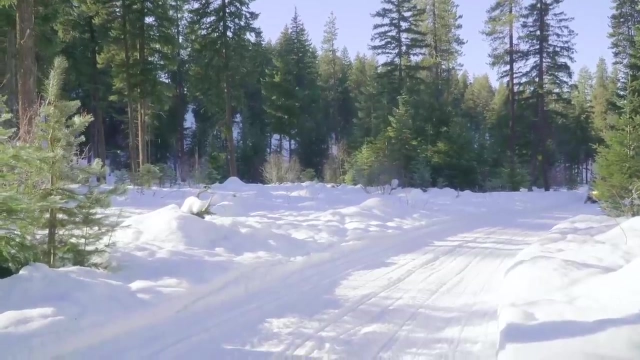 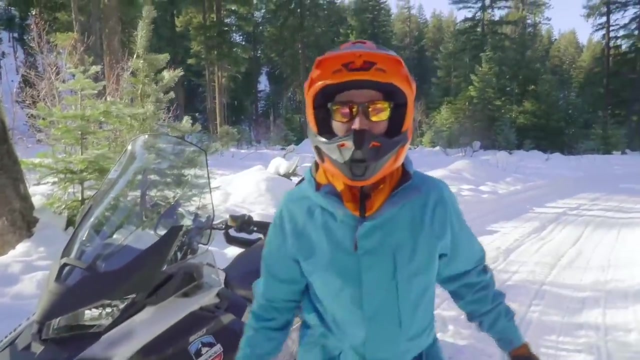 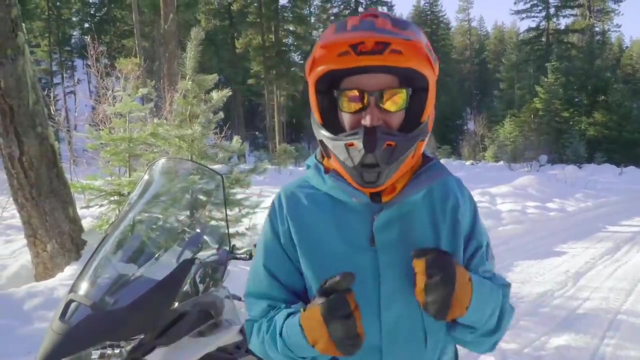 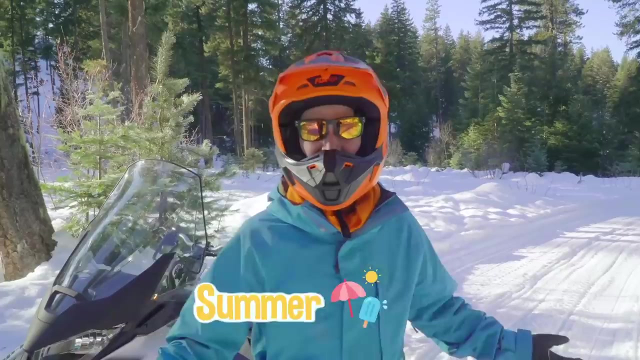 This. check this out. Oh, So for safety we have the brake and not for safety we have the throttle. here we go. Oh, This has been so much fun riding this snowmobile. Oh Geez, I sure do love the seasons, Don't you? It's so cool How you can do fun things during the spring and the summer and the fall, and. 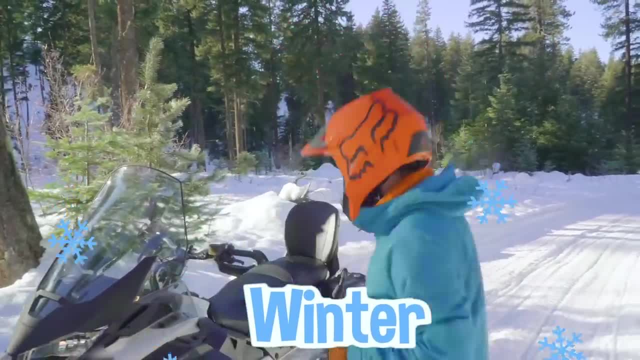 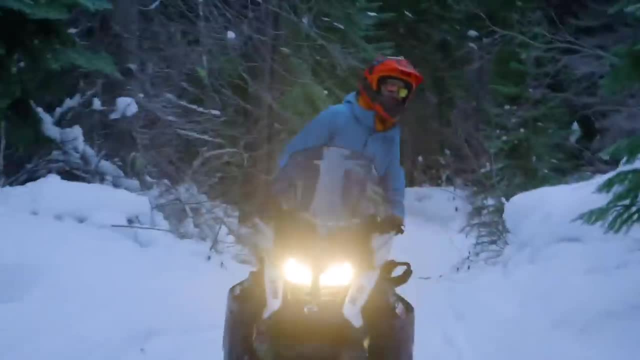 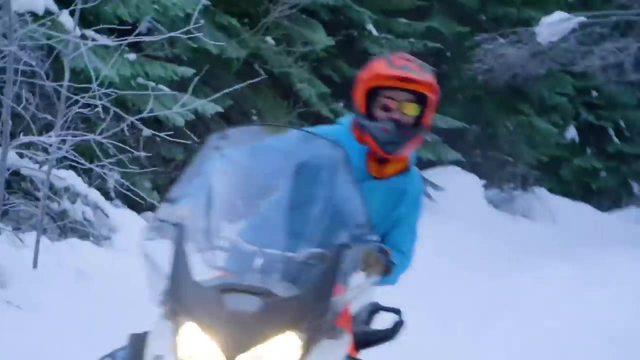 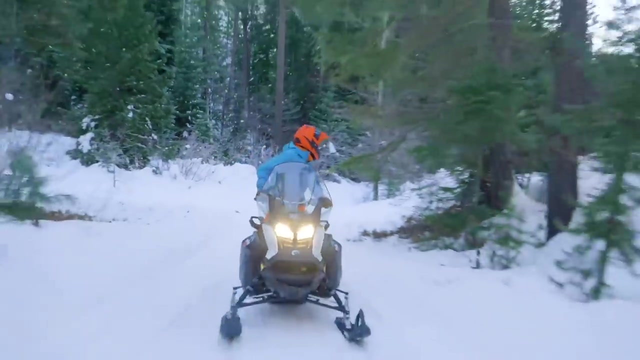 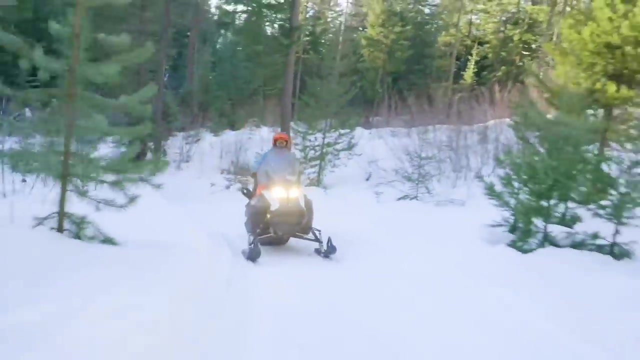 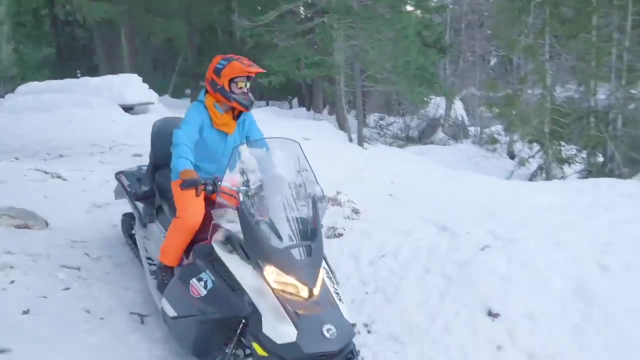 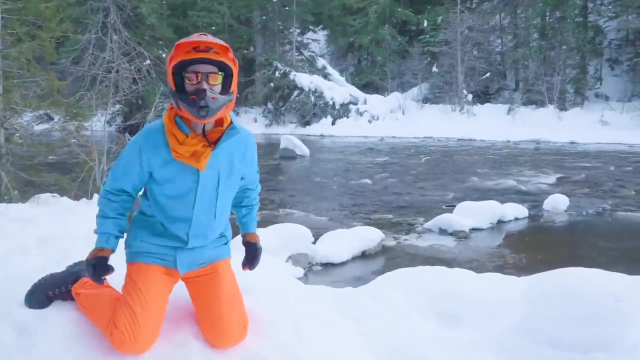 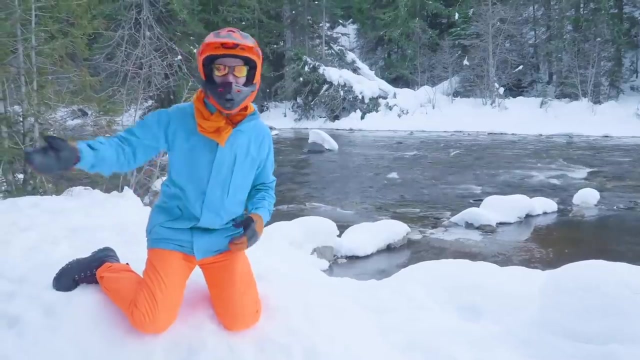 the winter. Yeah, let's go. Oh, Oh, Oh, Oh, Oh, Oh, Oh, Whoa, Check it out. Look at what we found. Yeah, we found a river, Whoa. This has been so much fun exploring with the snowmobiles and finding this river. Hey, do you know what? 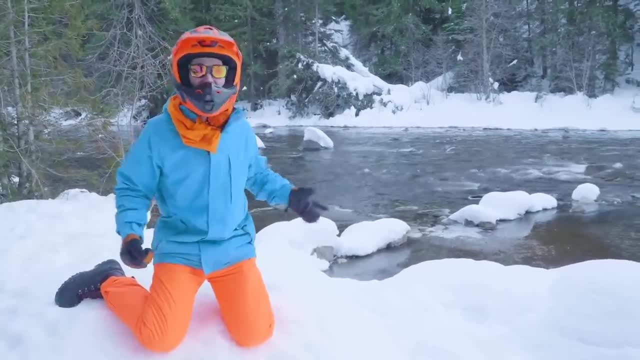 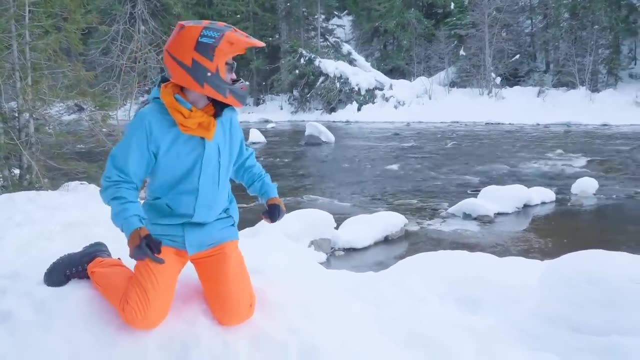 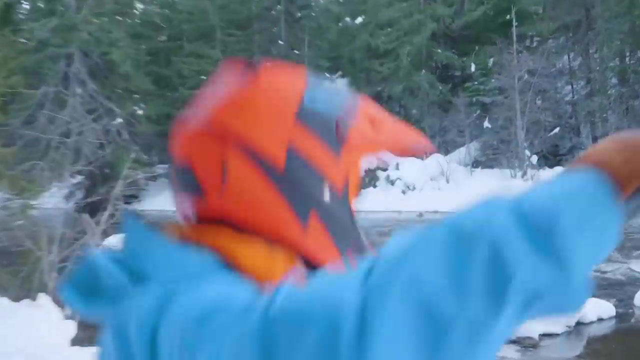 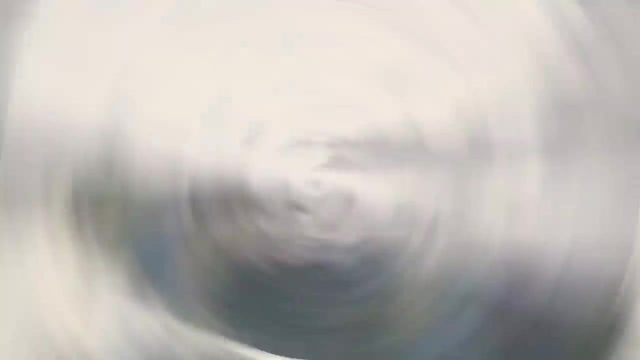 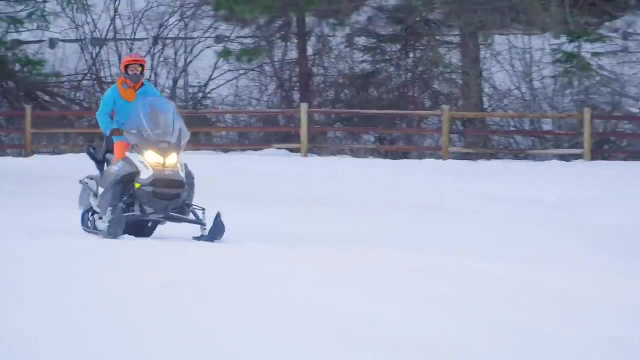 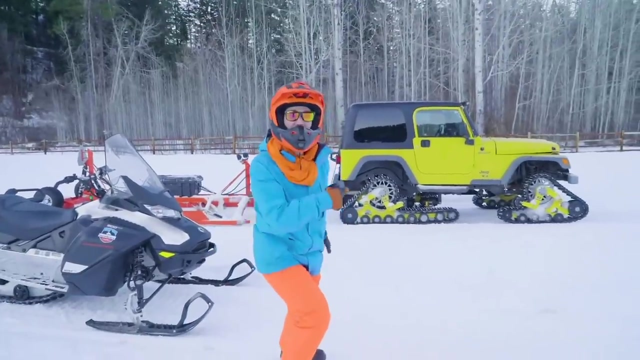 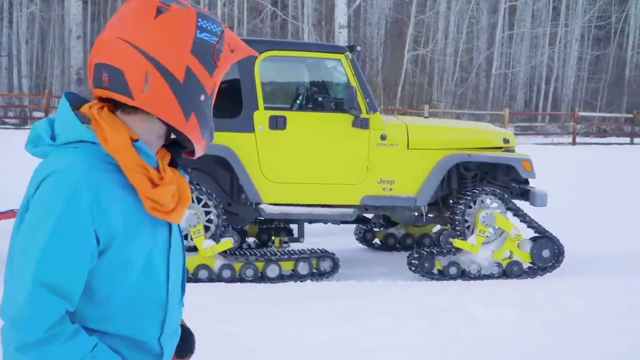 animals live in this river? Yeah, probably some fish. Whoa, I definitely don't want to be a fish right now and swim in that water. That water looks so cold. Whoa, Check out this yellow vehicle. Whoa, Do you see something unique about it? Yeah, check.